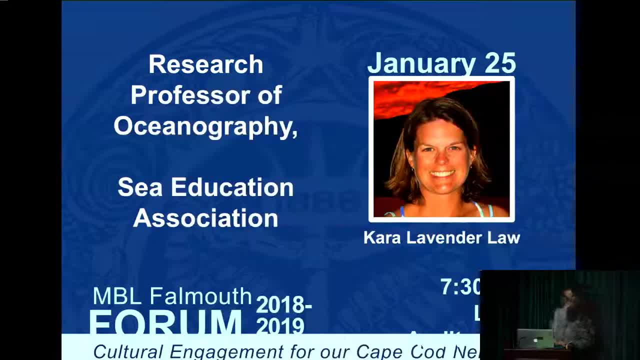 Hi, good evening everyone. So today I'm pleased to welcome Dr Carol Lavender-Law to the MDL Falmouth Forum. So Carol Lavender-Law is a research professor at the Sea Education Association. She holds a PhD in physical oceanography from Scripps Institution of Oceanography and a Bachelor in Mathematics. 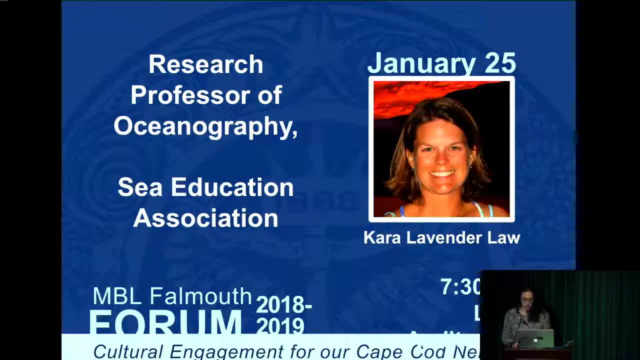 from Duke University. Dr Law's research interests include large-scale and mid-scale ocean circulation and plastic marine pollution, Specifically the distribution of plastic marine debris driven by ocean physics, and the degradation and ultimate fate of plastics in the ocean- the main focus of this talk today. So Dr Law has more than 12 months. 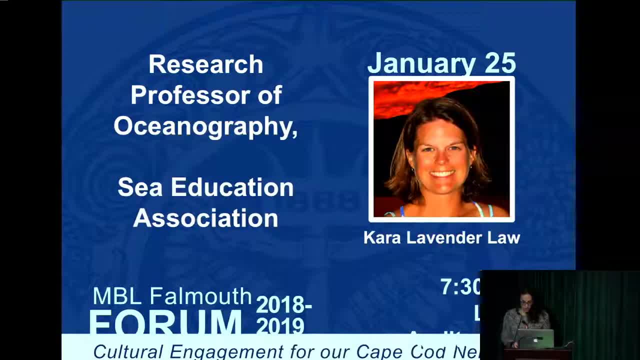 at sea time on research vessels, including in the Eastern North Pacific and Western North Atlantic Oceans, where a lot of plastic debris accumulates. In 2008,, Carol began the analysis of the Ocean Plastics Data Set, collected in thousands of plankton net blows over more than thirty years by. 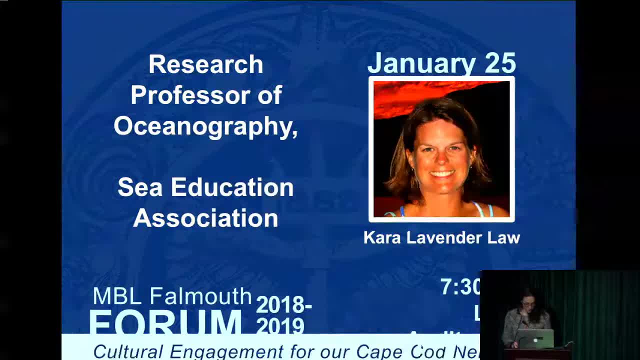 the sea semester students and faculty ongoing long time Syria, which is really, really unique. Cara published in several journals, such as science, in 2010 and 2014. just I'm telling you this to just like to let you know, like how unique is the data that Cara actually has and all. 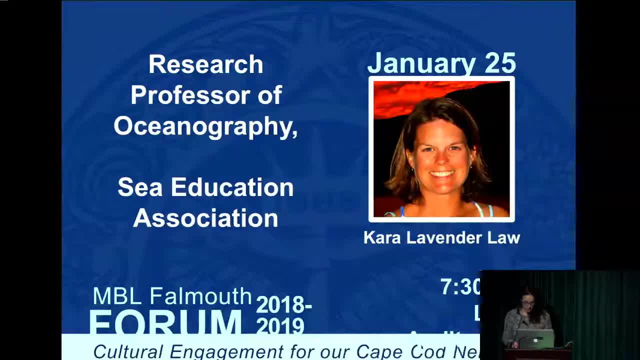 her team, Cara has helped lead efforts both locally and globally to address the problem of ocean plastic pollution, so linking science to solutions on the local level. here in Falmouth, Cara led a team that received a NOAA marine debris program grant to reduce the use of single-use plastic items, and not just 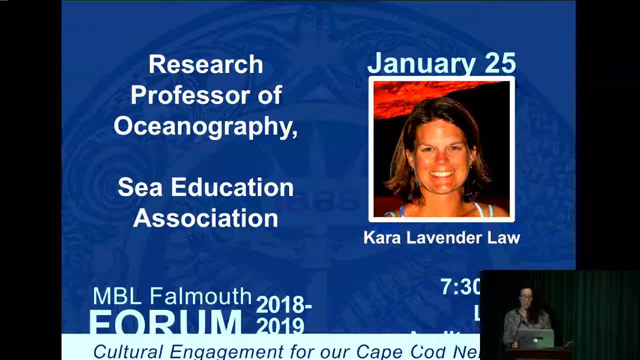 not just that, she also works with her local community in Maine to promote this plastic reduction and is on the board of directors of the Gulf Oceanic Research Center, and is also on the board of directors of the Gulf of Maine Marine Education Association. additionally, last year, in 2018, Cara 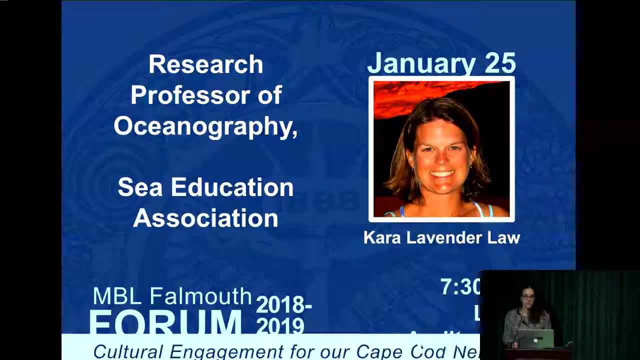 testified about ocean plastics pollution before the us Senate Committee on environmental and public works. on a more international scale scale, Cara participated in a United Nations scientific advisory. she also has served as a science advisor to the tri-sphere scientific advisory. she also has served as a science advisor to the tri-sphere. 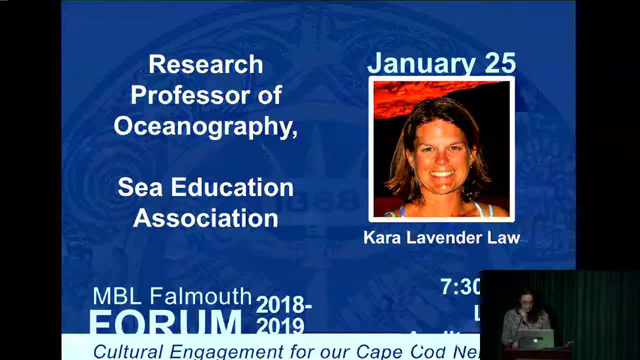 Sea Alliance, led by the ocean conservation conservancy, a group of non-profit leaders working toward an ocean free of trash. so, as you can see, with all that I just explained, Cara has done a lot to raise awareness of the issue of plastic pollution through papers, articles, interviews, talks through. 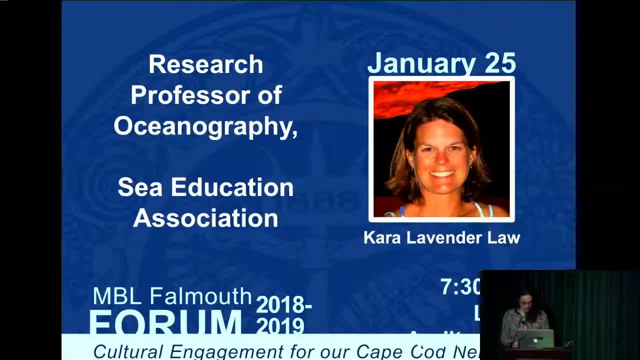 global and local communities and initiatives. but I want to remind you also that, as an active part of the urban agreements framework for hybrid, As an educator she's preparing the next generation of scientists and non-scientists, so everyone to continue working to have a cleaner ocean environment. 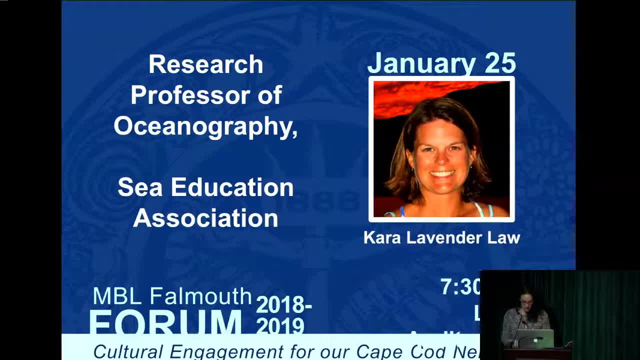 So thank you for that, Cara. Today we will learn how Cara and her team has brought scientific rigor to the popular field. what we know and we've been hearing- ocean plastic pollution. Helping this spell means a conception. So is it real? not in which way? why? from where it comes from? 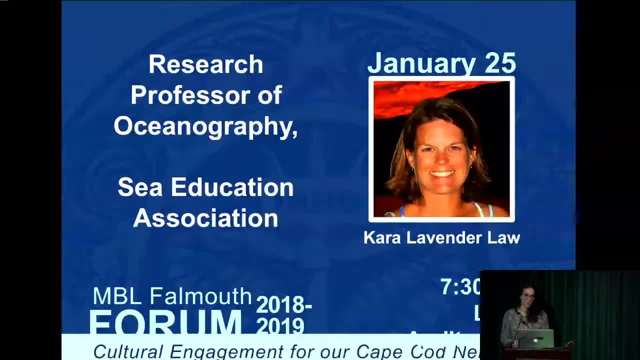 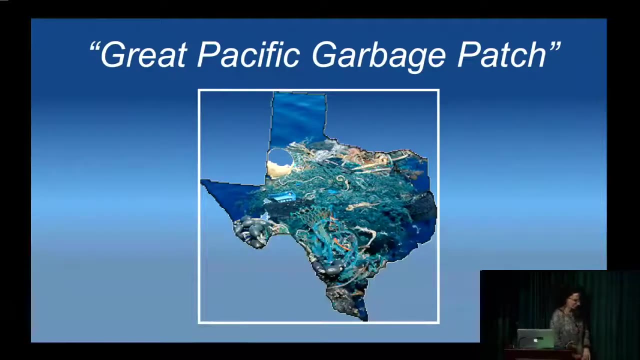 So quantifying the problem and identifying possible pathways to reduce this problem. So just to remind you again, as Anne said, just like silence, your most used plastic-based object, your phone. And please join me in welcoming Cara Lavender. Thank you, That was very generous. 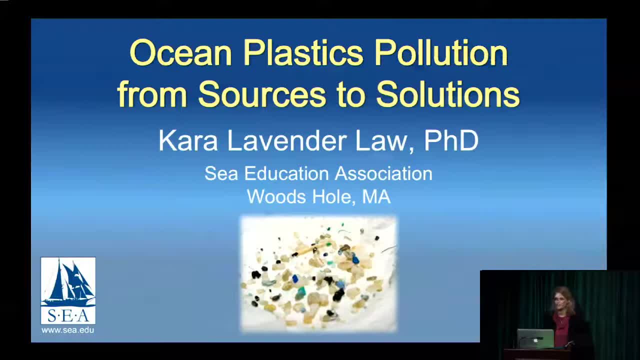 Well, good evening everybody, And first I have to thank Ruth for an extremely generous introduction. I'm not sure where she dug up all of that information And I will try to live up to the billing. I also want to thank Susan Morris for the invitation to come speak with you tonight. 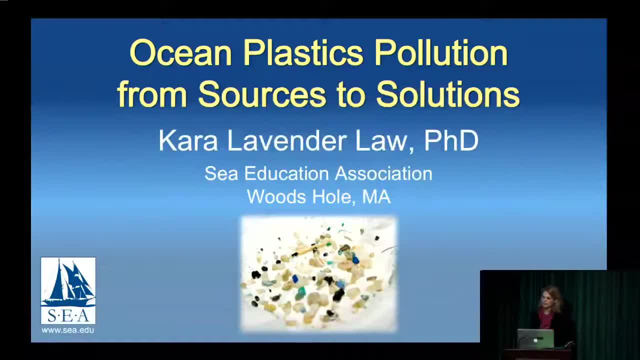 It's a pleasure to be speaking in Falmouth, where I have been working with Sea Education for, oh gosh, what are we coming up? Oh, more than 15 years I'm now based in Maine, but I do come down here fairly regularly. 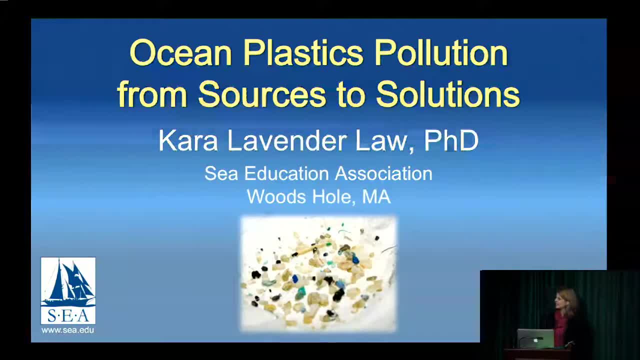 And so it's a pleasure to be speaking to a local crowd, And also thanks to the MBL for hosting and for a lovely meal. So actually let me back up one second. Thanks to all of you for spending your Friday evening here listening to a talk about trash. 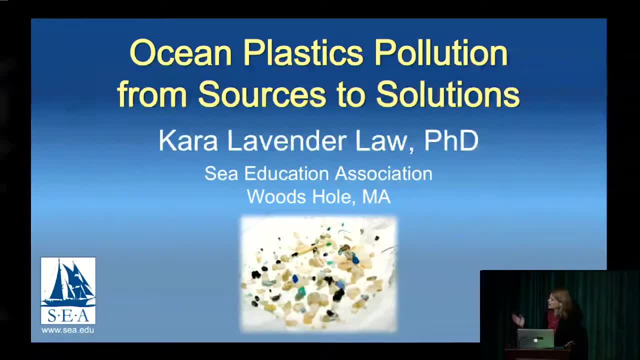 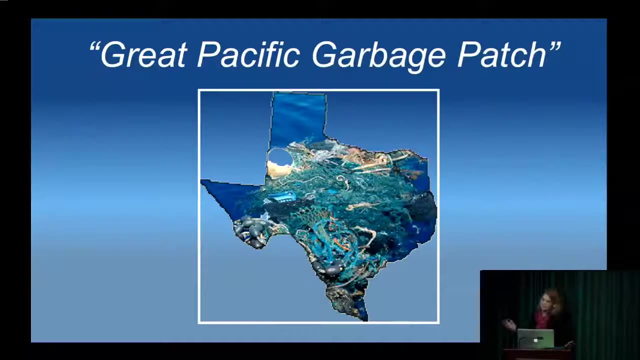 I'm really heartened to see this many people are interested. So I'm going to talk to you today, sort of giving you an overview of my perspective of ocean plastics pollution, From sources to solutions. And I want to start with kind of my entree into this world, which can be summarized by this image of the Great Pacific Garbage Patch. 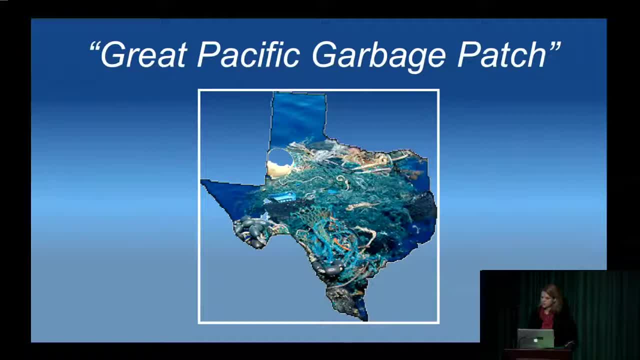 So when I first heard about this problem, it was more than a decade ago And it was from a journalist who emailed somebody at SCA and said: I hear you sail in the North Pacific. Do you sail through this fabled garbage patch? 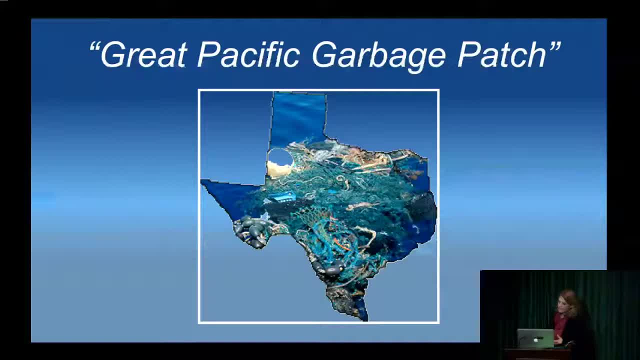 And I had never heard of it. A little bit of digging Found some descriptions about a floating island of trash Twice the size of Texas, So thick you could walk on it, of everyday items- You could see this from space. All kinds of descriptions of something that, if it were true, would almost be a tractable problem, in the sense that you could identify it, find its edges and potentially try to clean it up. 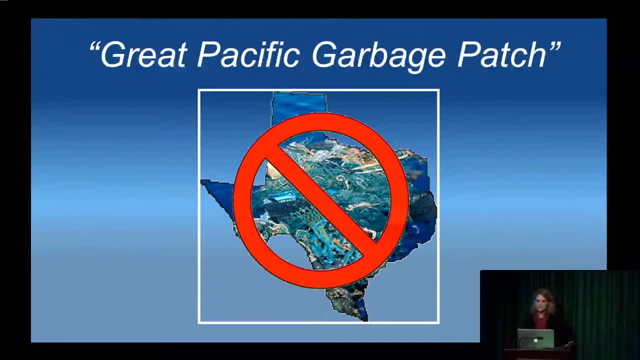 In fact, these are misconceptions, And at Sea Education Association, just up the road here, students and faculty scientists have been collecting data for decades And we knew in-house that this was not an accurate Description of the problem. So we realized that the time had come for the rest of the world to know about what our little educational nonprofit was doing. 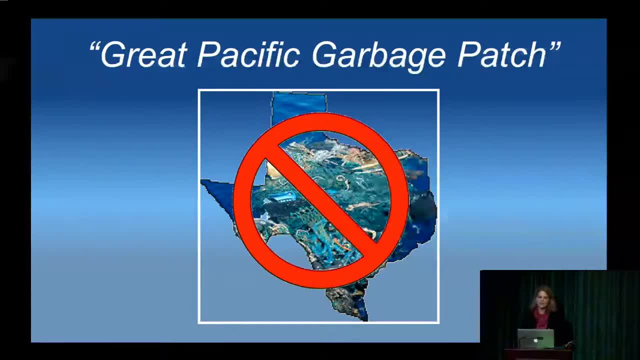 And I was fortunate to be in the right time in the right place to analyze the data set that Ruth so nicely described. So I'm going to tell you that story in a little bit more detail, But first I want to talk about the conception. 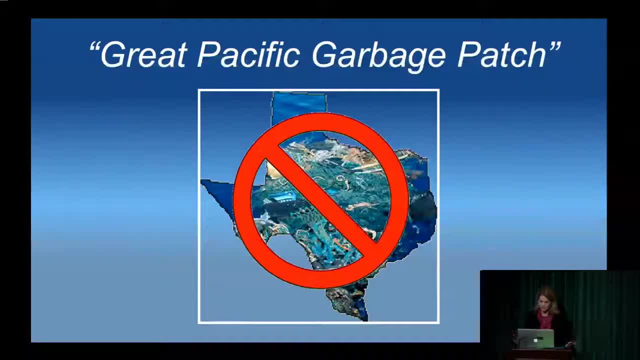 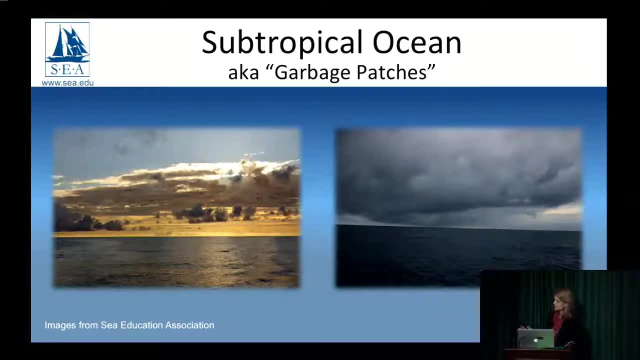 So if you had an idea about a floating island of trash, we're going to put that aside And, from my experience sailing out in the open ocean and the places That you would refer to as garbage patches, these are more typical images of what you would find if you were standing on the deck of a ship. 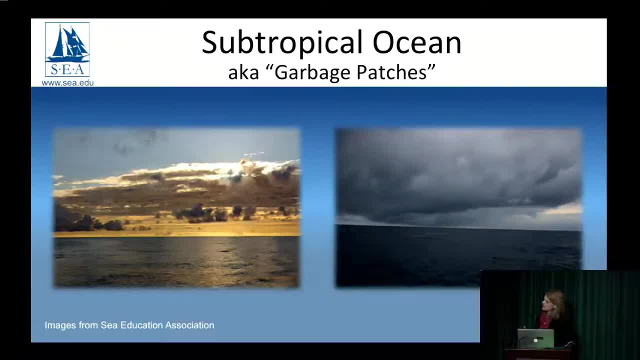 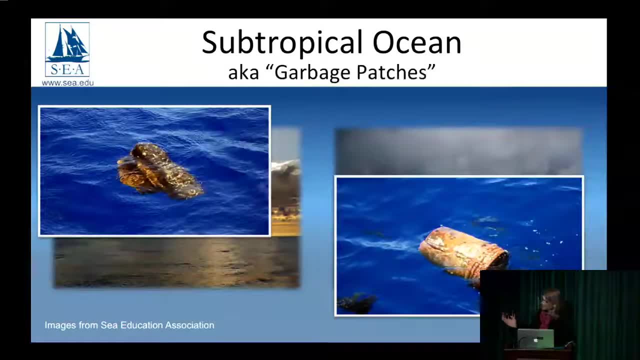 So you look over the side. often there's very light winds, you see water and clouds, and occasionally something might float by. that's very surprising. So in this case we have a boot, we have a five-gallon bucket that's all encrusted with some kind of organic matter. 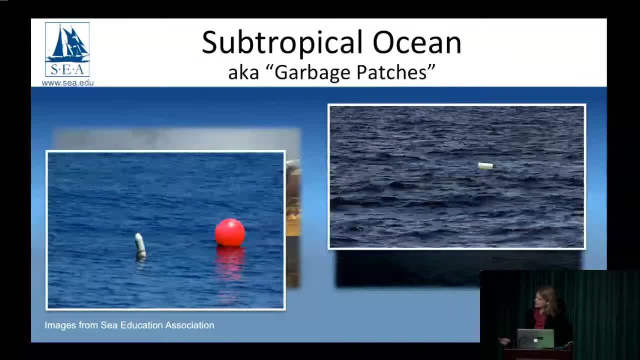 More often than not, you would see something that is clearly an item, a man-made item. You maybe don't know exactly what it is. we think these are probably fishing buoys of some kind. this is some kind of container. You might see a large fragment that's pretty clearly made of plastic. 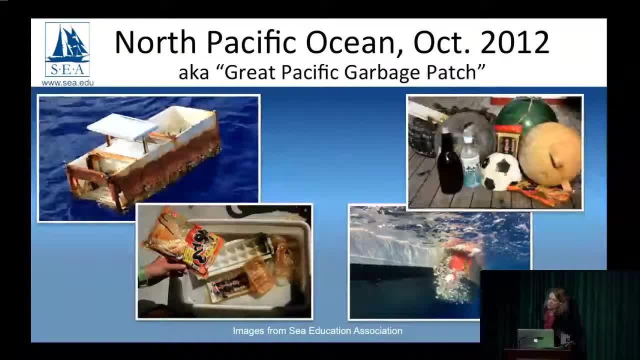 And in extremely rare cases you might see very recognizable items that you can trace to an actual source. So these are pictures that were taken on our ship that sails in the Pacific Ocean about 18 months after the Japanese tsunami, So this was in October 2012, on the opposite side of the Pacific Ocean. 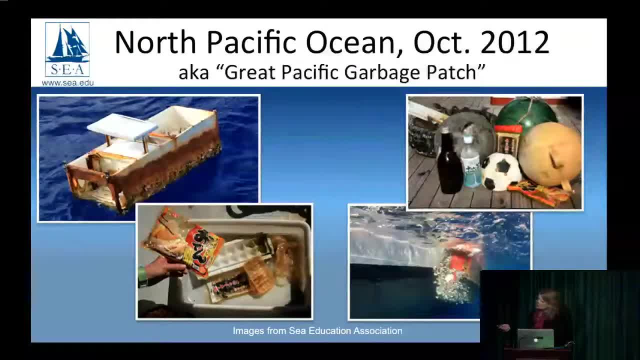 And we saw things. the crew on the ship. The crew on the ship saw this floating refrigerator going by. We of course couldn't recover it, but inside this drawer you could see these food packaging items and an egg tray. So really shocking on many levels. 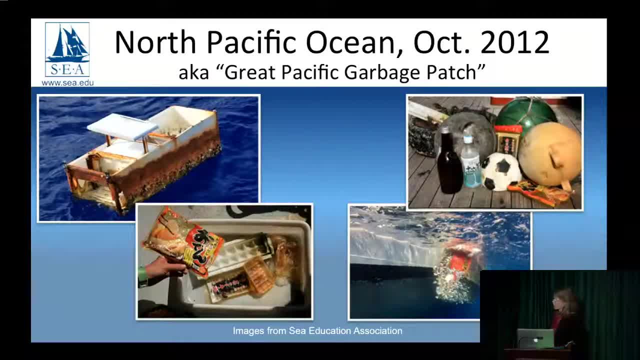 This was somebody's appliance and their food that got washed into the ocean that drifted across. We found also other clearly recognizable items. There's a tire back here. there's some fishing buoys, the food packaging. there's bottles with clearly Asian characters, a soccer ball. 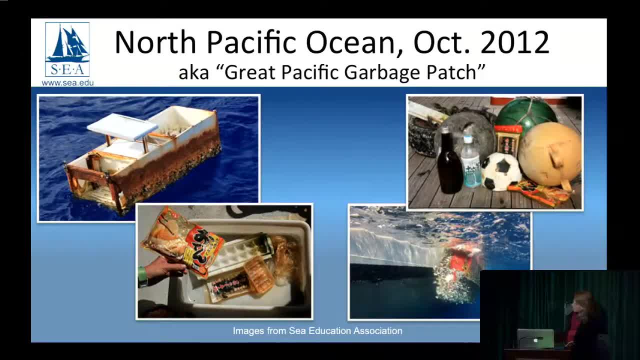 There was also a bottle. There's also this dinghy that was drifting- had been weighted down by the barnacles growing on it. This is pressed right up against the side of our vessel. So in this instance we can't say with 100% certainty, but it's pretty clear that these were items that washed out to sea and traveled across after the tsunami. 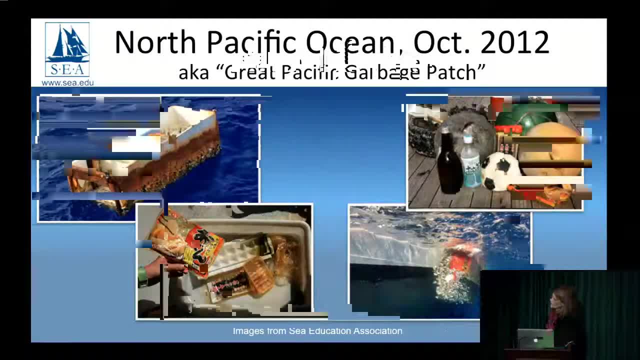 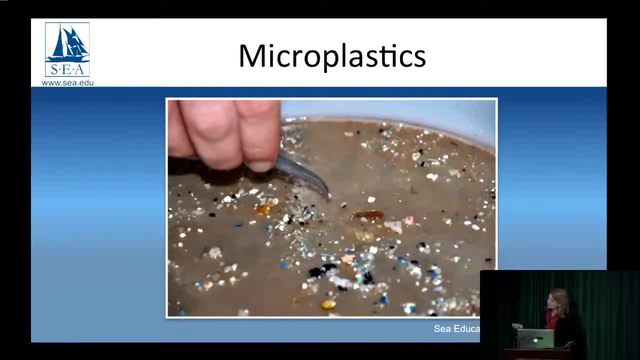 So instead- you know that's a very rare instance, I don't think we've had another occasion like that, But in these regions the subtropical ocean gyres. what you typically see are these microplastics. So this is a sieve and a student with some tweezers. 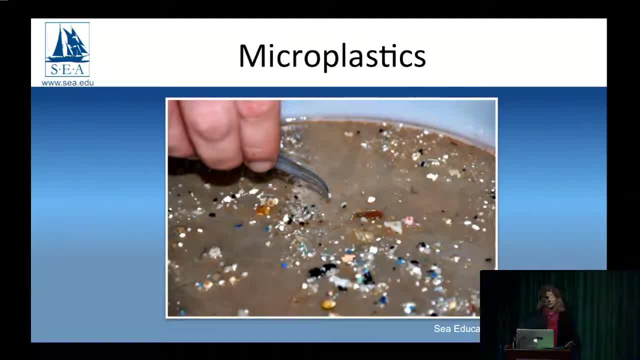 And you just see these brightly colored fragments that are irregularly shaped And there's different sizes and different colors. This is not a big item. It's not a water bottle, But it's still plastic and it's still a contaminant. So we hear a lot about microplastics. 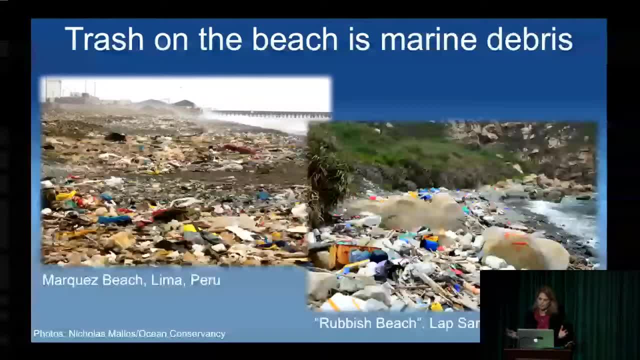 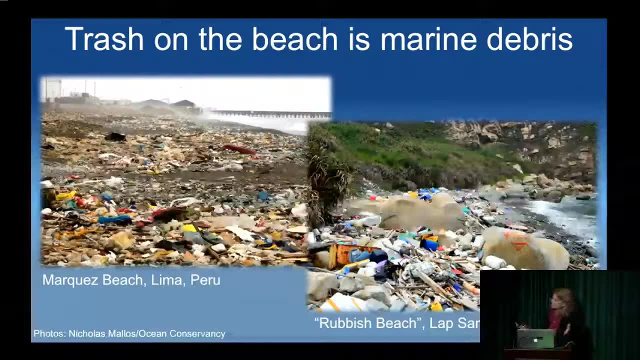 But in fact the category of materials we're talking about are broadly referred to as marine debris, So manmade items in the marine environment, And I just want to take a minute to acknowledge other aspects of the marine debris problem. So trash on the beach is also marine debris. 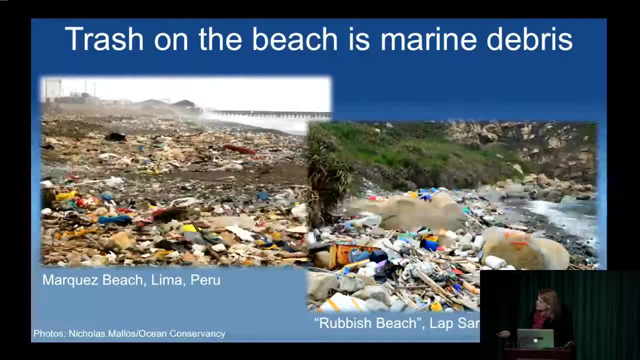 These are images taken by a colleague at Ocean Conservancy. This is a beach in Lima, Peru, that pretty clearly serves as an open dumping site. If you look at the sort of materials here, it looks like everyday items, And in Hong Kong this largely looks like a lot of sort of fishing debris or maybe debris that has washed ashore. 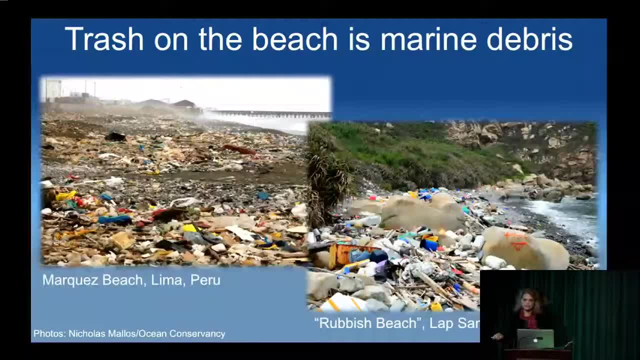 So, even though maybe here in Falmouth we typically don't see things that look like this, we have all gone to the beach and found different types of items, Trash type items. Well, the International Coastal Cleanup has been going on for more than 30 years now, carried out by Ocean Conservancy. 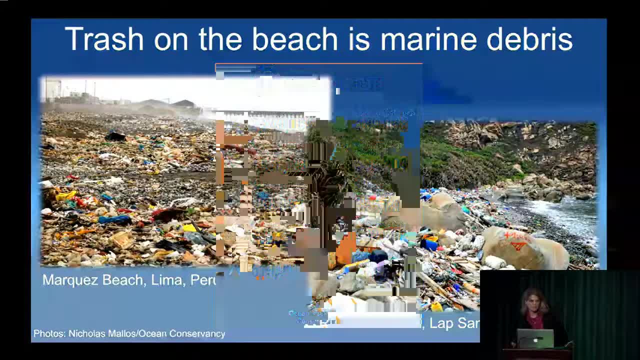 And they've done a great job logging the types of items that are collected And the number- the top ten list of items collected- has not actually changed substantially over that 30-year period, And the things that are picked up are things that we all recognize. 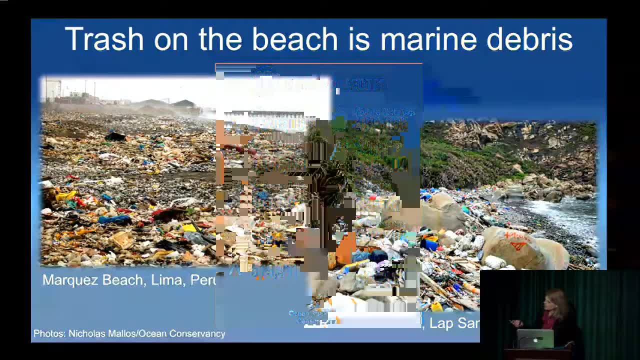 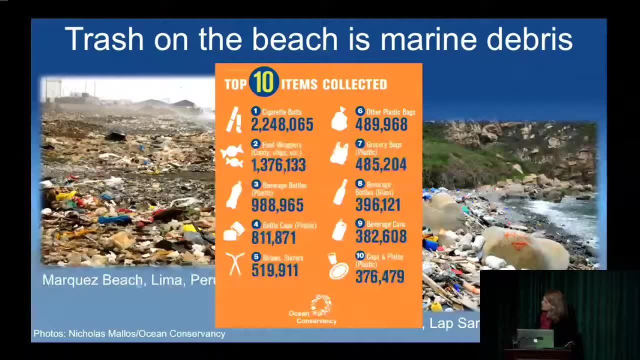 That we all use every day- although I hope we don't all use this every day- But cigarette butts, food wrappers, beverage bottles that are plastic, glass grocery bags, Cups and plates. In 2018, I believe it was the first time that the top ten items on the list were all made of plastic. 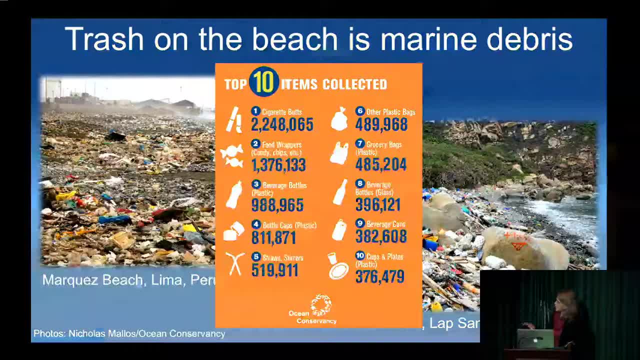 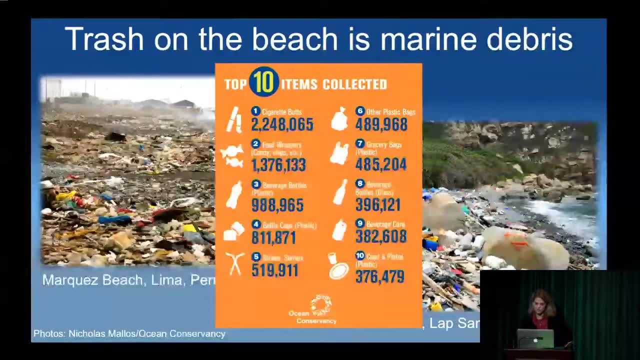 So glass bottles had dropped off And other types of bags had dropped off. So marine debris is made up of items that we all use every day. You're probably not surprised also to know that marine debris is also found on the sea floor. 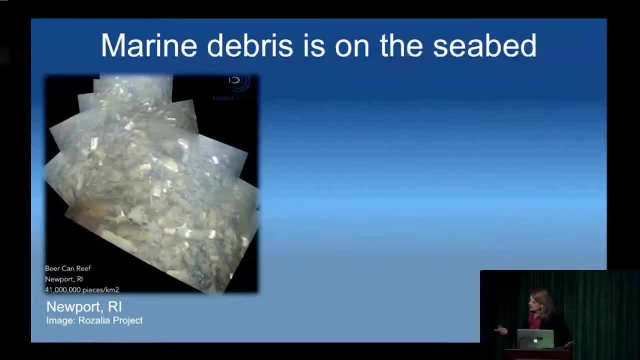 So this is a collection of images taken by the Rosalia Project with a remote camera, With a remotely operated vehicle in Newport Harbor in Rhode Island, And so it's probably hard to see, But there are plastic water bottles and cups and cans and beverage items. 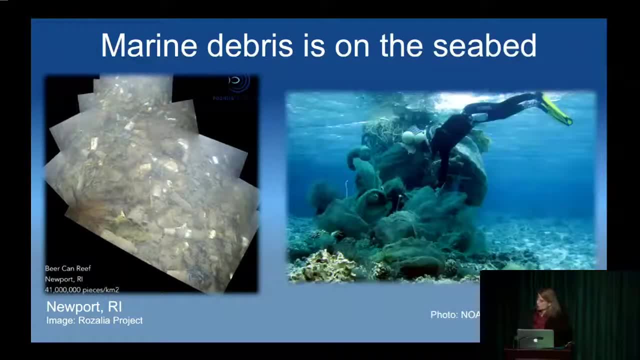 Again trash that is ending up sitting on the sea floor. But there are also things like large derelict fishing nets. This was a photo from Midway Atoll in the North Pacific. This was actually a debris removal effort, So the marine debris on the seabed also takes lots of different forms. 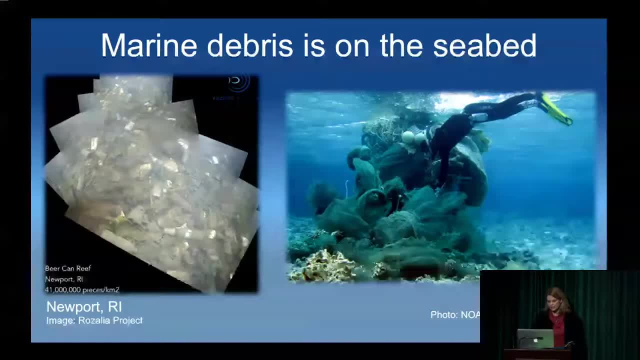 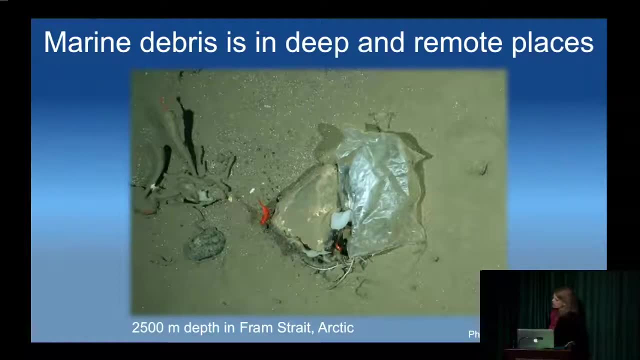 It can be consumer items. It can be large derelict fishing gear And other strange items too, I'm sure, But you may be surprised to learn that marine debris is also found in very deep and very remote places. So this is an image of a plastic bag that just looks pristine. 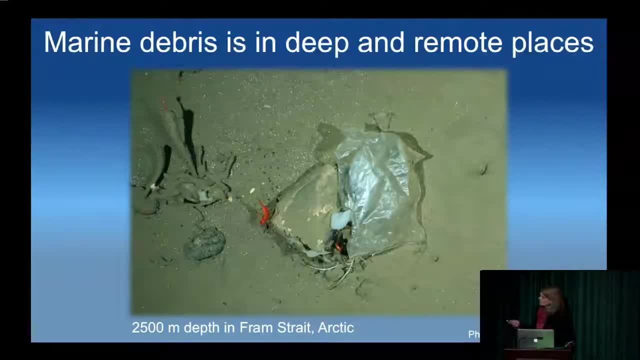 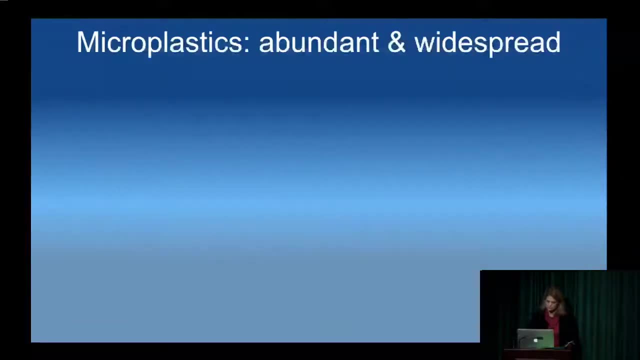 From 2,500 meters depth in Fram Strait in the Arctic, So even in very remote places far from human populations, we're finding identifiable trash items. So we hear a lot about microplastics. and why is that Well? 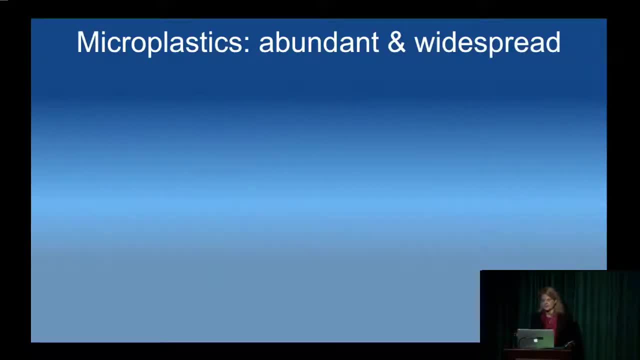 First and foremost, microplastics- by count, are the most abundant type of debris in the marine environment, So, counting individual particles, And they're also the most widespread. So microplastics, these tiny bits, can be found on beaches. 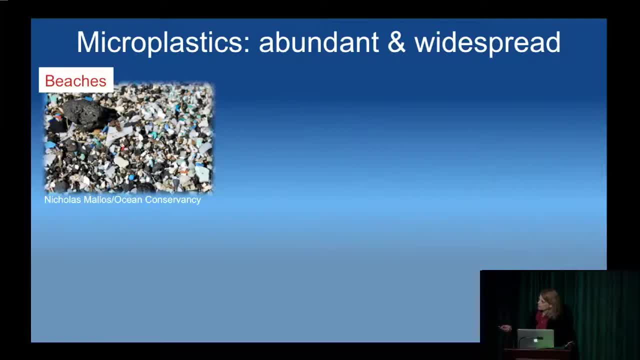 This is a photo from the big island of Hawaii, Camilla Beach, which is well known for being trash collecting beach. These microplastics are found in the water column in the ocean, So this is a picture of plastics collected on one of our ships in the North Atlantic. 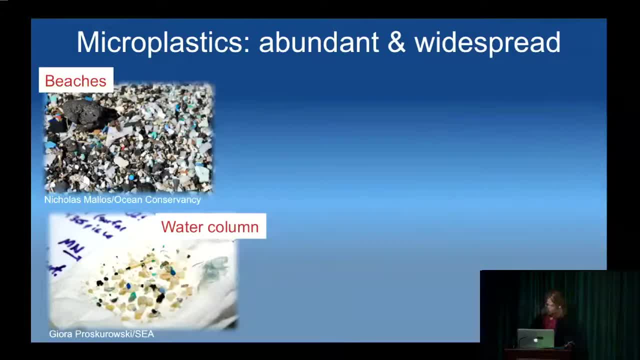 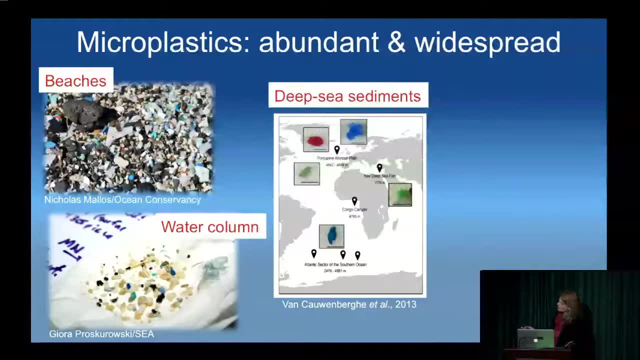 But they are also below the sea surface too. What we collect is at the sea surface. Microplastic fragments have also been found in deep sea sediments. So these little pinpoints are showing you where these were collected. So broadly around the North and South Atlantic and also the Mediterranean Sea, these fragments have been found. 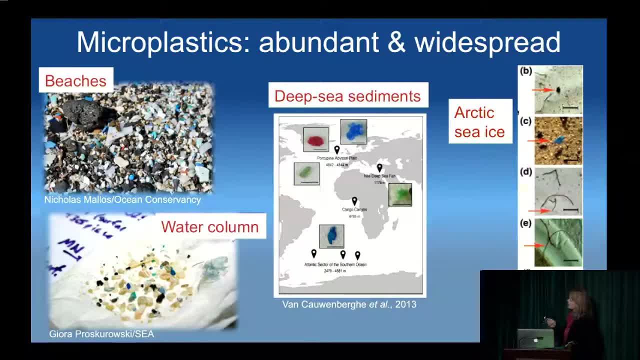 And then most recently there have also been microplastics found in Arctic sea ice, And here we start to see this form that people refer to as microfibers. So this is kind of the newest category of microplastics, The newest category of microplastics that's starting to get a lot of attention. 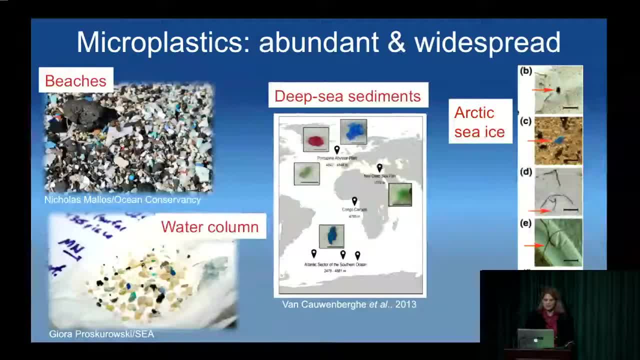 So even frozen into Arctic sea ice. So microplastics, especially microfibers, seem to be quite ubiquitous in the marine environment, And so for that reason alone, I think people are really starting to focus on research into microplastics. 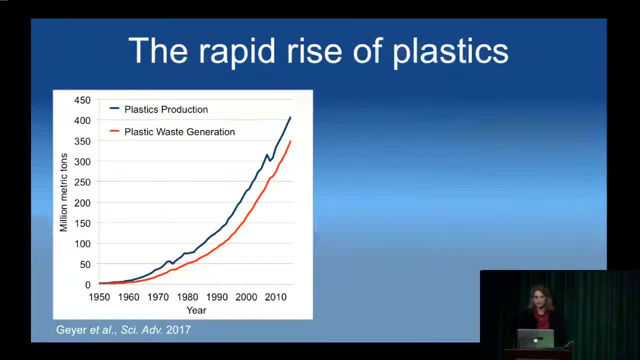 Well, how is it that plastics, plastic, debris, microplastics have become so widespread in the environment? And microplastics, by the way, are not limited to the marine environment. There is also increasing work showing that microplastics are not limited to the marine environment. 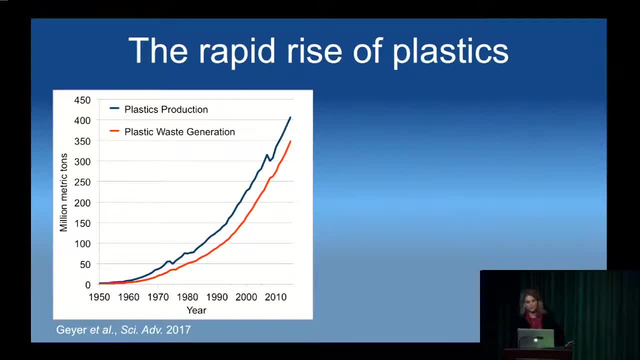 There is also increasing work showing that microplastics are not limited to the marine environment. So microplastics are found in rivers, in lakes, even high alpine lakes. They are in agricultural soils, They are in our drinking water, tap water, bottled water. 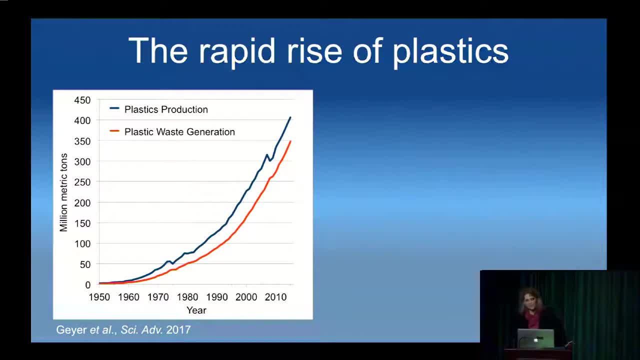 They are in beer, They are in sea salt. It seems that wherever we look, we can find little bits of plastic. So why is that? So this figure is showing you the two curves. The blue line is global plastics production in units of million metric tons, as a function of time. 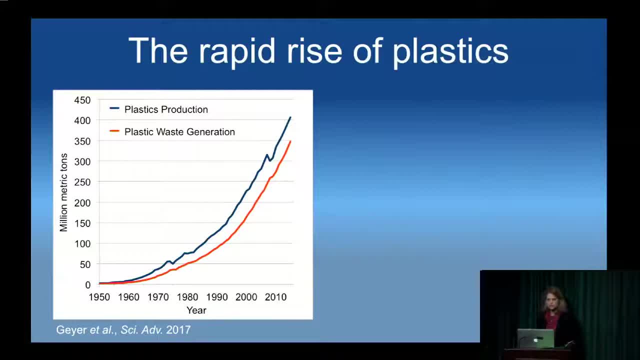 So 1950 is sort of the canonical start of global plastics production. so 1950 is sort of the canonical start of global plastics production in units of million metric tons as a function of time, From industrial production consumer plastics, You can see, over time this curve is pretty much exponentially increasing. 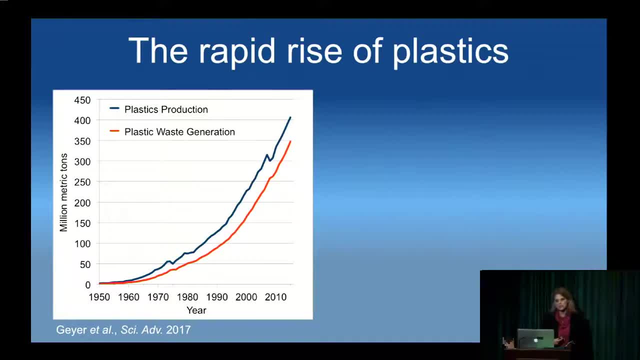 There is a little dip here. because of a global recession. The increase in global plastics production has actually outpaced most other commodities- materials including steel and cement. So the growth in plastics is notable, From our estimation, since the beginning of this commercial production. 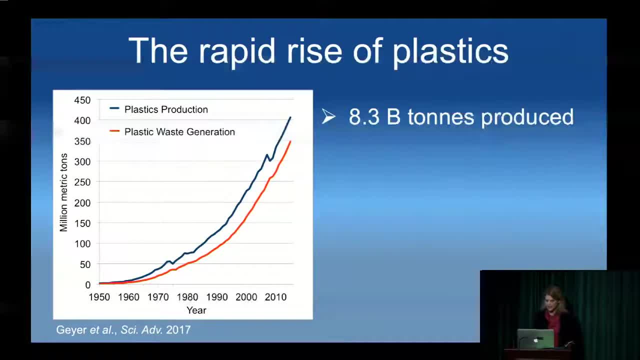 8.3 billion metric tons of plastics. That number is so big that it doesn't matter if I describe it to you in terms of Empire State Buildings or Blue Whales or football stadiums: it's huge. It's a huge amount of material. 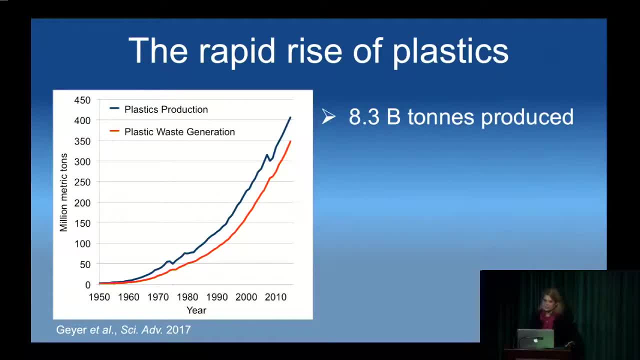 So what happens to that material? The red line is showing you plastic waste generation globally. So in this study we tracked plastics production and we tried to follow sort of the uses through sectors like packaging or transportation or industrial purposes And we asked what's happened as that plastic waste has been generated. 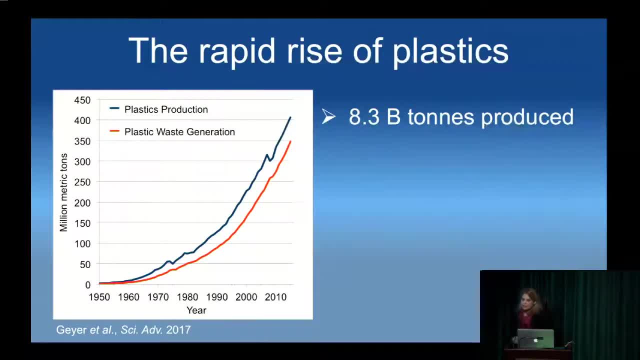 How has it been handled? And what we found is that the vast majority has either been landfilled or is sitting in the environment. Less than 10% has been recycled and about 11% has been incinerated. So when you look collectively at all of this 8.3 billion tons that we've produced between 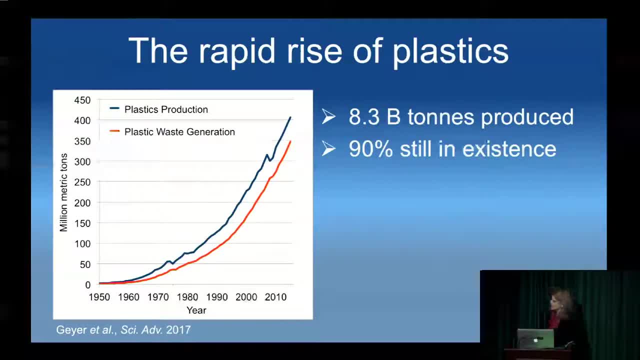 what's still in use and what's in landfills or in the environment. we estimate that about 90% of plastic waste has been generated. 90% of that material is still in existence on the planet, So this is a tremendous amount of material. but even back when we were only producing 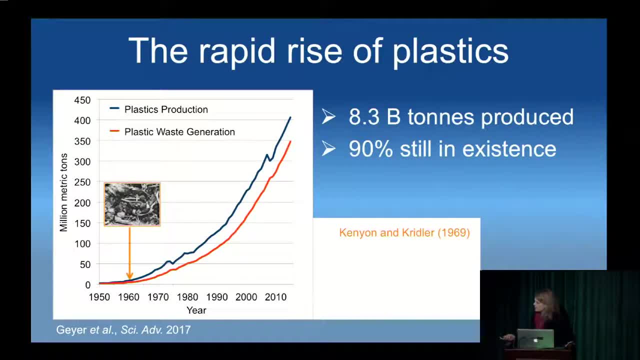 maybe 10 or 15 million metric tons. back in early 1960, there was evidence of this material ending up in the environment and contaminating wildlife. So there was a paper published in 1969 that documented: this is a seabird, if you can't. 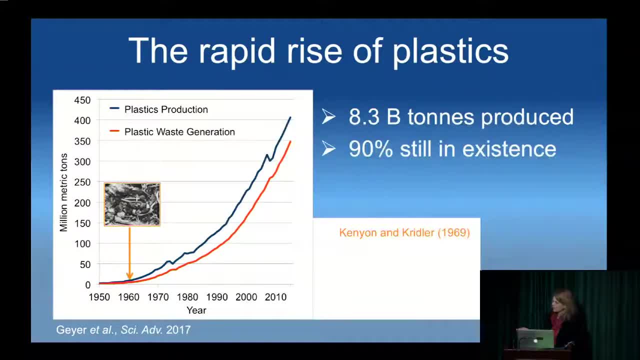 tell The seabird is. it's a seabird carcass that has plastic debris in its gut And it was first described in 1960.. The first description of floating plastics in the open ocean was published by Hooey scientists in the 1970s from the North Atlantic. 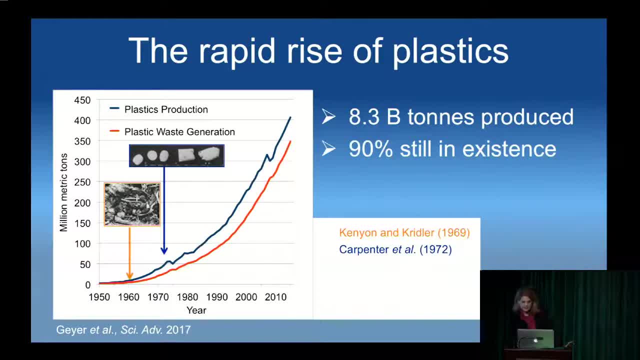 These are little industrial resin pellets and then microplastic fragments And then SCA. first started getting into the microplastics business in a formal way in the mid-1980s thanks to a scientist named Jude Wilbur, who's still a Falmouth resident. 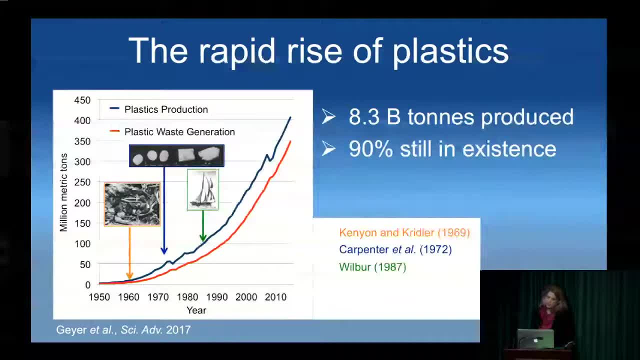 And he published a paper in Oceanus Magazine documenting some of our early data collection. But really it wasn't until 2003 when a man named Charles Moore described in Natural History Magazine a sale from Hawaii to San Francisco in which he coined the term garbage patch. 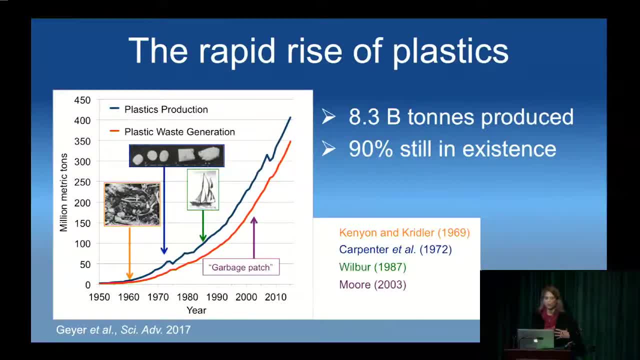 and described this pollution problem in a very visual way. that has sort of led to some of these images and descriptions of appalling islands of trash. But he coined the term garbage patch in this article And it really took hold. People finally had a vision of what this might look like. 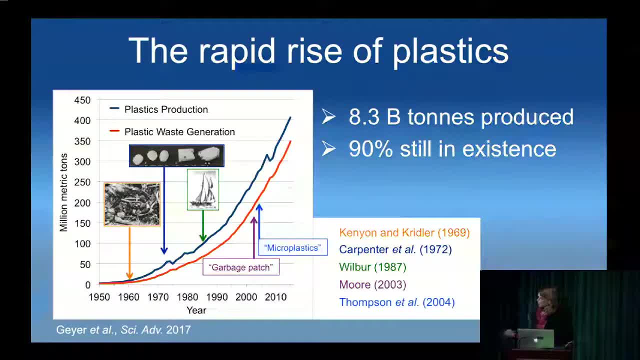 And just a year later Richard Thompson in the UK published a paper where the term microplastics was first used and first described. So if we look at sort of the scientific interest and scientific articles that have been written about marine debris or plastics in the ocean since then, I would argue that that curve probably 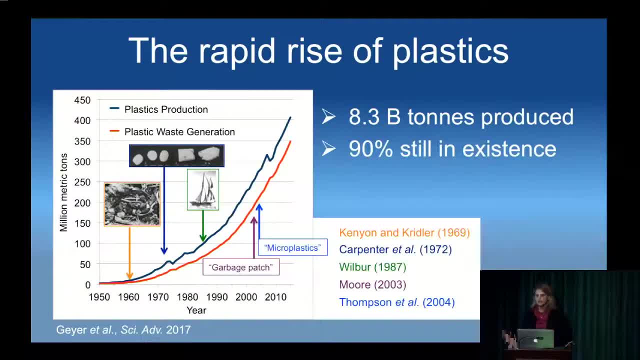 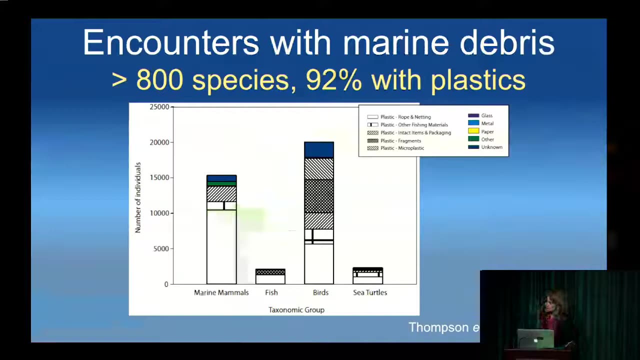 looks something like these curves. There's been a tremendous increase in scientific attention to the topic. I think that's in large part due to the tremendous increase in public attention to the topic. So why do we care about this? I mean, of course, there's an aesthetics problem and we should clean up our messes. 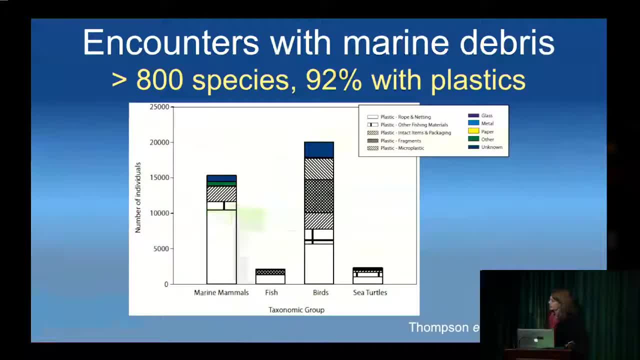 But really I think most people are concerned because of the potential impacts of marine debris with marine life. So this is a figure showing the number of individual animals that encountered some form of marine debris, according to taxonomic group: marine mammals, fish, birds and sea. 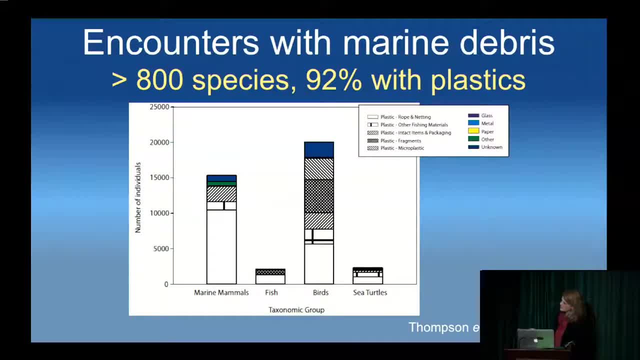 turtles, And this color coding is a little bit crazy, But all I really want you to see is that the black and white parts of these bars is describing interactions with plastic debris, And the colors are other materials like glass, metal, or they're unknown. 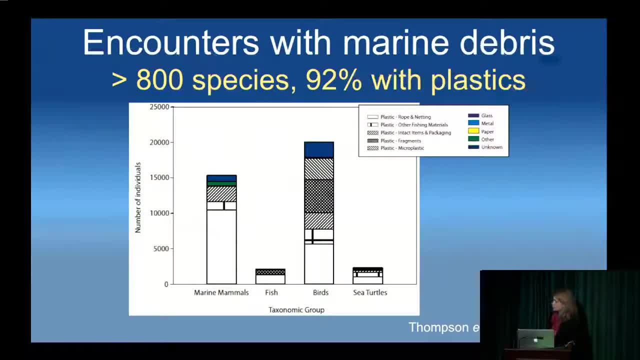 And so in this study, which was published a few years ago now, where they did a literature review, they found evidence of encounters with marine debris in more than 800 species And of those encounters, 90% of those encounters were with plastics. 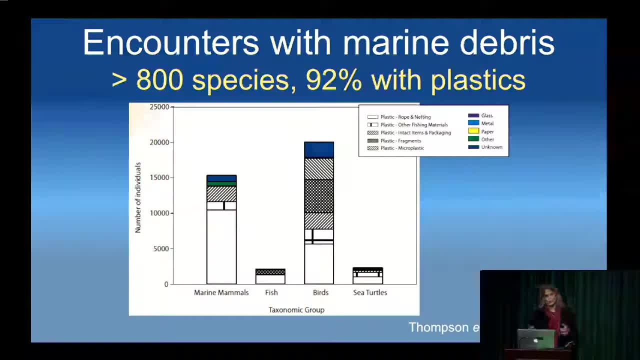 And, in fact, 17% of those species were plastic, And so the number of species that were encountering this debris were listed as threatened or endangered on the IUCN list. So these are species that are already threatened, And, in fact, we're talking about tens of thousands of animals. 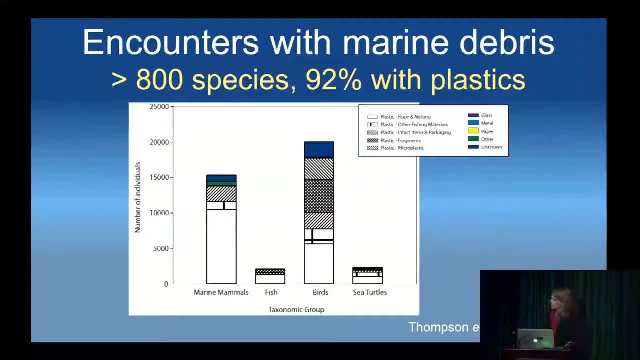 And in some cases, we're talking about all of the species. So all the species of sea turtles, for instance, have been interacting with marine debris, and about 50% of species of marine mammals and seabirds. Well, what are these? 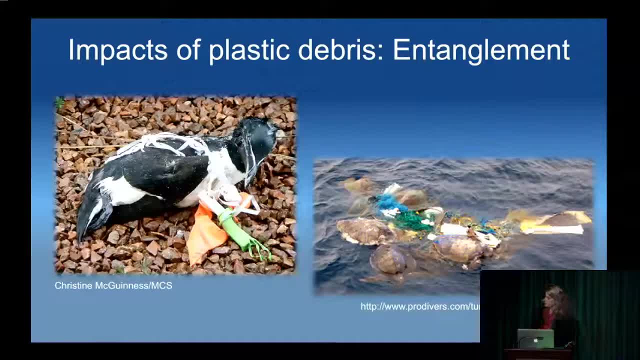 What do I mean by encounters? So marine debris encounters take a few forms, And you'll be familiar with some of these. The most common ones are sea turtles. The most obvious, I think, is entanglement. So here's an example of a bird entangled in what looks like a balloon string and some. 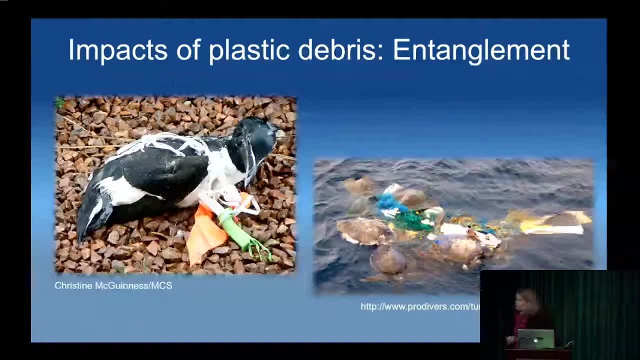 sea turtles, with probably some derelict fishing gear. So entanglement causes pretty obvious consequences. There can be very severe injury, can be linked to death. So we know that there is certainly a risk to animals when they encounter some of this debris. 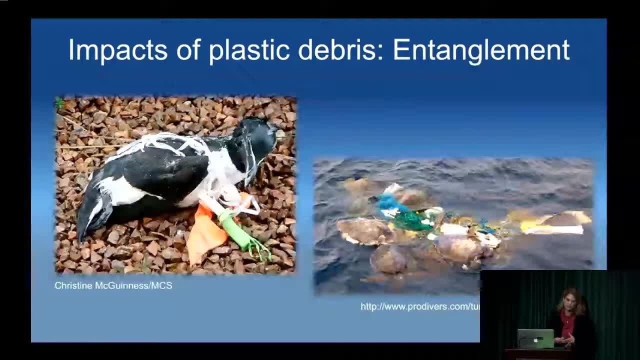 And the entanglement debris is often fishing gear or fishing line. There can also be anything really looping, So packing straps that go around, sort of cartons or bait boxes. anything that's looping can be a threat to these animals. What we know is this is a threat to individuals. 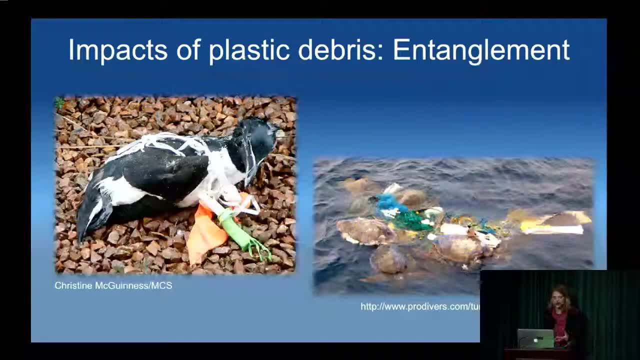 What we don't know is what the impact is on populations, So especially a population of a threatened species, for instance, And that's very hard to know because we don't encounter all of these animals. Much of what's reported is what's been you know. you report what you can find, or that. 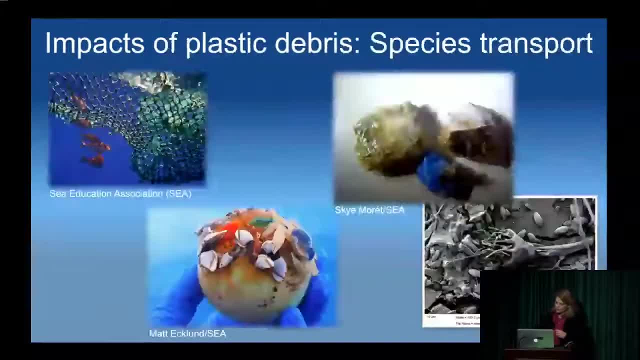 you can see, You can't survey all sea turtles, So this is a very clear risk, The thinking about: Okay, So not just large debris going to smaller debris. we know that marine life is interacting with it as a substrate or as a sort of floating platform. 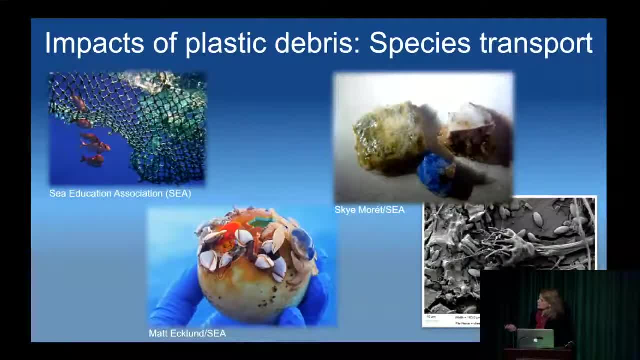 So species are transported in association with debris. In this case, we're looking at some fish that are swimming below this net. We know that fish tend to swim underneath things that are floating. This is why fishers create fish aggregation devices to try to draw the fish to them. 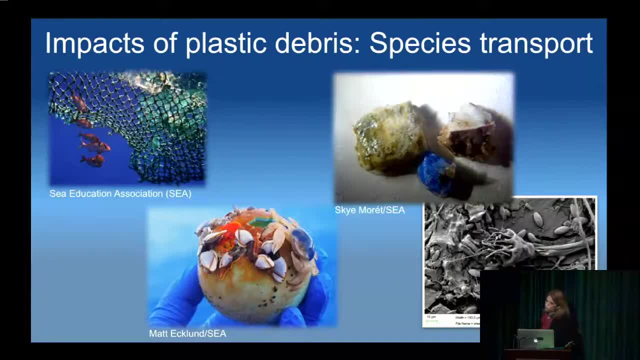 And so in this case we could have species that, just by following this debris, can end up outside of their normal ranges. Here we're looking at now species that are actually using the debris as a platform, So this is likely a child's ball from that Japanese tsunami. 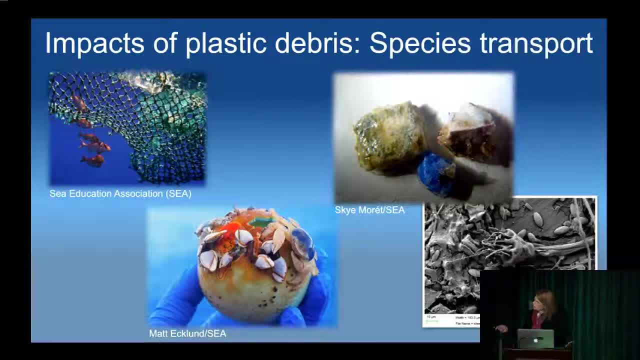 And what you can see is it fits in the palm of your hand. There's this crab here, There are barnacles on it And these are traveling along with that debris across the ocean. There was a recent study, about a year ago I think, by Jim Carlton down in Williams, Mystic. 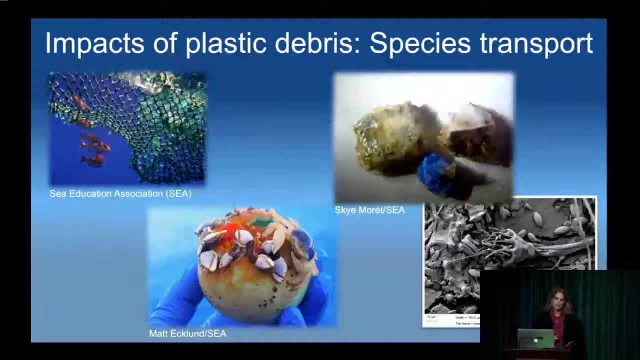 documenting more than I think, close to 300 species, 300 living coastal species that were transported by debris from the Japanese tsunami over the course of six years, And this was really an unprecedented rafting event, the consequences of which are really not known yet, because we don't know if these species were able to establish in a place. 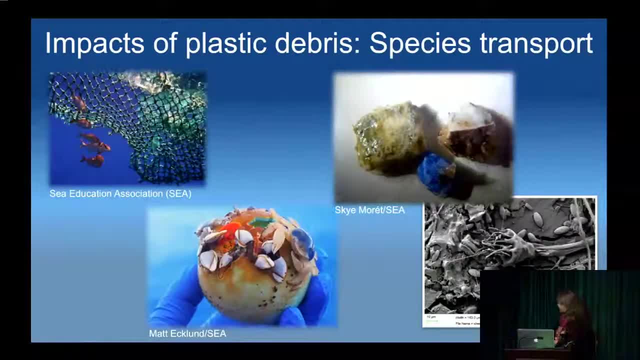 then become invasive. That is the concern. But even if we go down to these microplastics, there are rich communities living in these biofilms, communities of microorganisms. So this was a paper by Eric Zettler, formerly of SCA, and other colleagues. 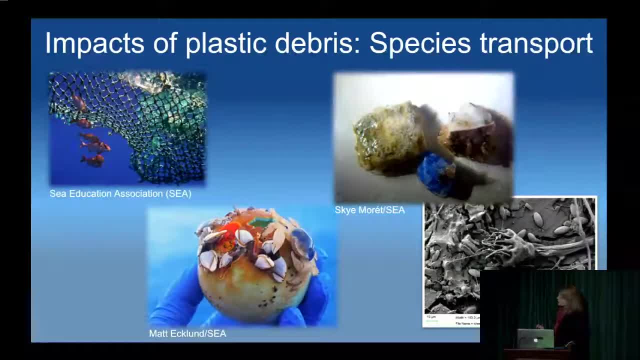 Linda Amaral-Zettler at the NBL and Tracey Minzer, formerly of HUI, that looking at the communities of microorganisms living in these biofilms on microplastics And what they found is that the communities of organisms living on the plastic are quite 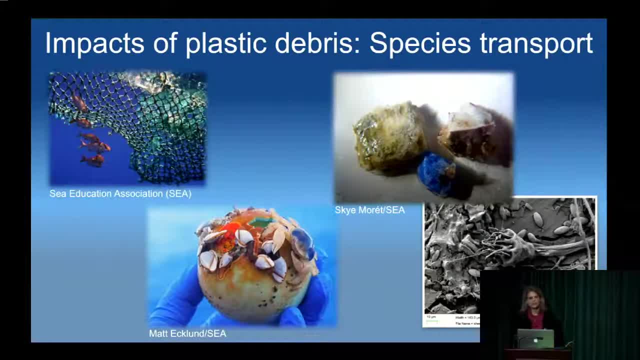 different from what's living in the surrounding seawater or even living on natural substrates, And at this point we don't really know what they're doing here, how they're making a living. if there's big questions about whether or not they're degrading the material, 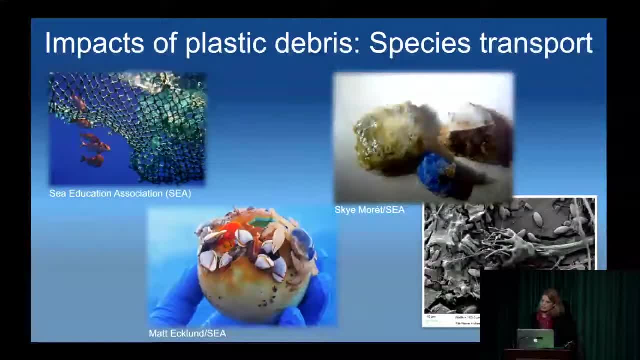 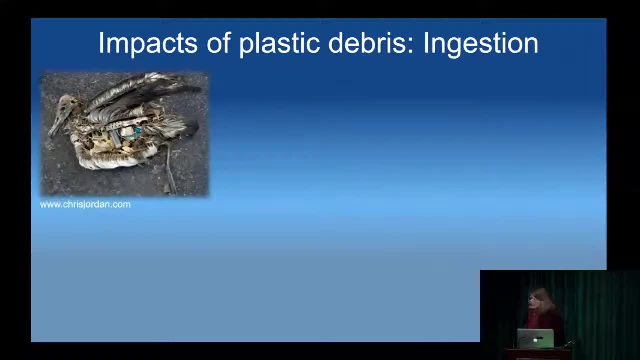 But they're clearly living, they're creating their own ecosystem. here that's been dubbed the plastosphere. So the final impact I'll discuss, but not necessarily. the final impact of marine debris and plastic debris is probably something you've heard of too and been concerned about. 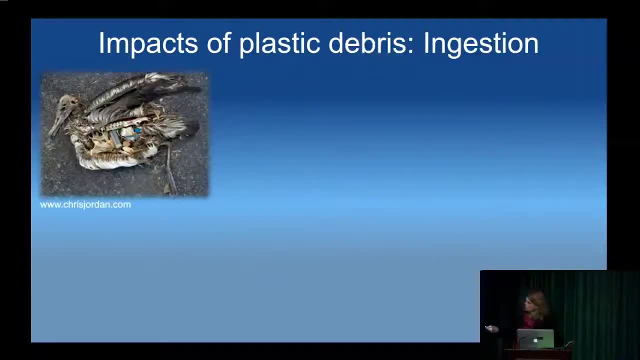 is ingestion. So I showed you that early seabird image, which the modern-day version looks like this. This is an albatross chick on Midway Atoll, photographed as it was found, And you can see inside its belly a cigarette lighter and a bottle cap and other fragments. 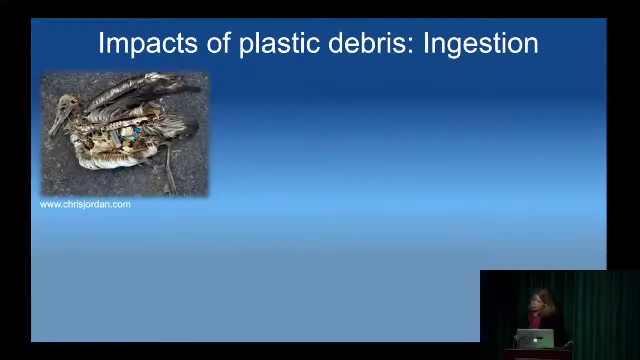 of plastic And this image has largely become sort of the poster child. The poster child, The problem of ingestion of plastic debris, Because it hits home when you see things that you recognize and maybe that you use every day. So at this point we know that at least 220 species have ingested plastic debris. 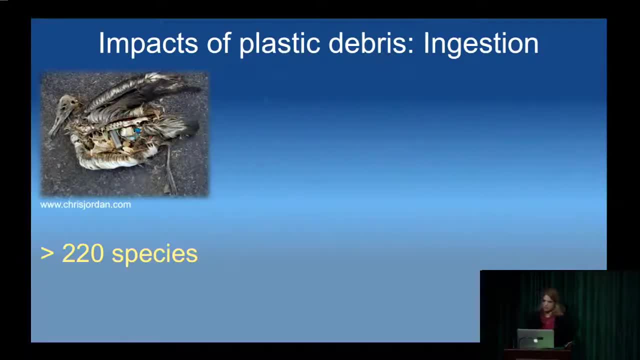 And these are animals that are not just sort of large or charismatic animals, but animals even as small as zooplankton. So these are zooplankton collected in the North Atlantic that had ingested microplastics inside of them. This is a study from my colleague, Deb Goodwin at SEA. 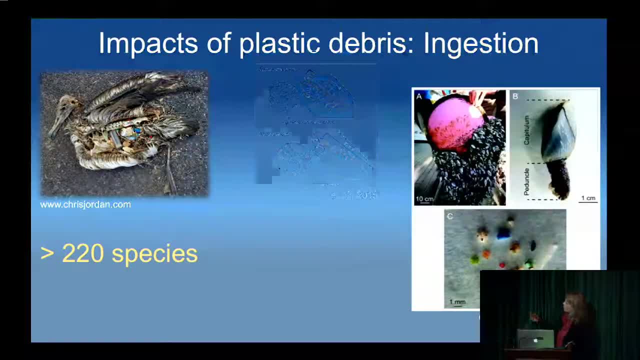 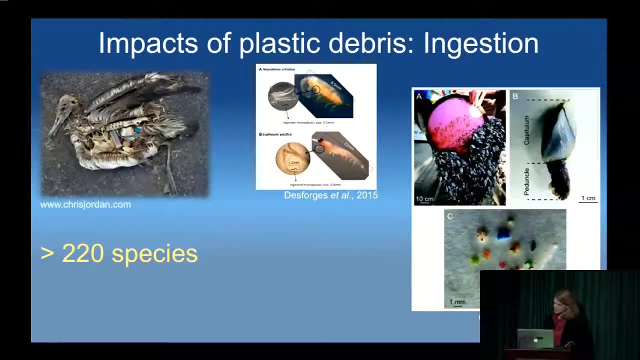 And a colleague of mine And a colleague looking at barnacles that were living on this buoy, again probably from the Japanese tsunami, And inside the barnacles they found these tiny pieces of microplastics And then, yes, fish and, of course, large marine mammals and turtles and other animals. 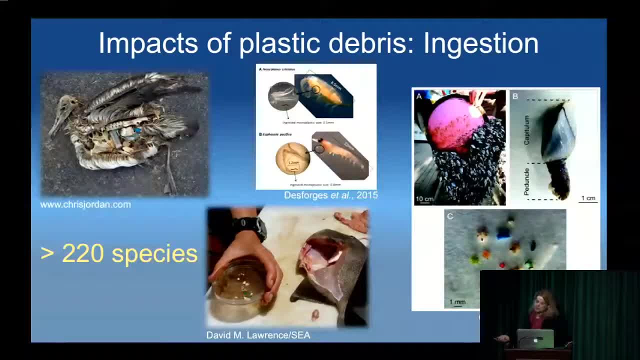 are also eating these particles. So this is a fish that was swimming below that five-gallon bucket that I showed you at the very beginning of the talk. That fish was swimming under the bucket following it And, by some lucky chance, both ended up in our plankton net. 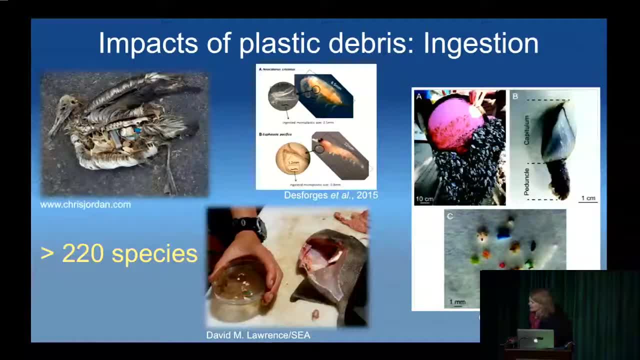 And when we cut open this fish, we found 42 pieces, 42 pieces of microplastic in its stomach. So we know that. you know: the smaller the particle, the more things can eat it And the big whales can eat. you know yards and yards of plastic sheeting and carp hearts. 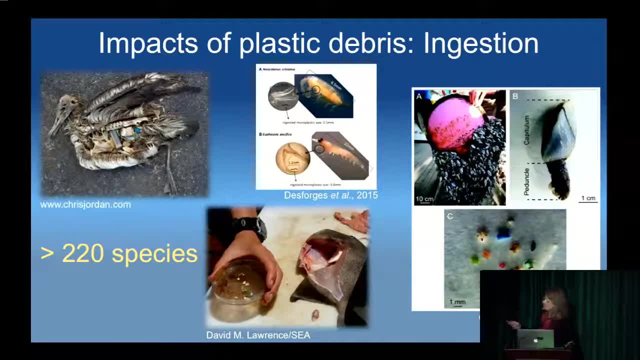 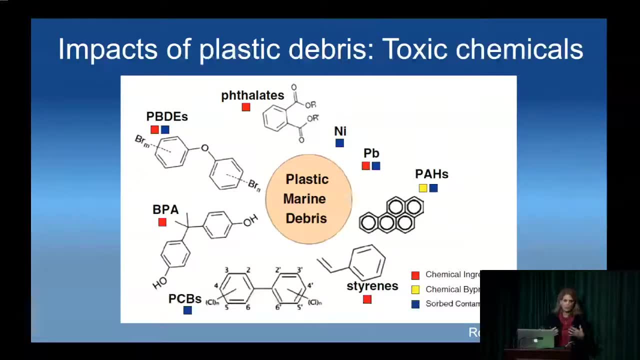 and I mean the things you read about are just appalling. But even the smallest animals in the food chain are ingesting microplastics. Now, part of the reason this is of concern. of course, nobody really should be eating plastic. We don't eat plastic voluntarily. There's no nutritive value. There could be internal injury caused, Especially if you're eating microplastics. You're eating a big carp heart that clogs up your insides or causes internal damage. But I think a big part of the concern has to do with the chemicals that are associated. 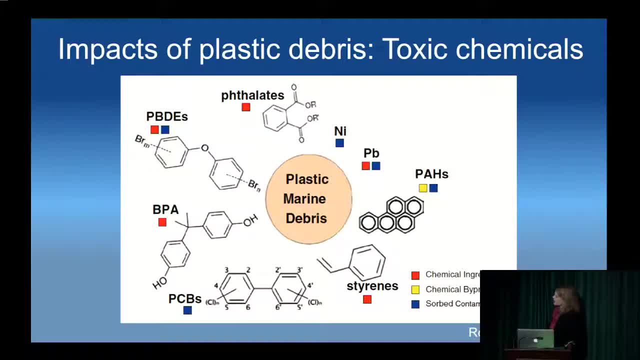 with the plastic debris in the marine environment. So plastics have a variety of chemicals associated with them. Some of them are actually ingredients, So chemical additives that alter the material's color or flexibility, or their antimicrobial Lots of added chemical additives are included. 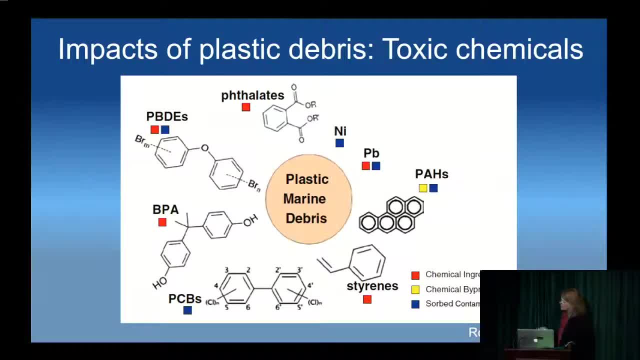 There's also byproducts due to the manufacturing process, And many of these may be toxic or hazardous. And then there's also a category of contaminants that are already present in seawater that would prefer to stick to plastic rather than be dissolved in seawater. 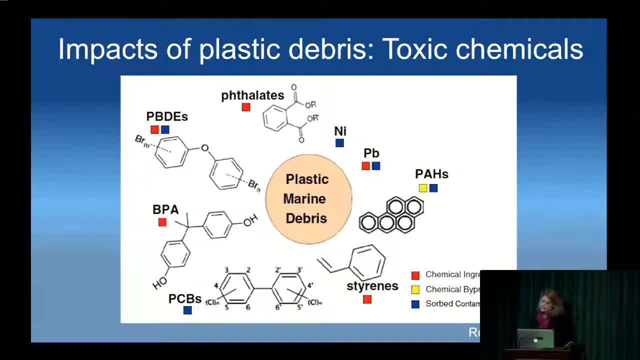 So these are legacy contaminants like PCBs and DDTs. We know that these chemicals can be harmful And the question, the big outstanding question, is: if an animal eats the plastic debris that has these chemicals associated with it, do those chemicals transfer into the tissues? 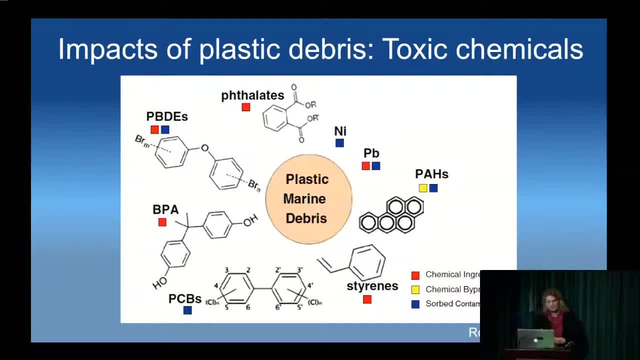 of the organism and cause damage. And then, taking that a step further, if we eat that animal, are we poisoning ourselves with plastic? So these are very open questions and, I would say, the focus of a great breadth of research at this point. 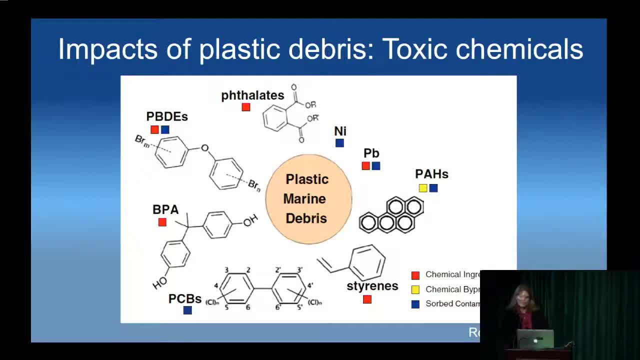 People are conducting controlled laboratory experiments and have found evidence of harm either to individual animals or growth or reproductive effects. The challenge is that a laboratory experiment, by necessity, is constructed to test a single outcome. So there's a certain type of animal, a certain type of plastic with a certain chemical constituent. 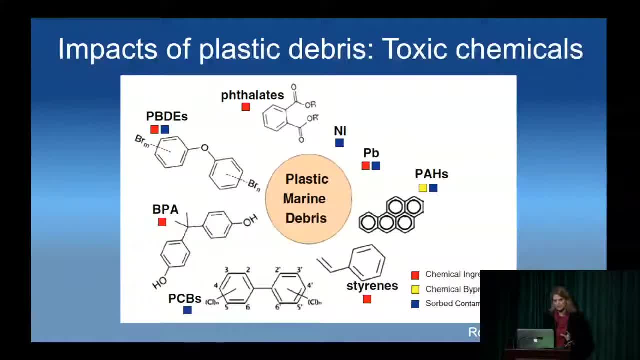 You know, size and shape of plastic is constant. You're trying to keep a lot of things controlled and you'll get an outcome, and that is very informative. But you can't easily take that result and apply it to the natural environment, where 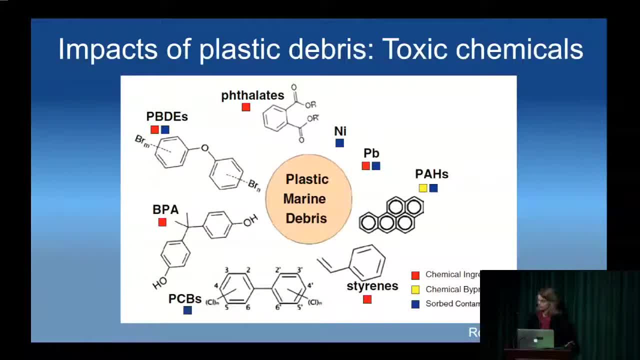 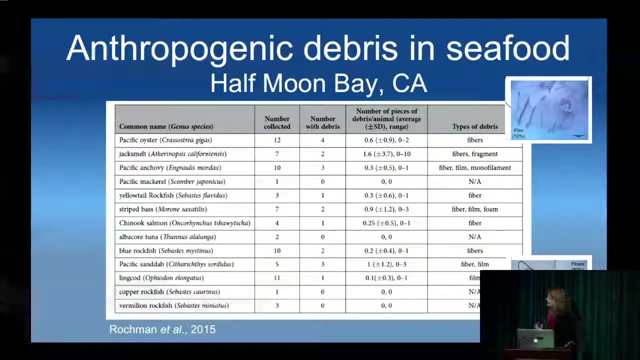 we really don't even know what kinds of plastics many of these animals are exposed to. So at this point I would say there is certainly reason for concern. I'm not panicking, But we should continue studying At this point to sort of try to figure out what these impacts might be. 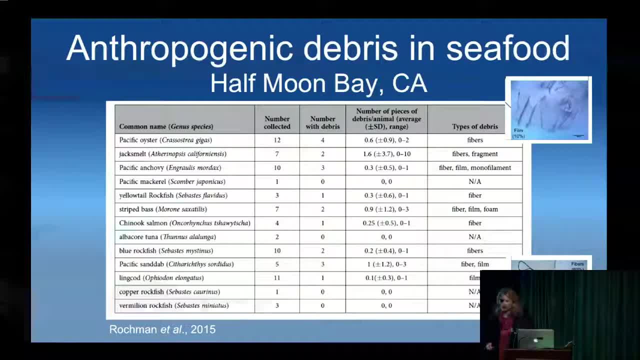 But back to this human health question which really, I think for many people is one of the ultimate goals to understand- is you know, is there plastic in our seafood? This is a study from my colleague, Chelsea Rockman. She gathered seafood from a seafood market in Half Moon Bay, California, and analyzed 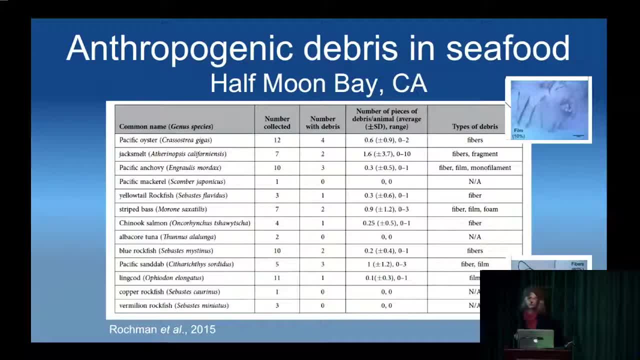 it either the whole animal, if it was shellfish, or the gut, if it was fish, for microplastics. And actually, yes, There was a study. And actually, yes, there's plenty of microplastics in our seafood. 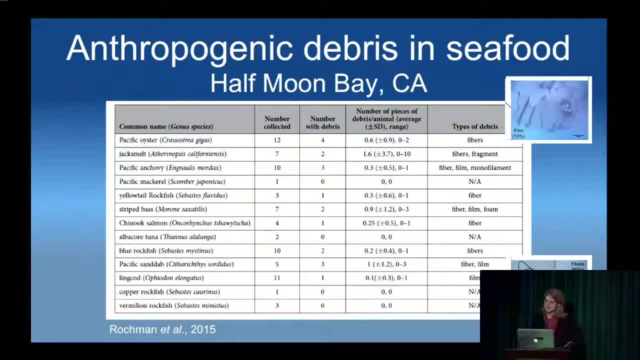 It was, I would say, maybe 20%, 20, 25% of the animals they looked at had microplastics in them. Typically there were small numbers of particles: 0 to, at most, 10 particles. Many of them were these fibers. 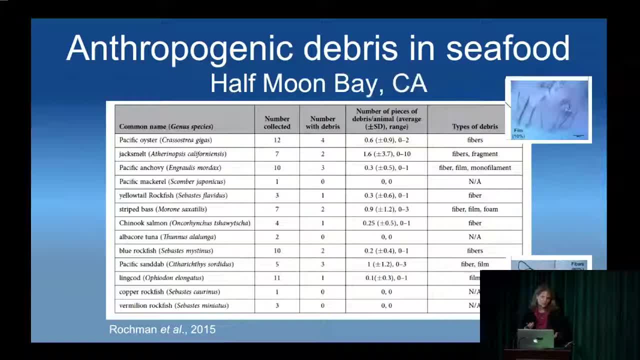 The question is: does it matter? So I mentioned that there's also been microfibers in our water and in our beer and all these kinds of things. In terms of seafood, we don't typically eat the guts of fish, And so, at least for particles. 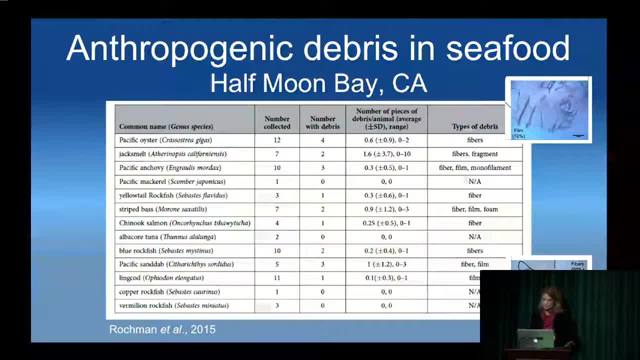 Okay Above a certain size. They may stay in the gut of the fish. They might be egested. We're probably not eating those, But certainly with shellfish it's in the tissue. We eat the whole animal. So we are probably eating microplastics in our seafood. 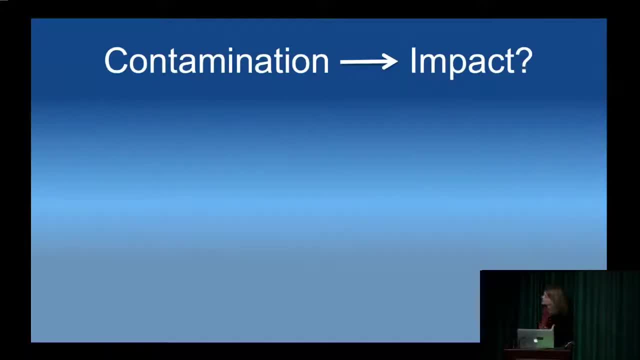 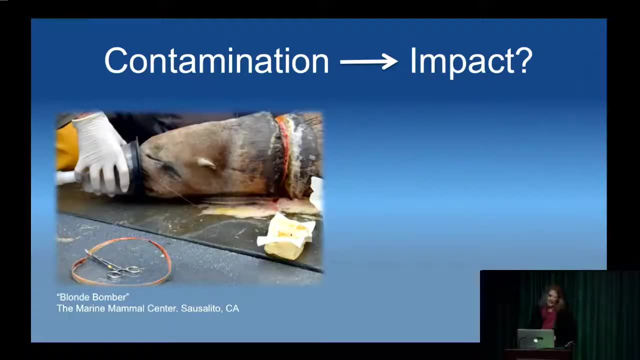 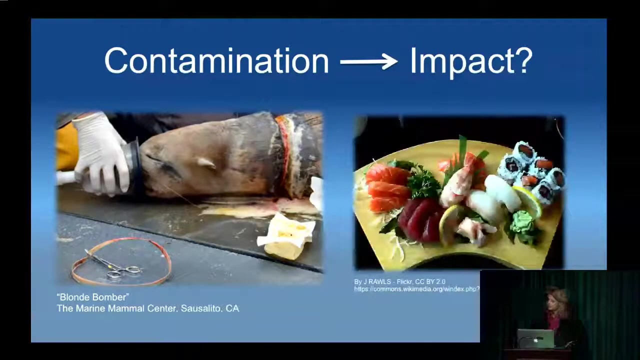 But, as I alluded to a second ago, contamination doesn't necessarily imply an impact. So contamination, we certainly know that animals are encountering debris. There are certain instances where we can find a very clear harmful impact. But in the instance of seafood, I think the germs 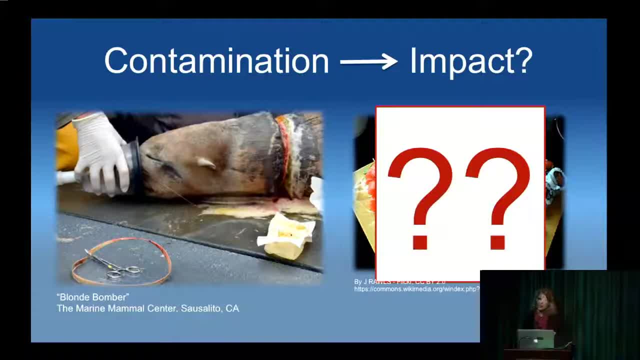 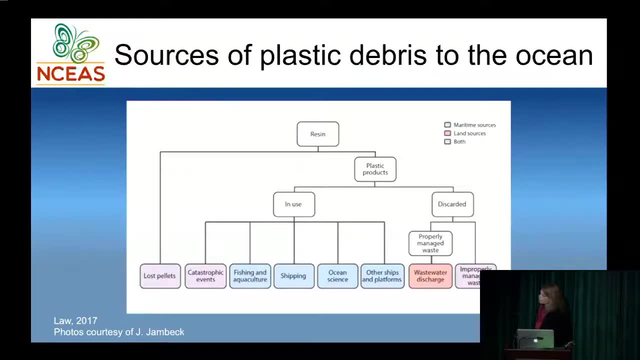 The jury is out whether or not there is a measurable impact to either the marine animal or to the humans eating it. Cause for concern. Okay, I want to take a step back and think a little bit about how all this plastic is getting into the ocean. 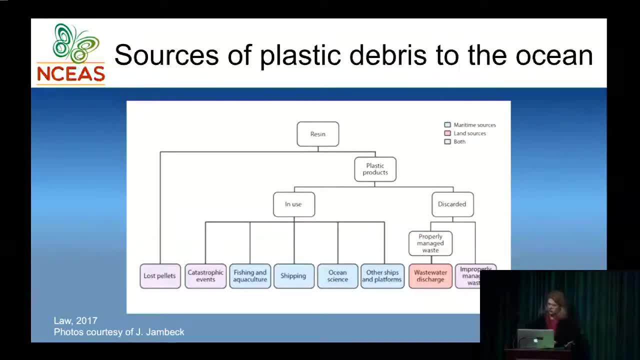 So this is a little bit of a complicated flowchart, But we're not going to talk about it in great detail. But the idea is that plastics start out as resin, most of which are formed as these little resin pellets that then get formed into plastic products. 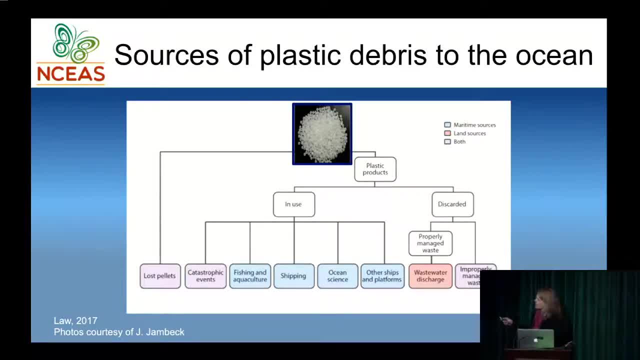 Those plastic products are either used or they're discarded as waste, And then There are pathways by which that plastic can end up into the ocean. It's color coded by whether it's an activity at sea or an activity on land, or both, So we can. certainly some of these pellets can be lost. 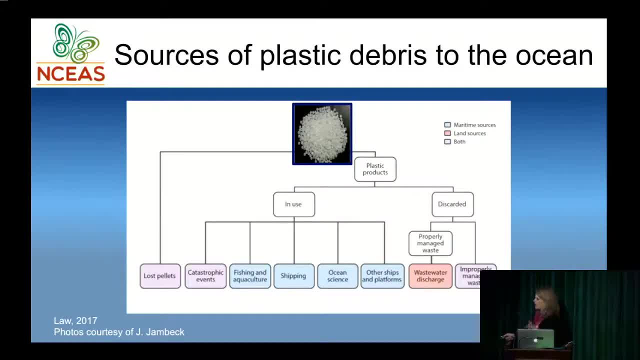 There can be catastrophic events like tsunamis that dump a whole range of materials into the ocean at once: Lost fishing gear, lost shipping containers full of Nike shoes or rubber duckies. Oceanographers deploy plastic in the ocean and we don't always intend to recover it. 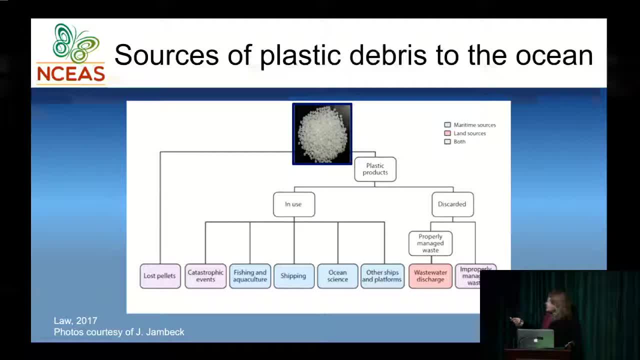 We can have losses from other types of ships and platforms, But the only category that we really have an estimate- a quantitative estimate- for from a source is down this discarded pathway. So these are losses that are probably not intentional. You're using the items, not intending to lose them. 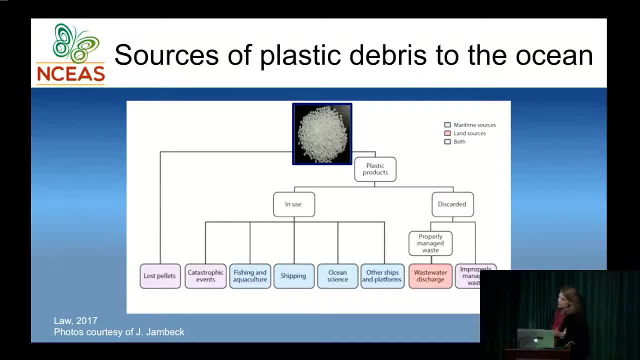 In terms of discards, we can think about properly managed waste. You put your garbage into the garbage can and it gets handled, whether it's in a landfill or burned. Properly managed waste shouldn't enter the environment, the exception being wastewater discharge. 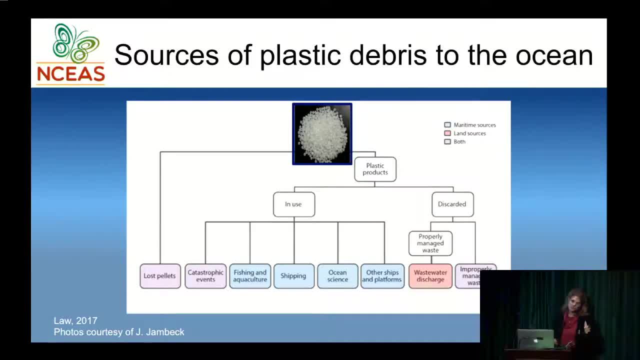 If some of these smallest particles don't get filtered out, you can imagine that the outflows that go into the environment can contain some of these small particles. But really, what we thought most about- because we're suspicious that this might be the largest source of plastics to the ocean- is the improperly managed waste category. 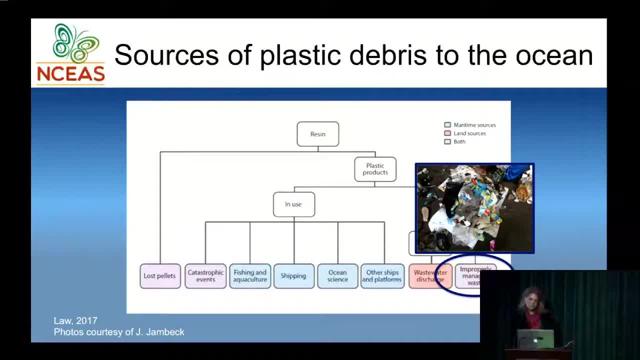 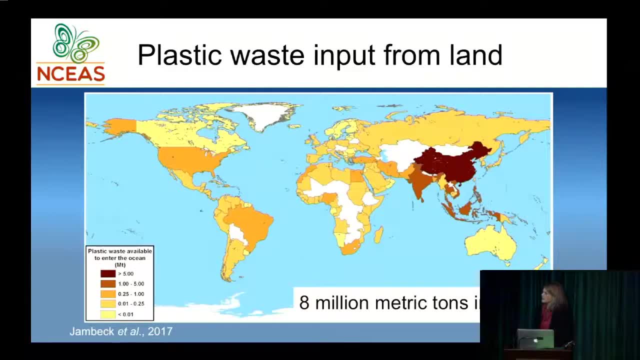 So what happens to all of that waste if it's not properly managed, either because of deliberate littering or accidental littering, or because there simply isn't the waste management infrastructure to handle it? So a study that I was involved in As I was looking at it, I was looking at it. 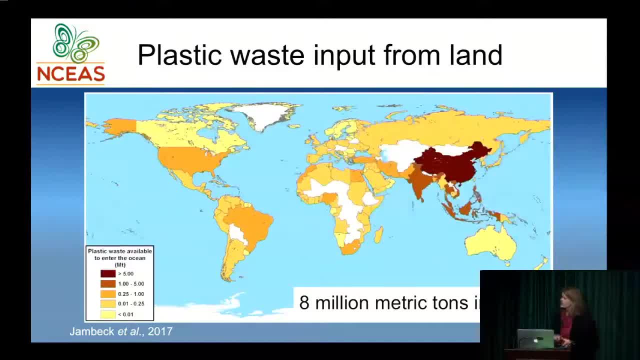 I was looking at it. It estimated the amount of plastic waste generated on land- that is, input to the ocean- in a single year. So what's interesting about this study is that we had absolutely zero data from the ocean. The way we did this was we took waste management data- data that estimated how much waste is. 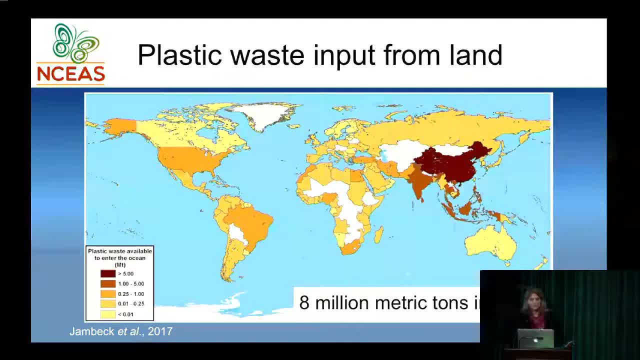 being generated in countries around the world. This was data that came from the World Bank- How much of that is plastic And how much of that is not properly captured and contained. And the way that this was reported was by country, not because we wanted to point. 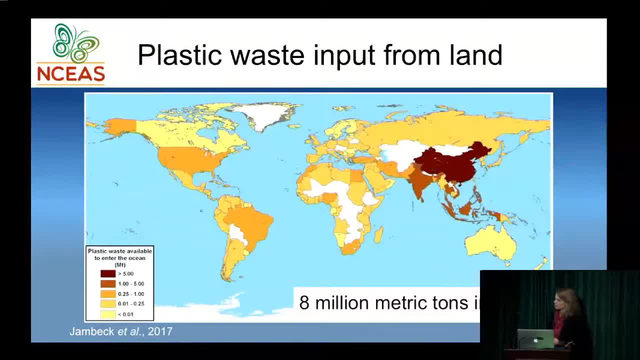 fingers or figure out where the bullseye was on the map, but simply because the data were reported that way by the World Bank. So first, the top line message is that the number is big: Eight million metric tons of plastic, we estimate entered the ocean from waste that was generated. 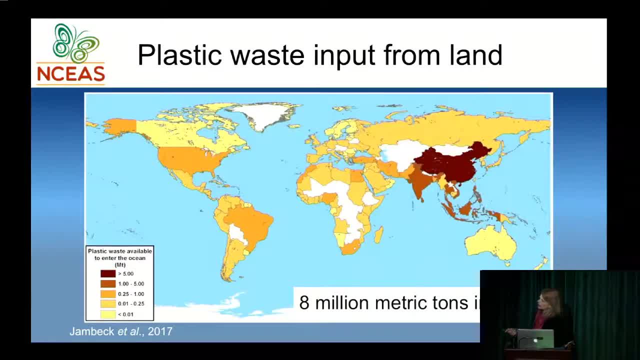 on land. When you look at the map, which is the warm colors are color coding, the highest values- you see that there's a very, very clear high region here in Southeast Asia, And we think the reason for this is that these are, this is a region where there are rapidly 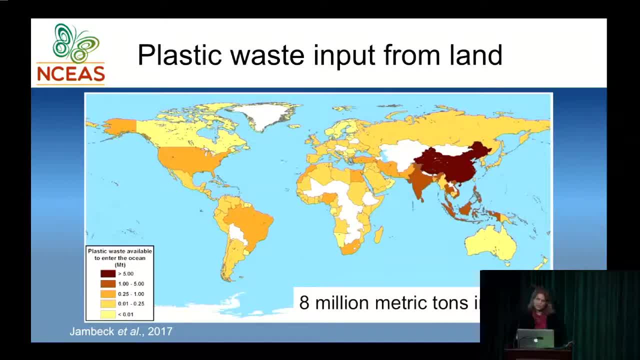 developing economies. With that is increased consumption, increased waste, and yet these are economies that have not yet built the infrastructure to deal with that increased waste- waste much of which is made of plastic. So this is definitely an area to focus if we want to stem the tide, if we want to stop. 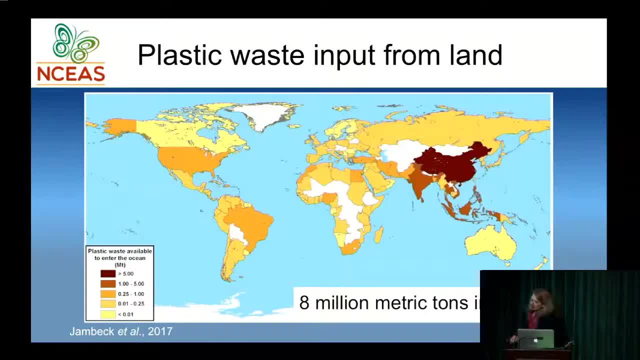 the waste from going into the ocean. But what's really important is not to just say, oh, it's China's fault. When we look at the list of top 20 countries in putting plastic waste to the ocean, the United States is number 20 out of 192 countries. 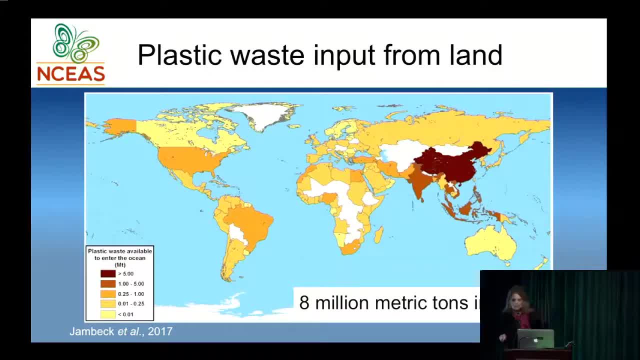 And the EU collectively is number 18.. And the reason for this is not because we're litter bugs, necessarily, But if you look at the United States, we have a very large coastline and we have a very high coastal population. And, equally important, we generate more waste- more plastic waste per person per day than 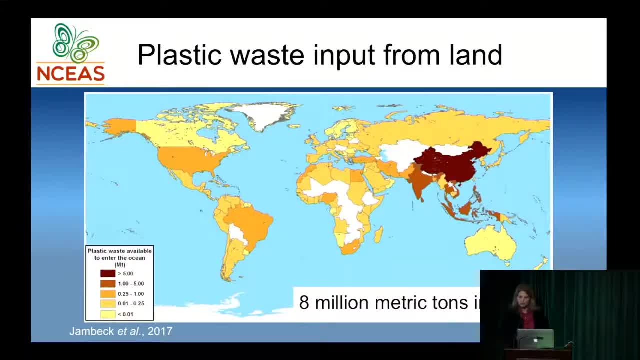 anywhere else in the world. So we create a tremendous amount of plastic waste, Even if all of us do the right thing, The right thing all the time, but accidentally the candy wrapper flies out of your hand. one day. when you add up all those lost candy wrappers, plus the intentional dumping and 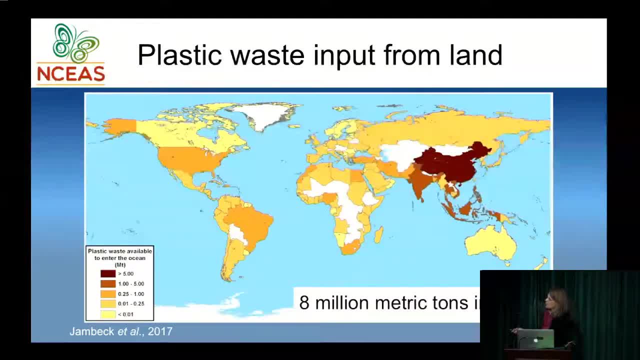 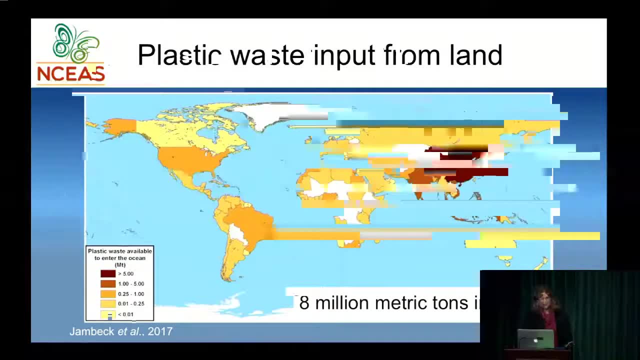 sort of bad actors. it adds up to a big number, So this is not something that we can ignore. This is a global problem and we are contributors. Okay, Now we come to SEA. So this study: here, as I mentioned, we didn't look at a drop of ocean data. 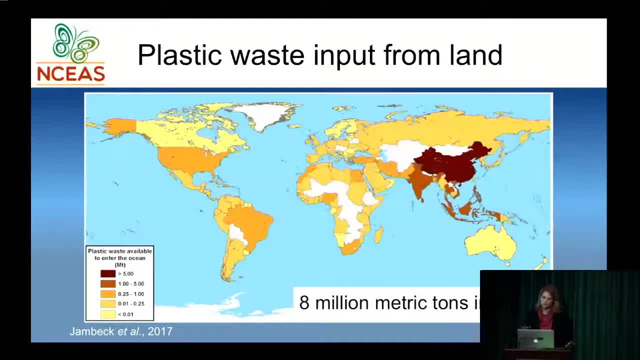 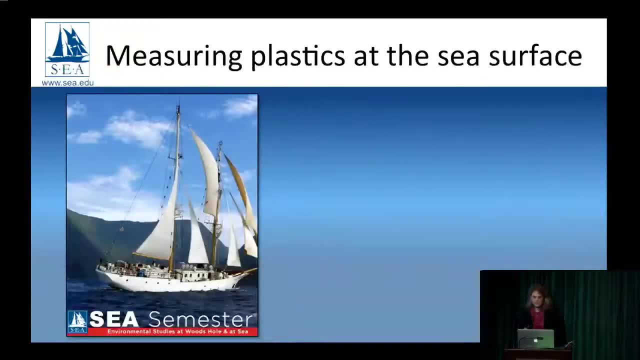 So we've got a number for how much we think is going in from one of a multitude of sources At SEA. we go out to sea and we measure the ocean. So another way to try to gauge this problem is to say: well, how much plastic do we think? 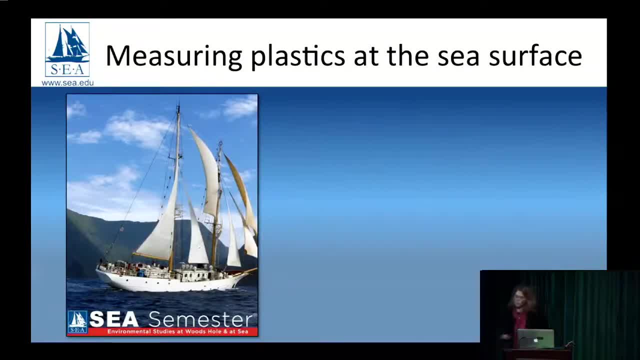 is out in the ocean by going out and sampling it. So if folks aren't familiar with SEA Education Association and SEA Semester, we are an educational nonprofit here in Woods Hole. We have been operating since 1971, and we run the SEA Semester program for undergraduate. 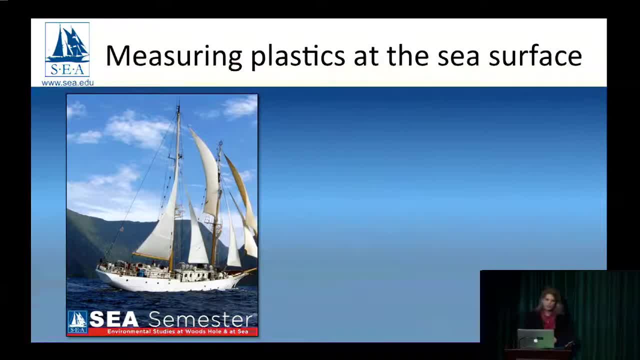 students who come to us for a sort of off-campus study abroad experience. They come to us, They come to our campus, which is halfway from here to Falmouth on Woods Hole Road, and they live on our campus and study for six weeks and they study the ocean environment. 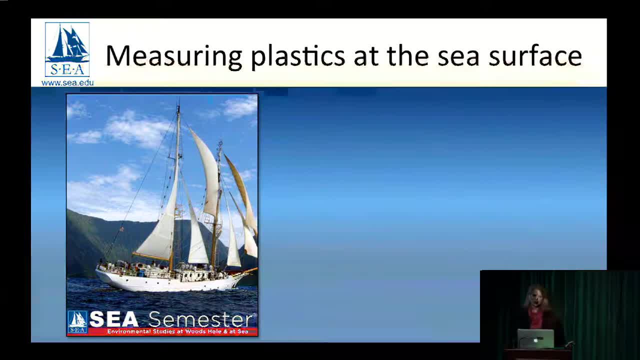 from a variety of perspectives, including scientific, of course, but also maritime history, marine policy, and they learn to become full-fledged crew members on board our tall sailing ships, which are also scientific research vessels. So they come to us for six weeks. 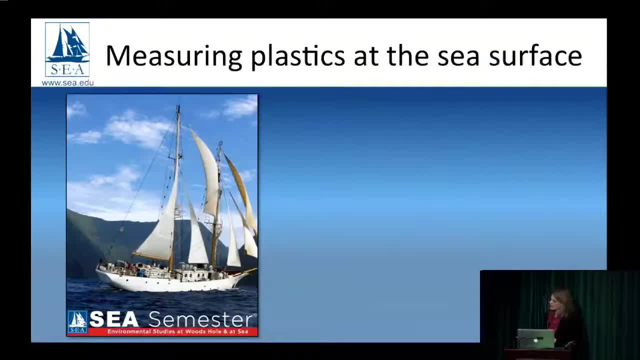 They propose, they construct research projects that they're going to carry out when they go out to sea on our ship, Either in the Atlantic or our ship in the Pacific, and then they conduct oceanographic research during their six weeks on sea, as they're also fully operating the ship. 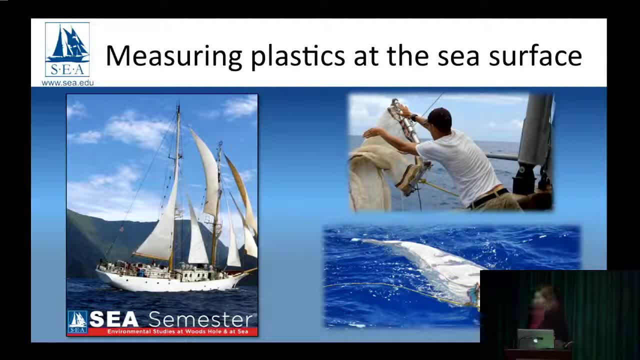 So early on we adopted the NuSTON net- a surface-towing plankton net- as a workhorse piece of gear For many reasons. you can learn a lot by sampling the ocean surface. it's accessible and students can pretty easily learn how to do all of the work to deploy, recover and analyze the data. 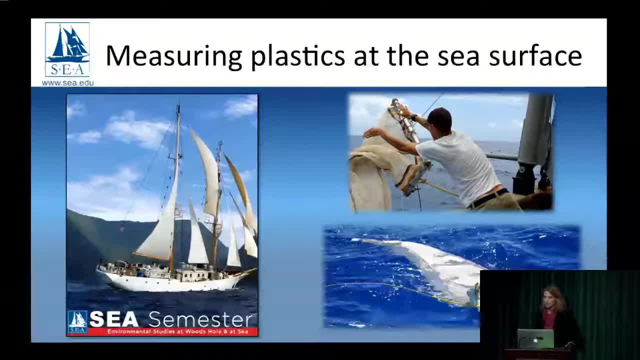 by themselves, And a big piece of our program is developing leaks. So if you have any questions, please feel free to reach out to us and we'll be happy to answer any of your questions. And I'll be happy to answer any of your questions. 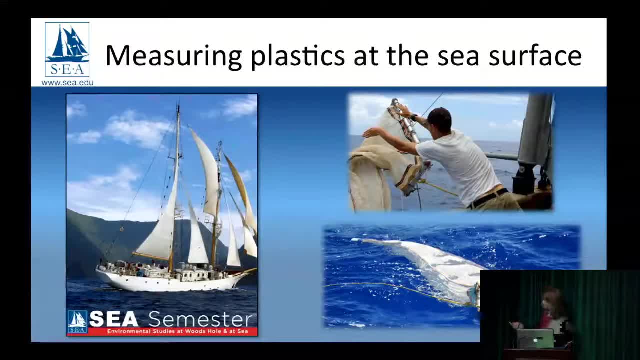 So we have this surface-towing plankton net. It's a meter wide and half a meter tall, and we tow it off the side of the ship for about a half an hour. And then here's a bird's-eye view of the net being towed off the side of the ship. 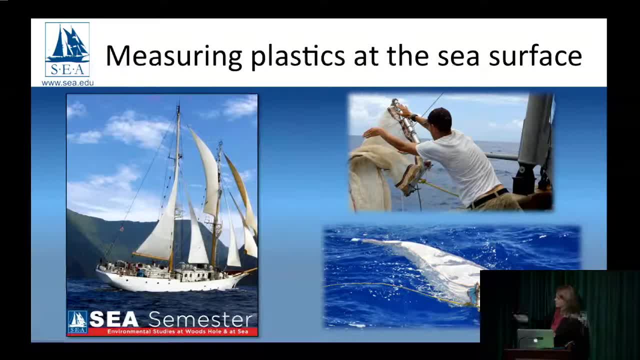 The net mesh is about a third of a millimeter in size, so pretty small mesh, And we tow it at a pretty slow ship speed. And then we bring that net aboard and rinse its contents into a sieve. and here comes the fun part. 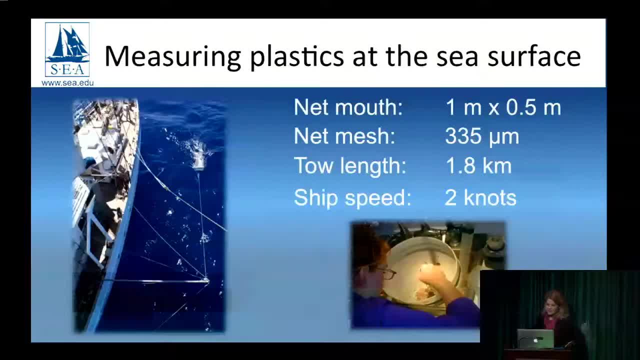 Students can see that this net is really heavy. So we're going to take that net off the side of the ship and put it on the side of the ship. And then we're going to take the net on the side of the ship and we're going to put it on the side of the ship and do it in a similar way, And then we're going to take that net off the side of the ship and we're going to bring that net aboard and rinse its contents into a sieve. and here comes the fun part. 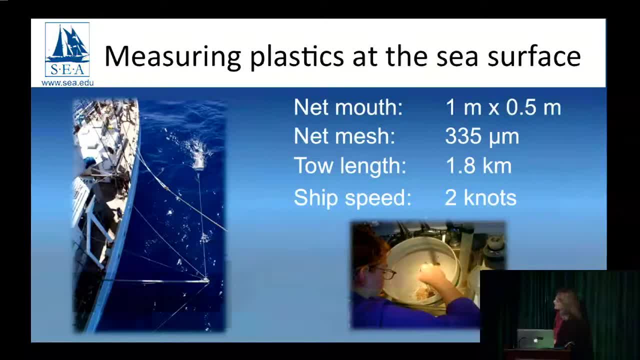 Students sit in the lab with tweezers and pick out individual pieces of plastic And from some further work that we've done now analyzing these samples, historically we know that the human eyeball does a good job selecting plastic at these sizes. If you start to get down to fibers at a large size, if you start to get down to fibers at 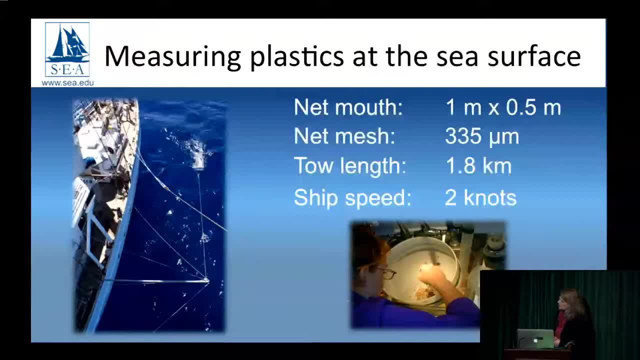 a small size, then you're going to have to work with your hands to figure out how to find the right size for the net. So we're going to take the net off the side of the ship and then we're going to take it off the side of the ship. 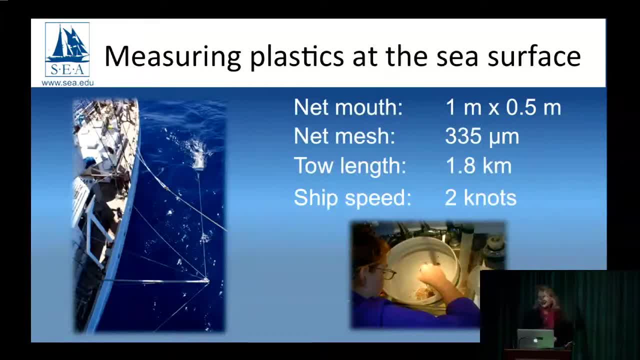 net, a board and rinse its contents into a sieve. and here comes the fun part: Students sit in the lab with tweezers and pick out individual pieces of plastic And from some further work that we've done now analyzing these samples, historically we know that the human eyeball does a good job. 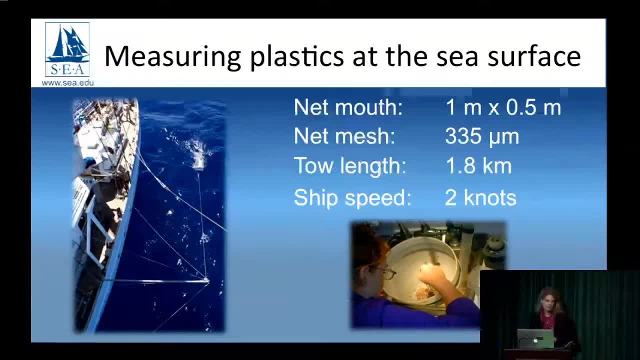 selecting plastic at these sizes. If you start to get down to fibers and things like that, you really have to use chemical identification techniques. But our students have been using eyeballs and tweezers for decades and they do a really good job picking out plastics. 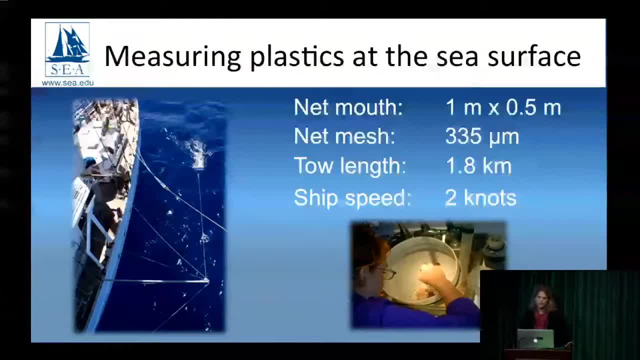 So when they pick out the plastics, we get a count number of particles for the netto and we divide that by the area of the sea surface that we measured and we report that concentration in terms of pieces per square kilometer. So what I'm showing you here is a map of the western North Atlantic. So we've got. 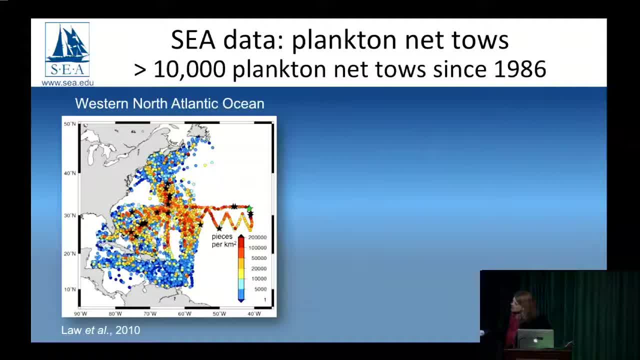 Newfoundland. we've got South America, here's the Caribbean Sea here And what you see, each dot represents a single plankton netto. that was conducted since 1986. So now we have more than 10,000 plankton nettoes. 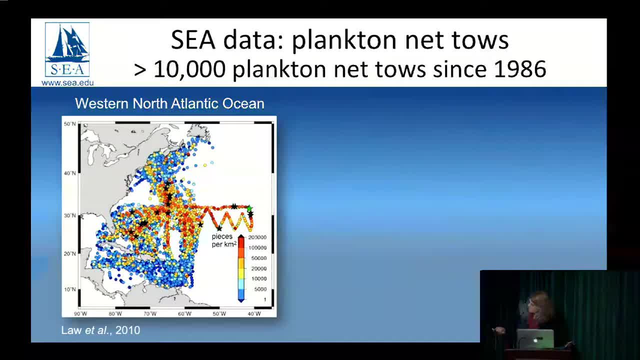 It's been towed and analyzed by our students over decades and it's colored by the plastic concentration in pieces per kilometer squared from zero, which is the dark blue all the way up to 200,000 pieces per square kilometer. So the red values are the high values and the stars are the. 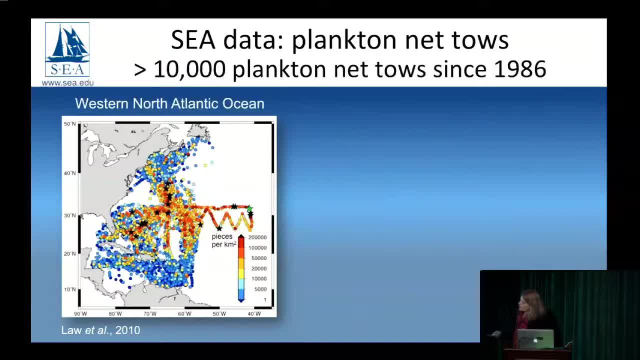 highest concentrations we've measured. So the first question, and especially coming from my background in ocean physics, was: well, where is the plastic and why is it there? So one thing that's a little bit surprising is that the highest concentrations, these black stars, you might expect. 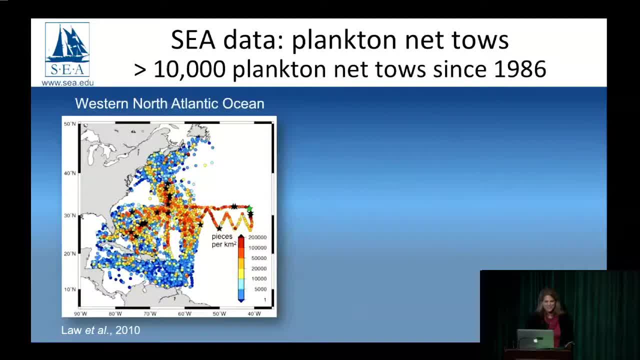 these to be pressed right up to the surface, but they're not, And so we've got a lot of plastic right up against the coast, because I just told you that 8 million metric tons of plastic is leaking off of our coastlines. But, in fact, these microplastics that we collect in the net, 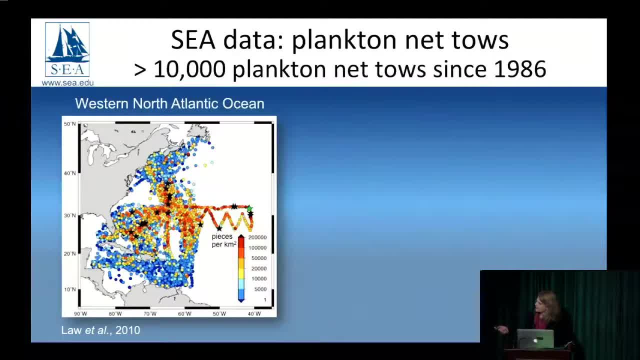 are all of the black stars are far from land and in fact, this green star is the highest concentration we've ever collected, and that's 26 million pieces per square kilometer and that was collected, quite literally, in the middle of the Atlantic Ocean, above the Mid-Atlantic Ridge. 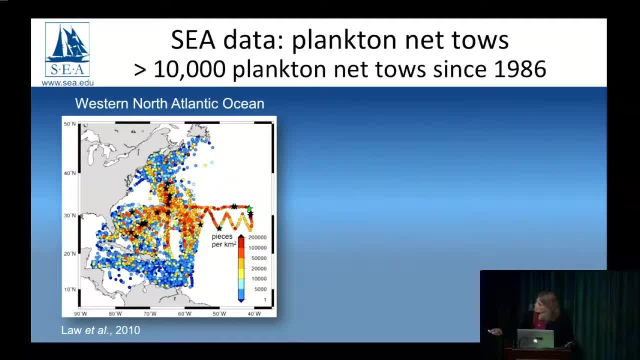 So when you look at this distribution, kind of squint your eyes and look at the warm colors- you'll see that this is a clear region where these plastics are accumulating. This is the subtropical ocean gyre and this is what people- this is really what the garbage patch is centered at- about 30. 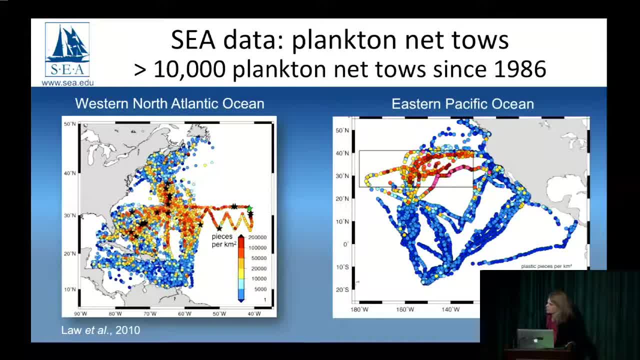 degrees north latitude. Now I also mentioned that we have a ship in the Pacific, so I want to show you our Pacific data set a little bit quickly here. So we're looking at the eastern Pacific Ocean. What's different about this map? it's the same in terms of one dot per plankton tow, The. 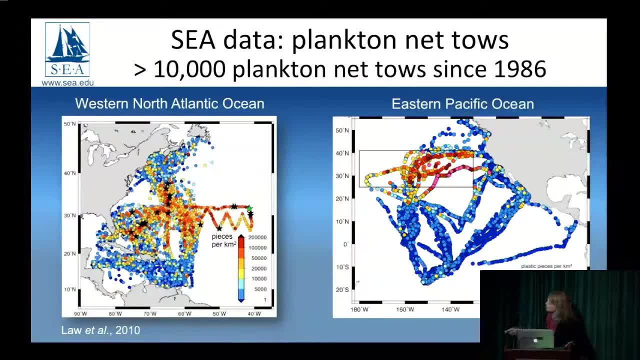 color shading is a little bit different because we've added a higher category here, but we're looking now at a much broader latitude range. So here's the Pacific Ocean and we're looking at a northern hemisphere. Here's the equator, So here's the northern hemisphere. We've got the. 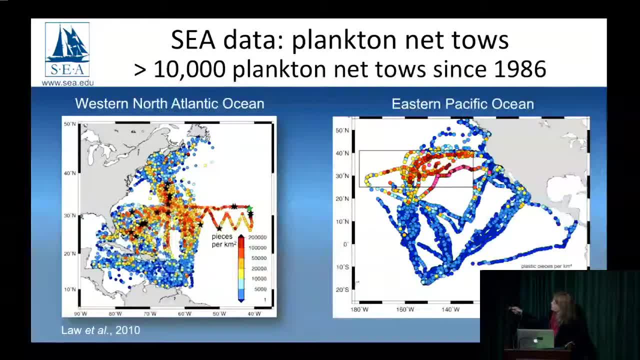 southern hemisphere. This is Tahiti, Hawaii, Mexico. So what you see is the highest concentrations, again, are centered at about 30 degrees north latitude. That's where the ocean currents are collecting them. But what you can really see in this image is that outside of that region, 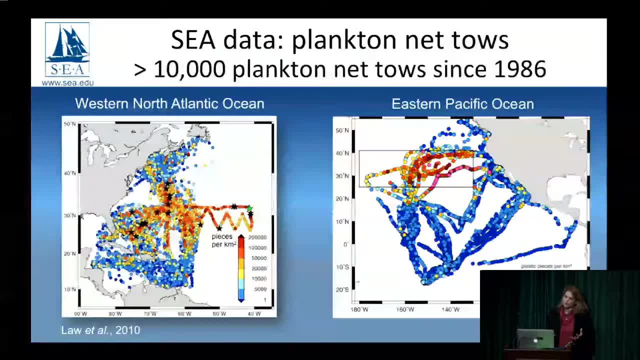 there are relatively low concentrations. So in the size ranges that we are collecting in our plankton nets, you can very clearly see the region of the ocean where they're collecting and where it's not. Well, why is that? So I have to tell you a little bit of. 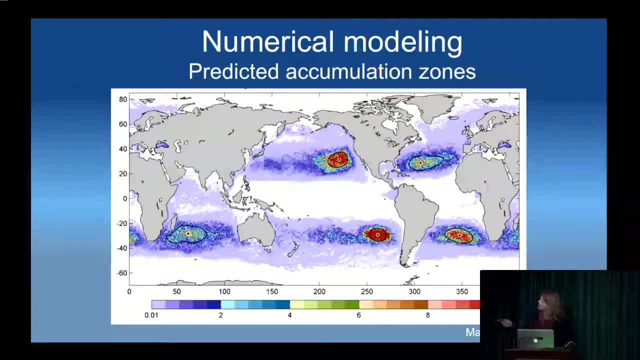 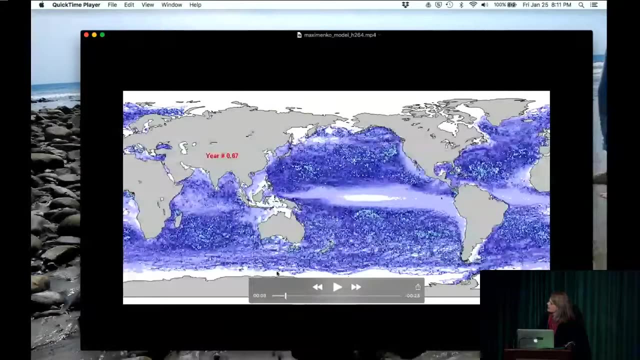 physical oceanography or I'd have to give up my card, So I wanted to show you. this is a numerical ocean model modeling ocean currents that was created by my colleague, Nikolai Maximenko, at the University of Hawaii. So we're going to look at a little movie. In this movie he started the 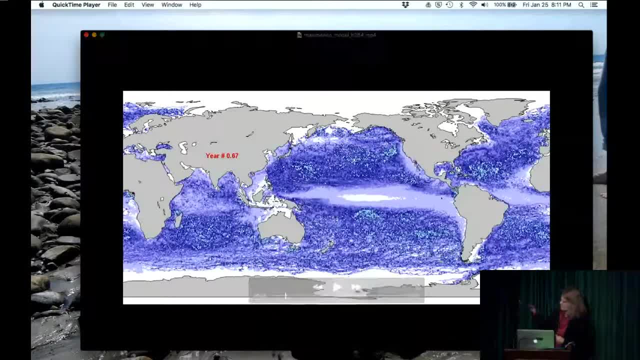 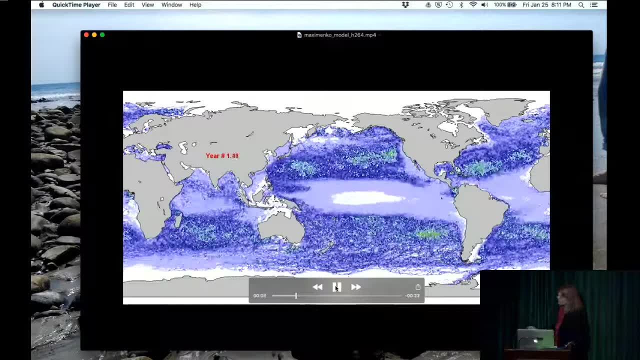 ocean, basically evenly covered in fake plastic debris. So that's what these purple specks are. I'm going to turn on the ocean currents and you can see what happens. So you can see at the equator, here, right in the middle of the image, it's becoming white because the material is moving. 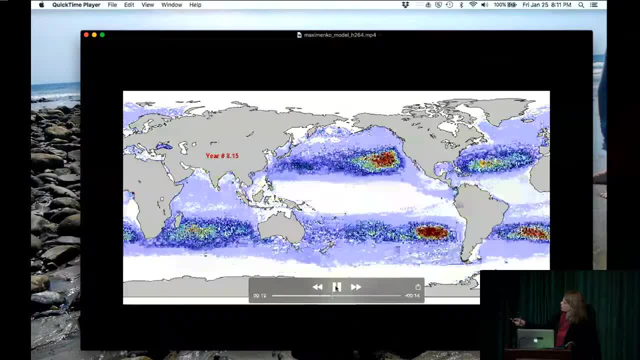 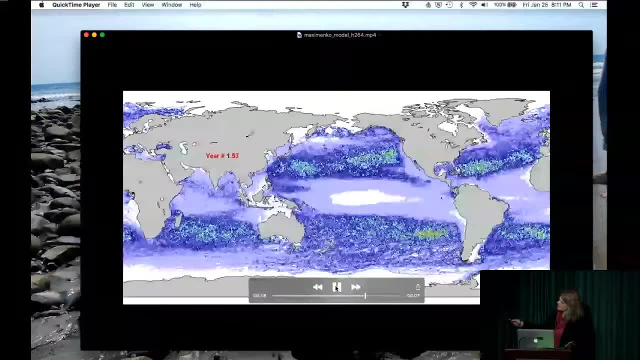 away, Whereas in these regions, in the subtropics, they're getting darker and darker and accumulating this debris, And these are the subtropical ocean gyres. So ocean physics happens in such a way that there are these gyres that circulate around the large ocean basins And at these latitudes in 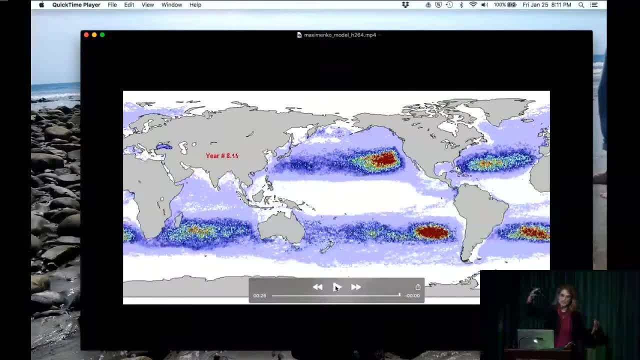 both the northern hemisphere and southern hemisphere, the currents kind of slow down and converge. It's kind of like an oceanographic dead end, And so that's what's causing these floating, passively drifting materials like plastics to accumulate here. So this is great. 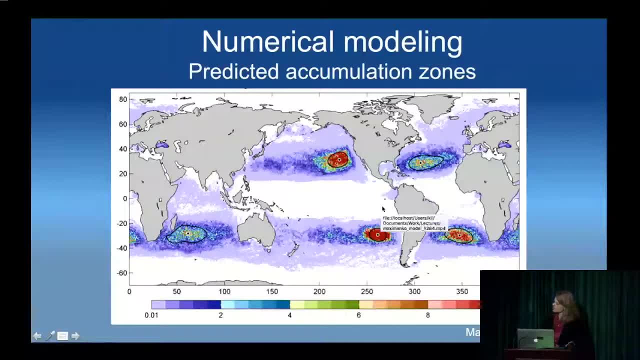 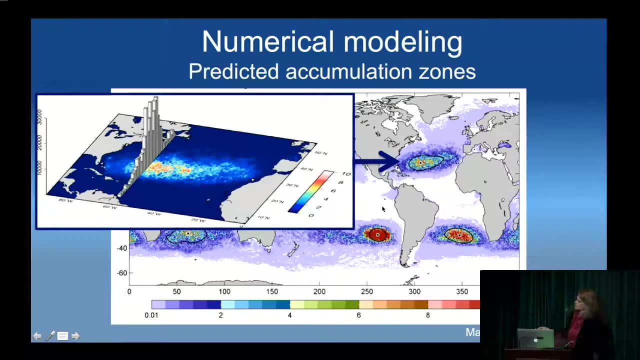 and really exciting to see. But then this is also going to show you now the utility of the plastics data that we've been collecting for decades, because we can now look at the plastics that we've collected in the real ocean and overlay that on the model predictions. 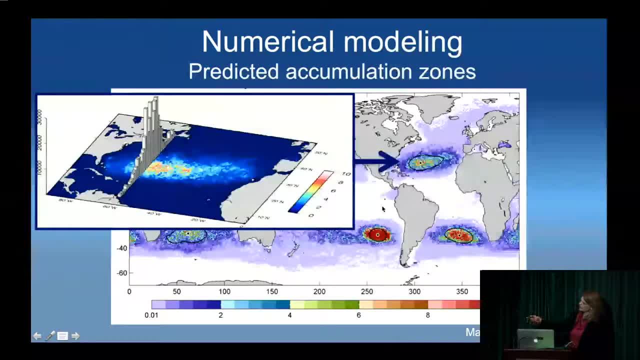 So the data that we're appreciating here is basically taking this North Atlantic patch and putting it on the ground, And then these bars are showing you the concentration that we collected in our net toes And you can see there's a really strong correspondence there. So not only is there, 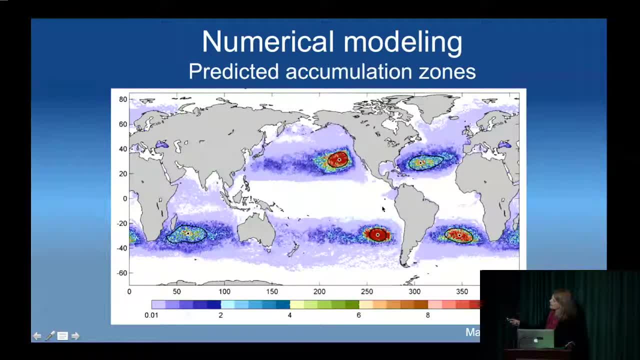 a garbage patch in the Pacific, an accumulation zone, as I like to call it, and one in the North Atlantic. this model predicts that you would find them also in the southern hemisphere gyres And in these regions there are very few ocean data. There have been sort of single cruises that 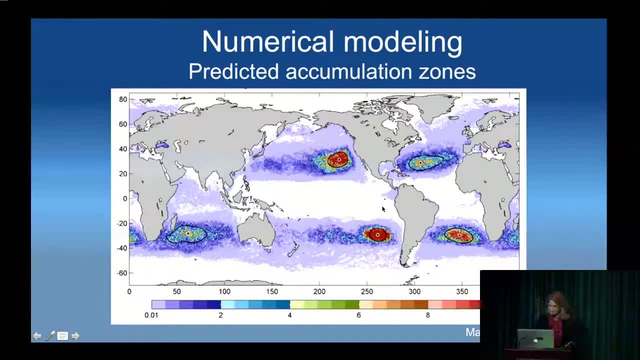 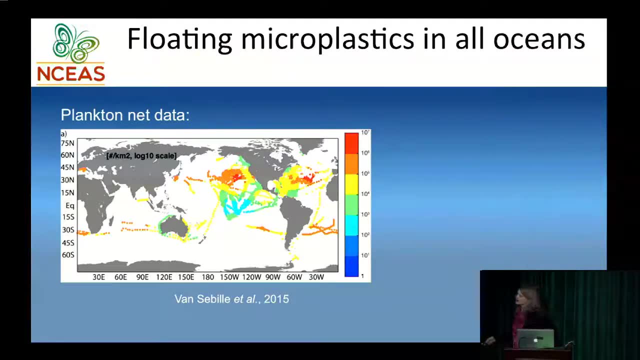 yes, in fact, there are plastics accumulating in these regions as well. Okay, so back to the high level question of how much plastic is in the ocean from ocean data. We did a study collecting all of the plankton net data that exists or that existed as of 2015.. 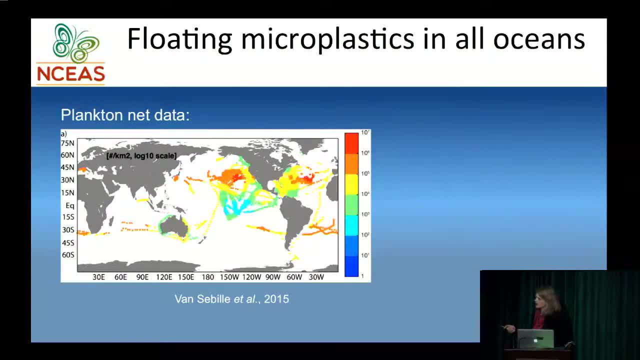 And this is now a global map And again each dot is a plankton net toe And you can see the SEA data sets here in dense concentrations in the North Atlantic and in the Eastern Pacific, And here are those singular cruises I mentioned in the south, the southern hemisphere. So you can see there does. 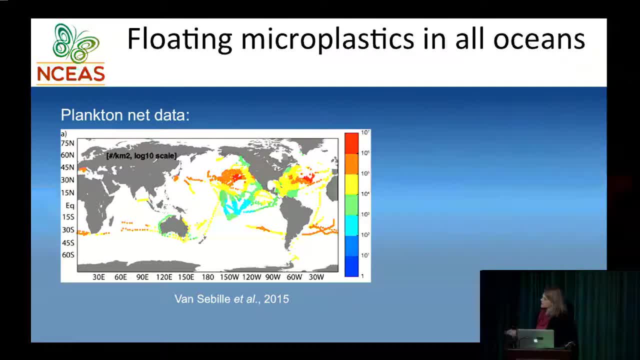 seem to be accumulations in these regions And it's color shaded according to concentration. So you can see that. But what you can see is if you wanted to make a global average, you certainly could average all these numbers and come up with something. But the vast majority of the global 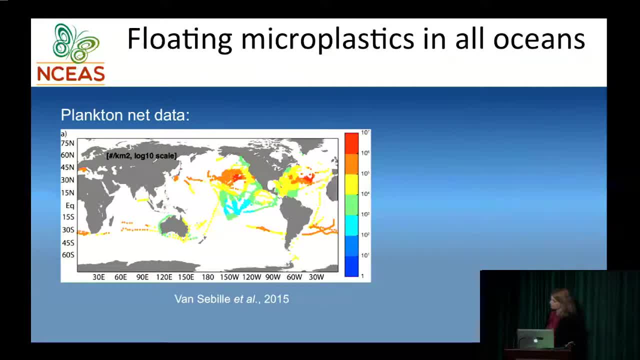 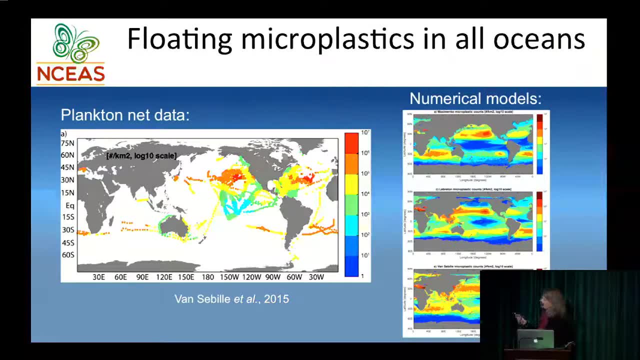 ocean has not been sampled for ocean plastics, So it wouldn't be a very meaningful number. So in order to be able to make a global estimate of floating microplastics, we turn to these numerical models. So these are three models. We don't have to go through the. 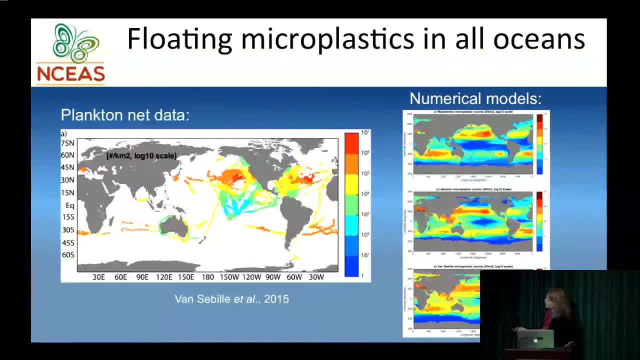 details. This top one is the one I just showed you. There are two other flavors that are pretty independent, the way that they were constructed, And in all three of these you can see these high concentrations. The reds are happening at 30 degrees north and south. 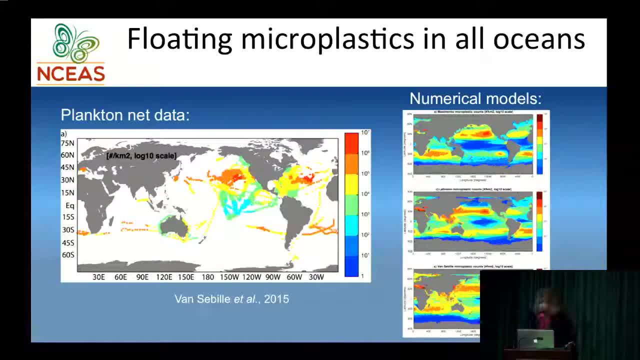 But obviously there's great variety in the details of these models, And when you actually put these together and add up all the floating microplastics, we come up with a range of between 93,000 and 236,000 metric tons. Okay, So that's a big number, right. 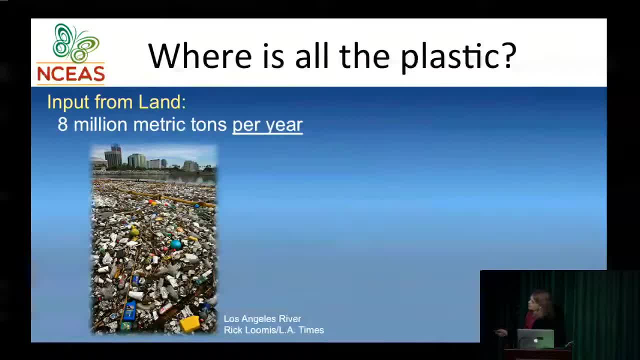 Well, let's go back and compare that to our estimate of input from land. So this is a picture of the Los Angeles River after a rainstorm. This is a big boom that was used to collect the trash that was washing out. All of this had been sitting on. 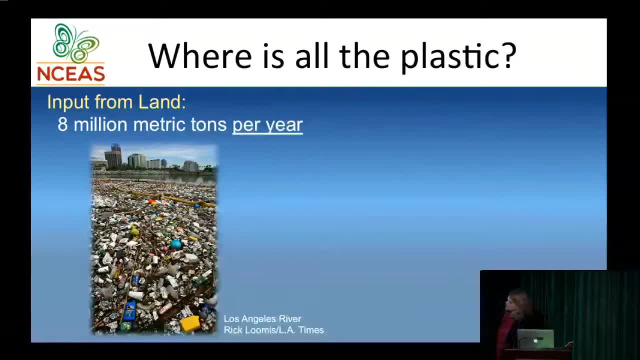 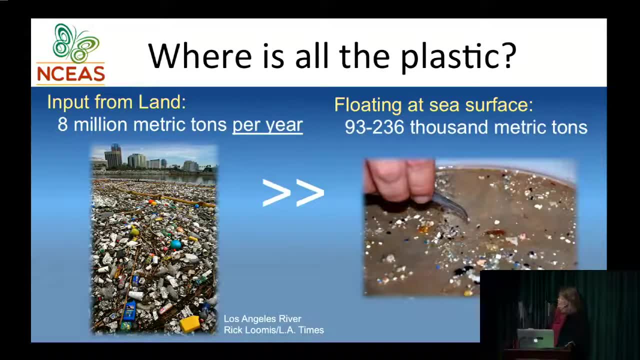 dry land until there was this big rain event. So we're talking about plastic waste from land. The estimate, to remind you, was 8 million metric tons per year And now what we've estimated from ocean data floating at the sea surface is basically 1% of that. You know we're talking. 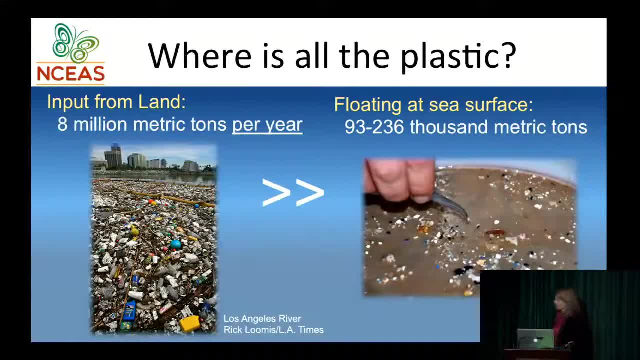 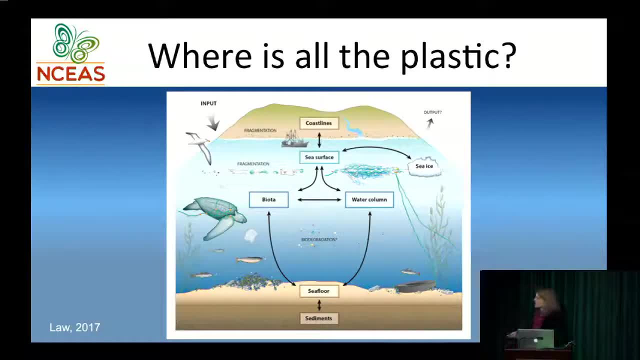 1,000 metric tons instead of 8 million tons per year. So this has raised a big question in the community: Where is all the plastic? This is a cartoon that's just meant to illustrate where it could be. So if you this is kind of, think about the big white box as the Marine. 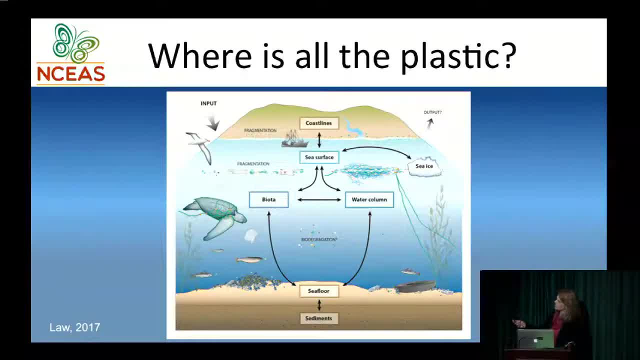 environment. So we've got coastlines which are beaches, but rocky shorelines and estuaries and wetlands. Here's the sea surface where we tow our nets. Here's the sea ice, where I mentioned there's been evidence of microplastics. Here's the water column where we have lots of biome and we're so. 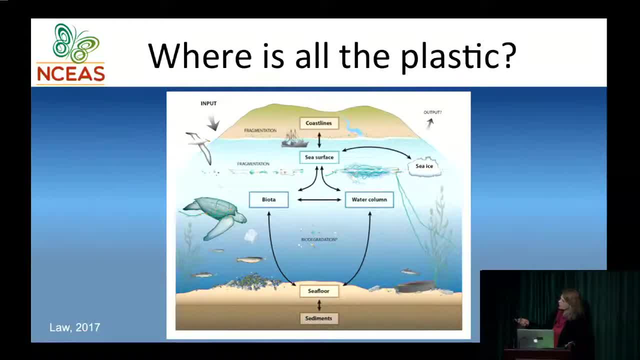 biota and the seafloor, including the sediments. So each of these boxes represents what I refer to as reservoirs where plastic debris could be residing. So we have a number for the little stuff in the sea surface box, but we really don't have any numbers for any of these other reservoirs. 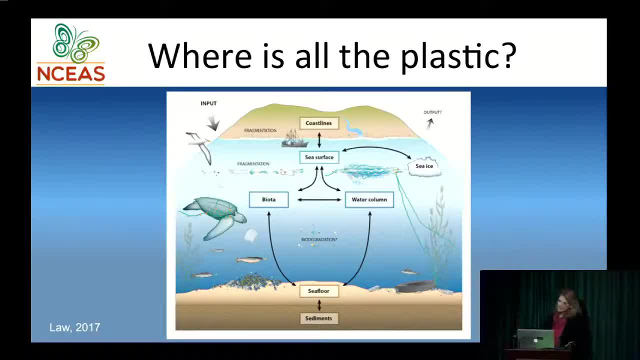 And we certainly know that there is plastic debris in all of these places. but we don't know which one of these boxes has the most, because it's very hard to sample the ocean As hard as it is to go out in the middle of the ocean and tow plankton nets. it's a lot harder to get seafloor images. 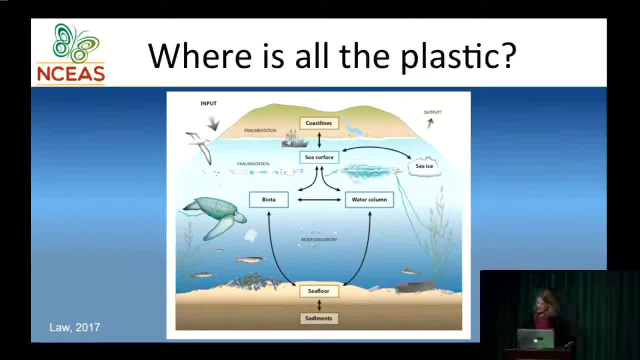 or samples, or to set sample sediments. So this is, I would say, a very big, open question right now And, of course, until you know where the debris is and what kind of debris it is- whether it's microplastics or big items or entangling items- it makes it hard to know what the impacts are. 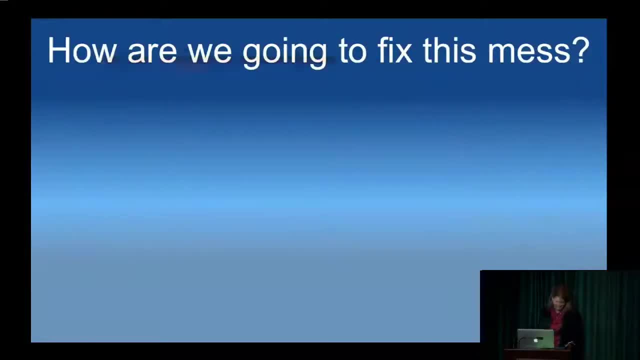 or how to clean it up. Cleaning it up: How are we going to fix this mess? Well, the bad news is there is no silver bullet, So get rid of that. How we're going to fix this mess? it's going to. 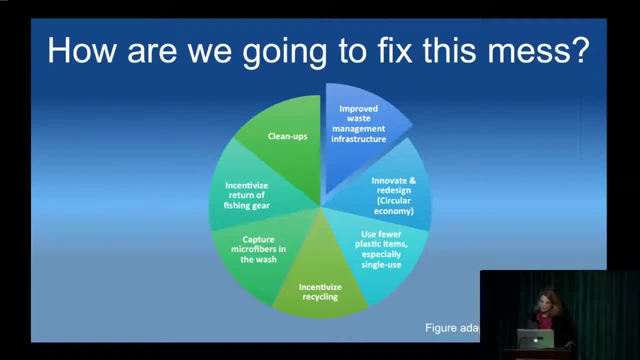 require a variety of interventions, So this is just sort of showing this wedge approach. The one that's offset here is improved waste management infrastructure, And in my opinion that is the top priority right now. We know that there's tremendous amount of waste in the environment that's not being captured, and 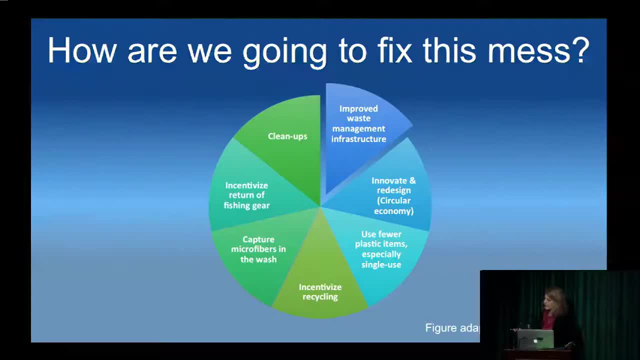 treated in waste management, So let's turn off the tap there as a first priority. Moving around, it is also important to do cleanups, And cleanups, in my opinion, are most effective if you're going to move slightly offshore, because that's where we think most of this material is. 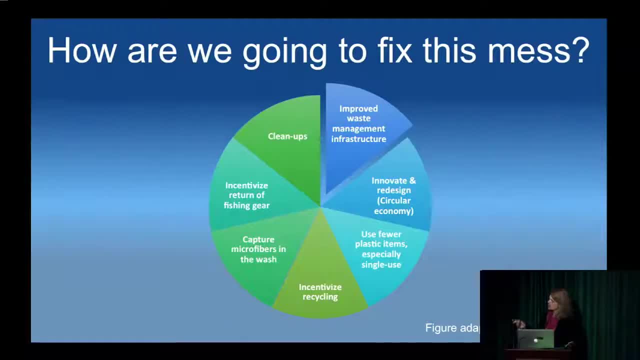 coming from, So this is sort of the last chance. There's a last chance capture in here where you can maybe get it or clean it up before it ends up as microplastic thousands of miles offshore. There are other things like incentivizing return of fishing gear, because we know 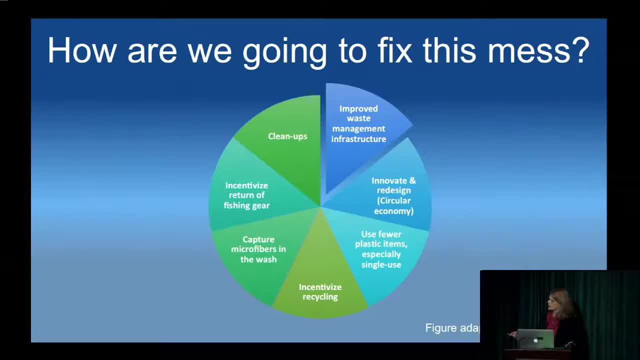 the entanglement risks of fishing gear, The microfibers I mentioned. we could put filters on our washing machines, Incentivize recycling so that maybe some of this waste that might be lost because people don't really care about it might be worth it. So we're going to have to. 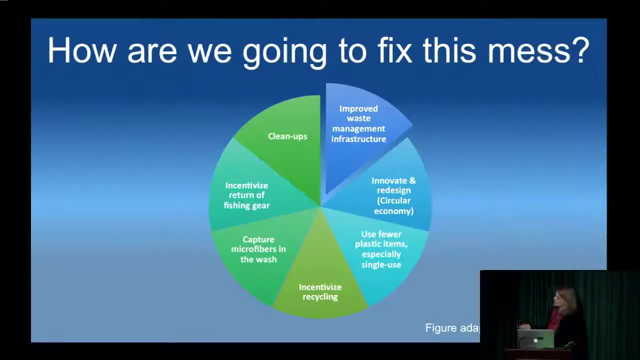 work with something and be captured and collected. But I think in the long term, we really have to move to this part of the figure And thinking about really, how are we using these materials? Plastics are invaluable. They were developed for a reason. It's a tremendous engineering. 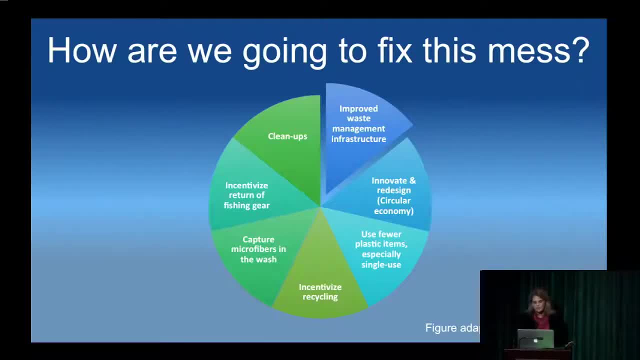 success. We all rely upon them, But are we using them in the best possible way? And when we do use them, do we have a thought about what we're going to do with them when we're done? So this is where we start getting into innovations, thinking about how we use these. 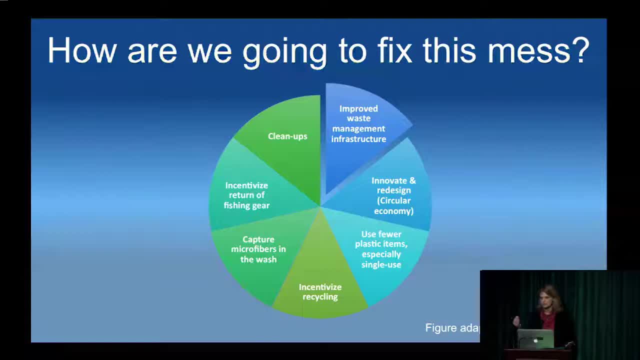 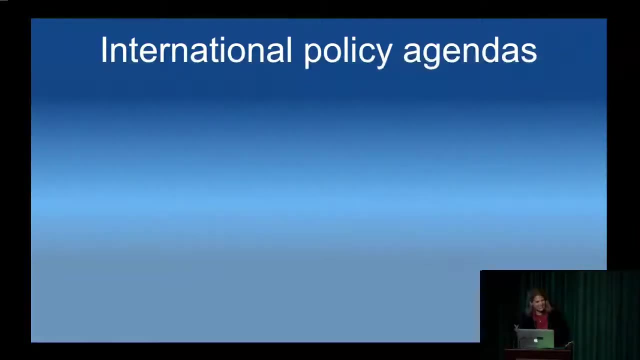 materials, trying to think about full life cycles and recapturing the materials to make sure that they have value and end up being reused, minimizing waste and minimizing what can be lost to the environment. So the fact that this many of you have turned out is a good indication of how much publicity 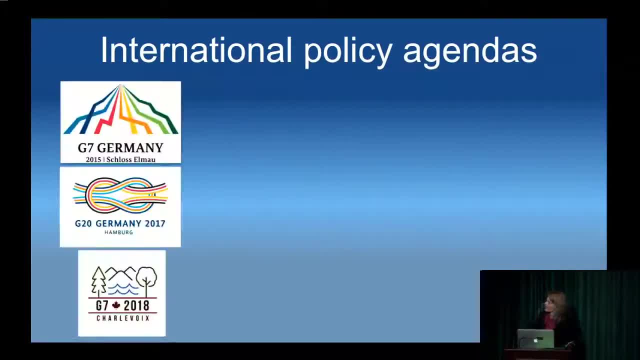 and public attention there has been to this topic And this has also caused it to reach really international policy agendas. So I had the opportunity to participate in discussions led by Germany when they had the presidencies of the G7 and G20. And they put this on the 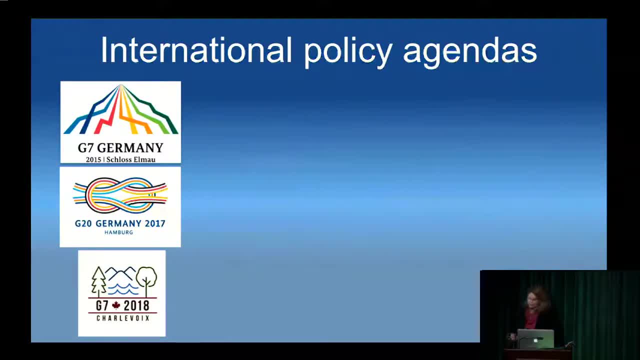 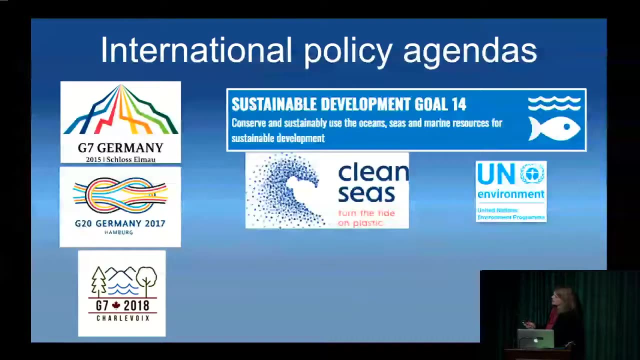 top of their agenda, Creating marine litter action plans, And then Canada followed up. Japan also engaged on this during their presidencies. So these groups are engaging on marine litter as a major global problem. The UN, in a variety of capacities, has programs around trying to. 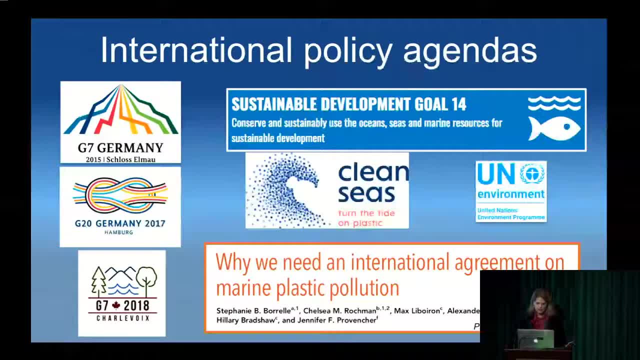 solve the problem, bring attention to it, understand the science better. And then a group of academics have even argued that we should have an international agreement on marine plastic pollution, something akin to the Paris Agreement. So there are a number of ways that we can do this. 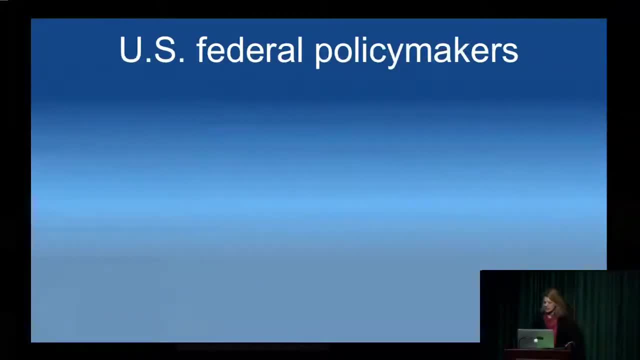 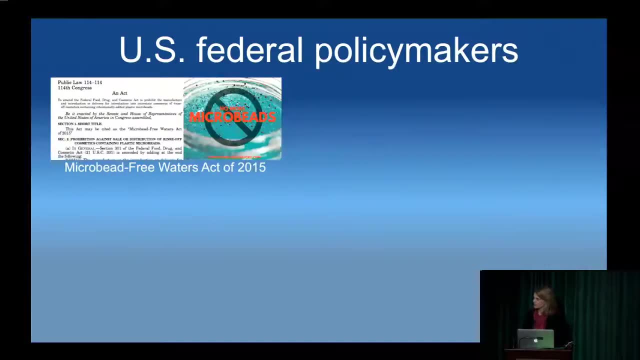 So this is being discussed at very high levels. What about in the United States? Well, the United States actually passed the Micro-Bead-Free Waters Act of 2015 under President Obama. It was bipartisan legislation that passed without any kind of contention. These plastic microbeads are no longer allowed to be used. 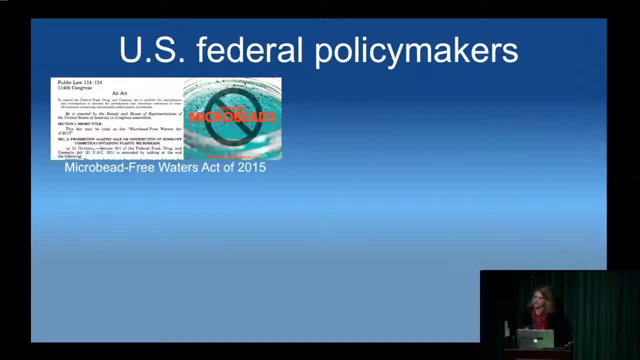 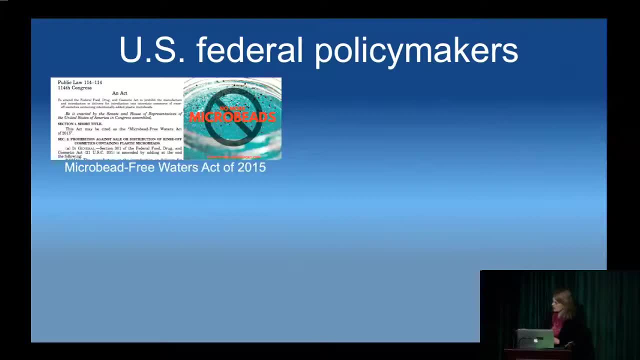 treatment plant may not capture it before it goes out into the environment, So this piece of legislation was intended to tackle what is a known problem. John Kerry held our first ROCian conference in 2016.. And marine debris was a featured topic there. 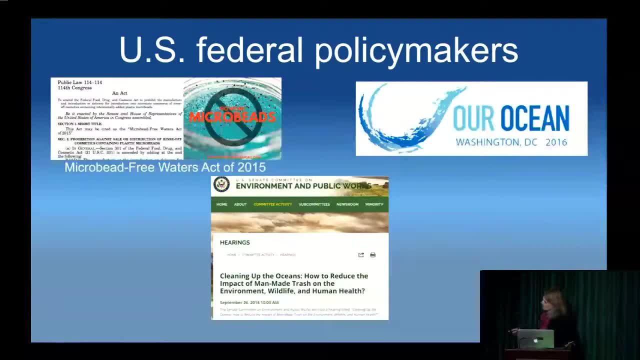 And then, most recently in last September, the Senate Committee on Environment and Public Works held a hearing, on which I was fortunate to testify, on cleaning up the oceans, And we could talk about. there's a lot of interesting things that came out of that, But for me, one of the big takeaways is that 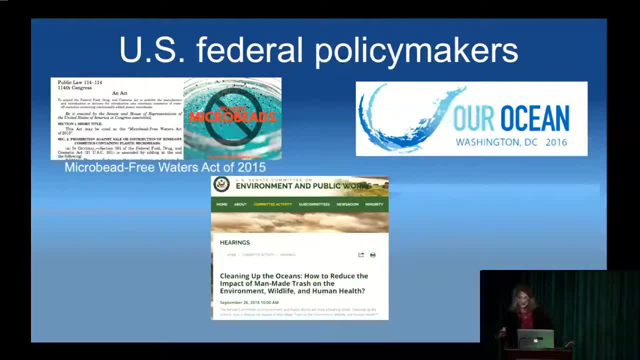 the discussion was not whether or not this was a problem. The starting point of the discussion was: this is a problem, What are we going to do to fix it? So there are good indications. And then, shortly after this, hearing Congress again bipartisan piece of legislation was the Save Our Seas Act. 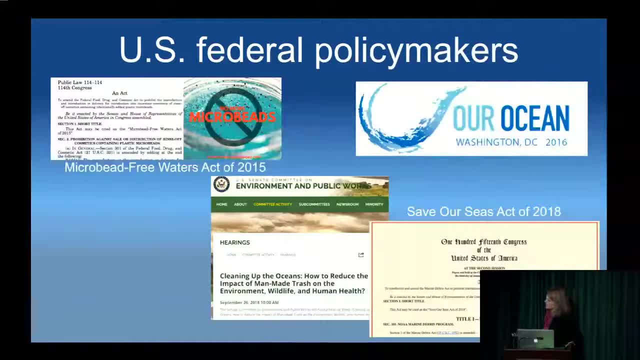 of 2018, which, mainly, the outcome was to reauthorize the Marine Debris Act, which allows the NOAA Marine Debris Program to continue existing. It's not all good news, though. As I mentioned, Canada and the G7 did come up with this ocean plastics charter, but unfortunately, the US 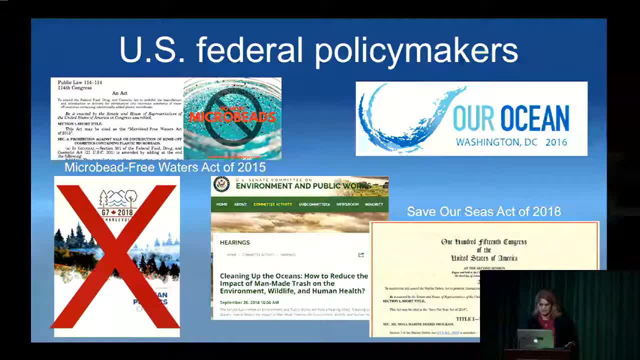 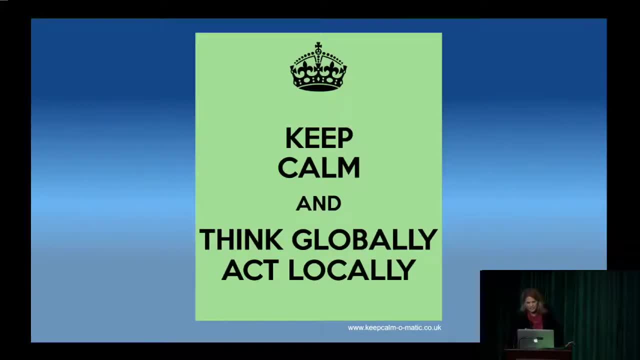 was refused to sign it. So the US and Japan didn't sign this charter. So there's work to be done. Well, that's great, but what are we going to do? We don't have to wait for the US government. 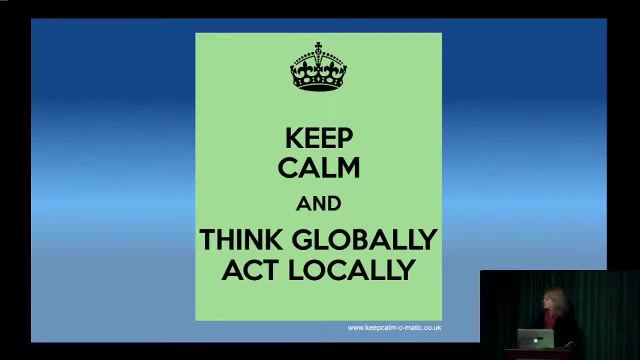 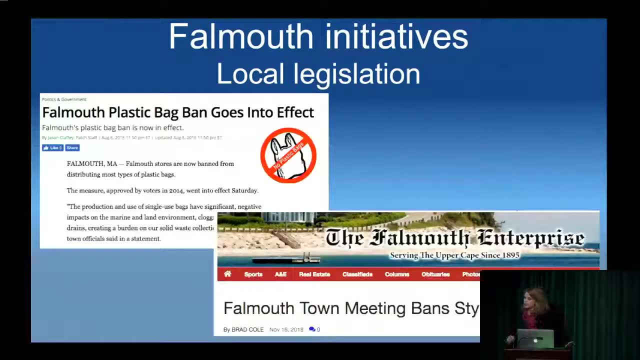 or for these high-level policy groups to do something. So, like many things, let's just think about what we can do locally, And this is where Falmouth is really, I think, leading in many ways. So you probably know that there's been local legislation passed. Plastic bags are banned from many stores approved in. 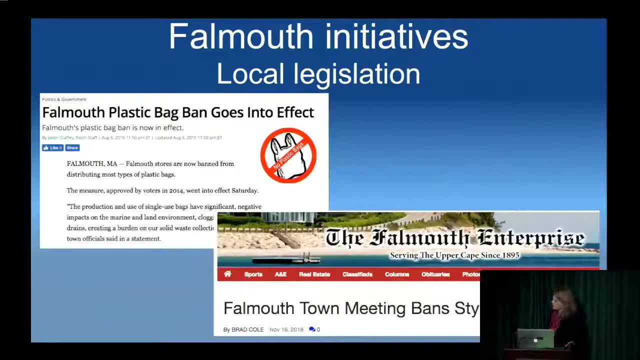 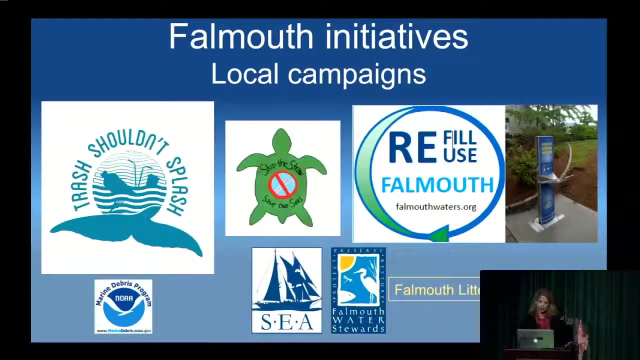 2014,, so quite a few years ago, And more recently, polystyrene foam has been banned. I think that's now in a phase-out place. It was passed just this past November. So local legislation can have an impact, especially when it's targeted to things that maybe have no negative impacts, or maybe 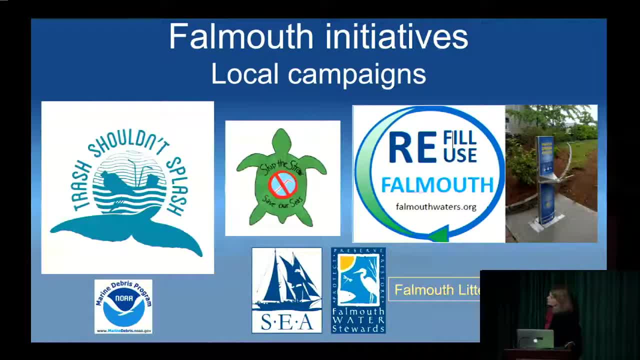 they're easily replaced. And then there are also a lot of local campaigns going on. So SEA, together with Falmouth Water Stewards, wrote a grant proposal to NOAA's Marine Debris Program to conduct a behavior change, a sort of local public education campaign about reducing use of single-use plastics, where we can. 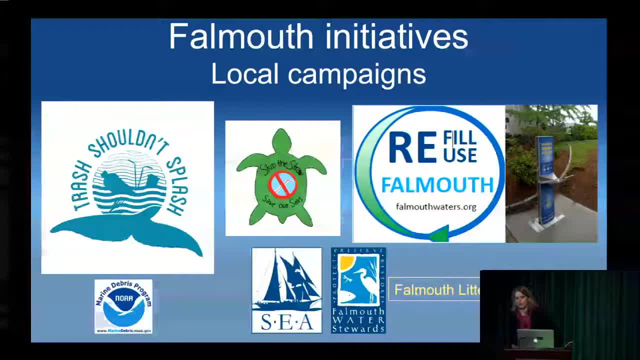 And so we've named that the Trash and Splash Campaign. We've worked with all of the local Woods Hole restaurants- You'll see signage in there saying do you really need that straw- Trying to help them figure out how to reduce the use of single-use plastics where we can. 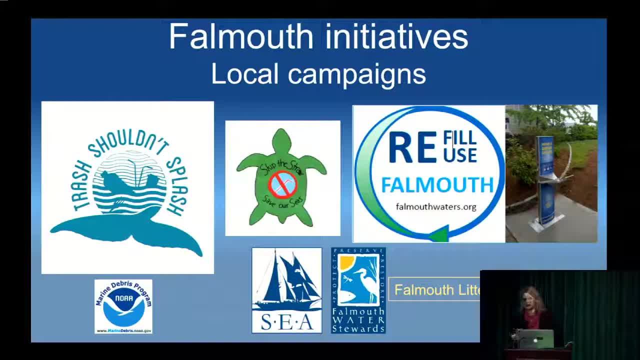 How to phase out single-use plastics where possible And, at the same time, educate the consumers- the customers that are coming into those businesses, so that they don't have blowback and angry people who just want their straw. So a lot of what we really promoted was things like: 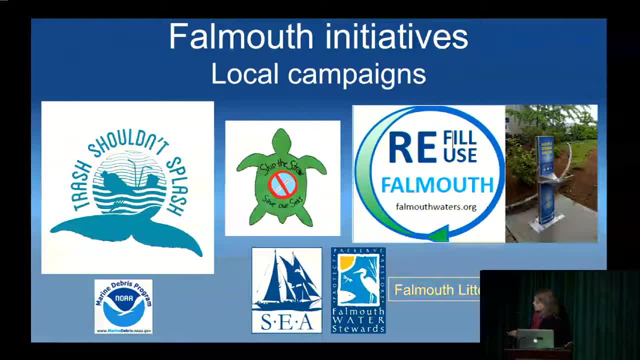 straw upon request. Don't give people a plastic straw unless they ask for one. And then we've also been working in K-12 schools, And a big part of that project was through the Falmouth Water. Stewards was a group of middle school girls who I think are about to be high school girls now. 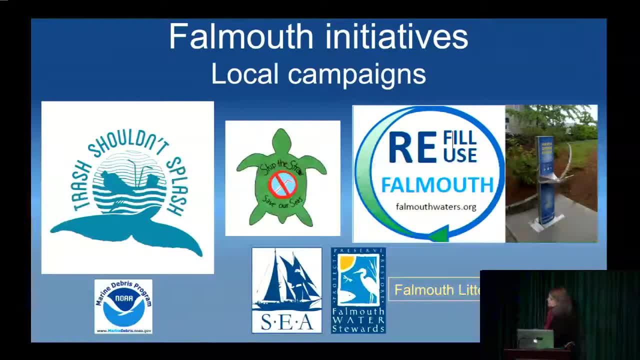 coming up, They started to skip the straw And so we've been working with them for a long time, So we've used the straw program in town. So you'll see this partnership. And then, if anybody knows Alan Robinson, he moved to town like ten minutes ago And he's 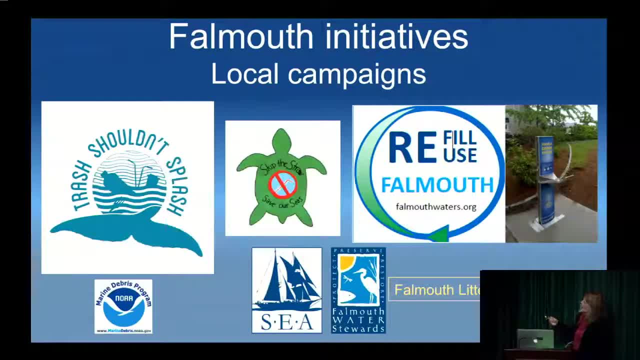 already got funding for eight refill refouled Falmouth water refill stations. So this is actually the first one that's off of Main Street here by the public restrooms. So these are, those are piped into Falmouth water. You can bring your own to fill up your poder at. a Memory where one of the town's down at the base of the poultry shoal And he was standing there and trying to figure out how to fix it. He's obviously a little clueless, so I think he's not willing to make the point about x and y, but hoping to get the transfer. 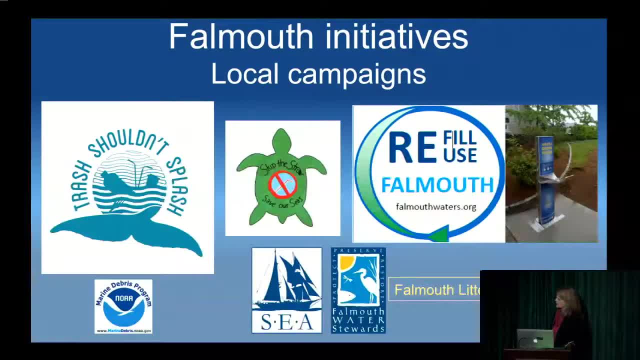 here. I'm more than glad to continue to help him out as he gets the job done with this Falmouth Water reducing single-use water bottle use, And he's very recently, with a number of other people, started a Falmouth Litter Reduction Team. So there's a lot going on locally, lots of 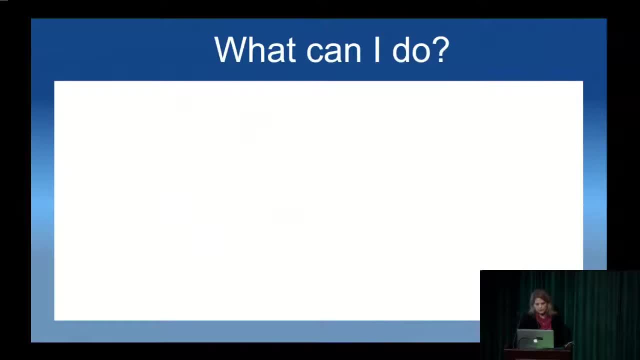 ways to engage. What can I do, Even if you don't want to get engaged with big groups? I think, first and foremost, if we all make less waste, there's less that we need to deal with. So this is really just the waste management hierarchy. This is not new right. Use less, Reuse, So. 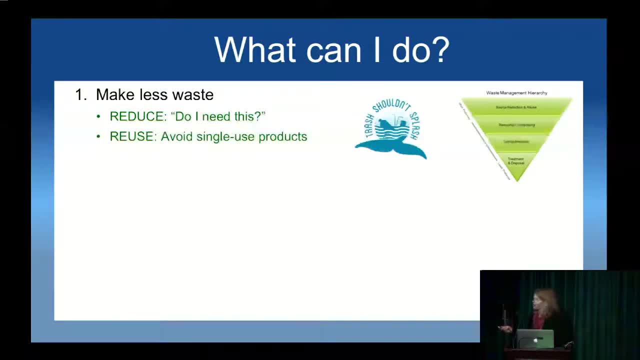 bring your reusable water bottle and coffee mug and produce bags and straws and utensils and that will allow you to avoid those single-use products. So that's really kind of the focus of our Trash and Splash campaign. Recycle what you can, of course, And then some people may want to. 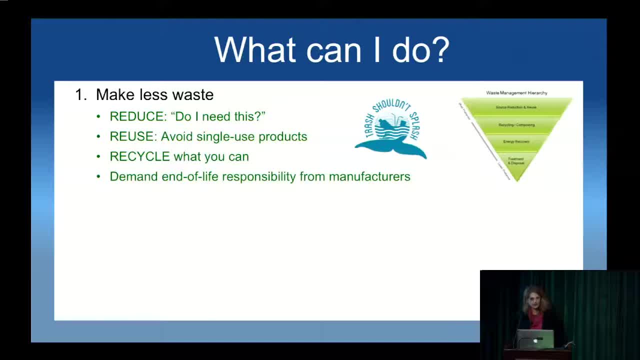 engage in conversations with manufacturers of products and say: you know you gave us this package. You should help us figure out what to do with it. So that's under the umbrella of extended producer responsibility, which is actually a lot of work. So I think that's a lot of work. 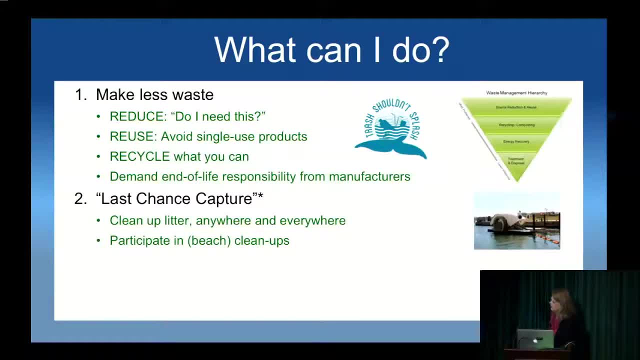 It's actually been legislated in Europe, but it's much harder to do here. Then there are things like last chance captures. So this is actually Mr Trash Wheel. He was built in Baltimore by a man named John Kellett, whose son is actually a current C-semester student, So we had him on a panel today. 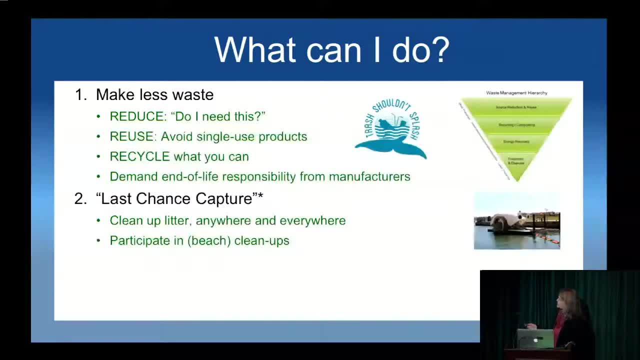 speaking to the class and I learned a lot of the history of Mr Trash Wheel, who's an extremely charismatic solar and hydro-powered water wheel that simply collects trash that comes down the Jones Falls River in Baltimore, goes up this ramp and falls into a dumpster, So it gets a lot of. 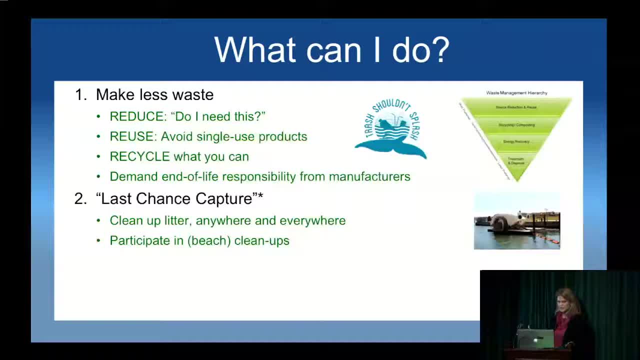 collected and towed away and properly disposed of before it goes into the ocean. And Mr Trash Wheel has a Twitter feed. and Mr Trash Wheel has two friends, Professor Trash Wheel and Captain Trash Wheel, who all have distinct personalities. Really an internet sensation, a great success story. I 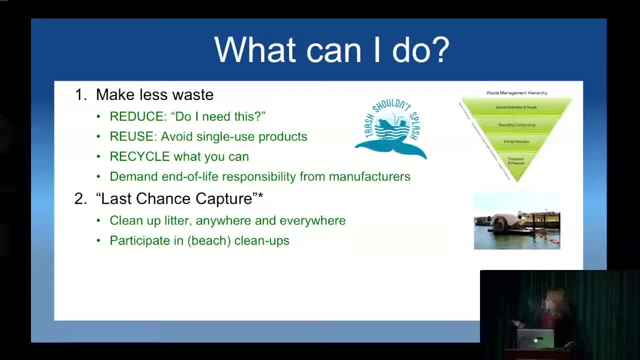 highly encourage you to Google Mr Trash Wheel. So this is a really effective way you know. and he just would walk by Baltimore Harbor every day, he said, and would hear tourists saying ugh, the harbor is so disgusting. And he would watch this trash flow out after a rainstorm. 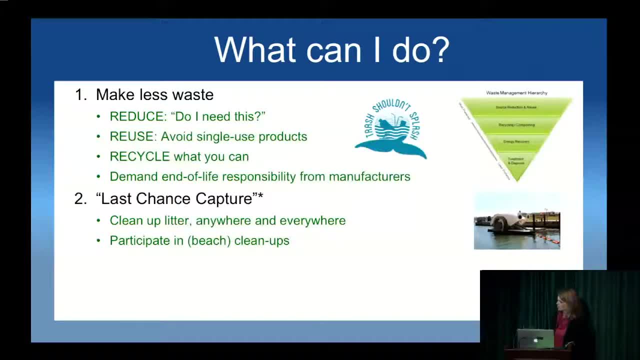 and just decided I'm going to do something about it. So this is a real success story. But broadly, cleaning up litter anywhere and everywhere, and that's what this Found This Litter initiative is thinking about, especially in beach cleanups, because we know those, of course, are. 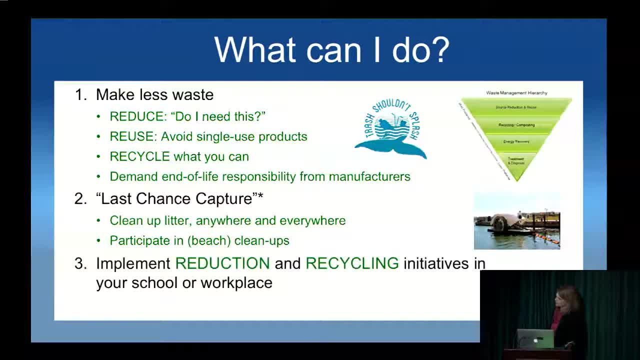 right on the ocean And you know this is like tell your friends and family. there are things you can do in your own business or in your own school- reduction and recycling initiatives, And I really encourage folks to engage with the local government and the public works department, because that's. 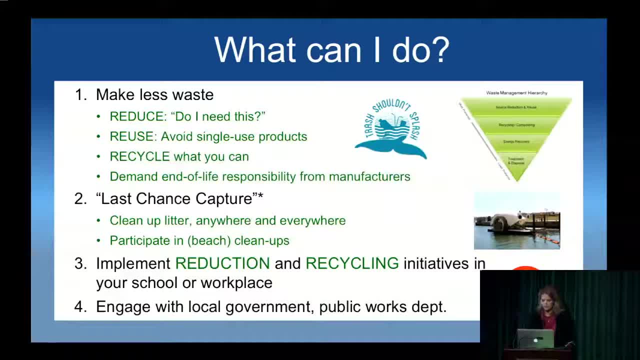 how some of these things really come to be is working with the town officials who know how things operate and know what the barriers are, So just engaging your community in any way that you can, or just at your household level with your friends or your family. So with that, I just want to end with a massive acknowledgement slide. 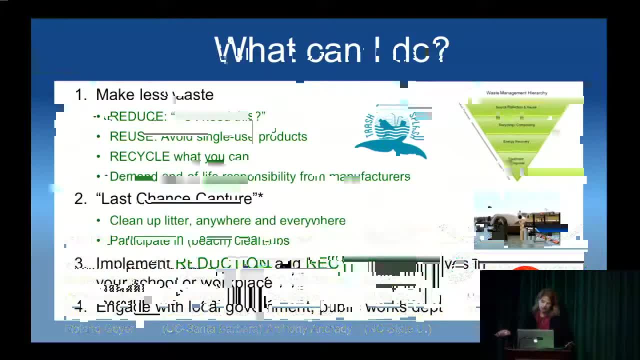 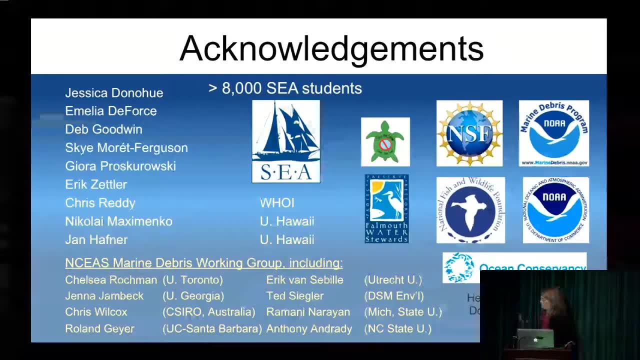 First and foremost, none of this would be possible without the more than 8,000 C-semester students that have been going to sea and collecting plastics for decades, And I wouldn't be here if not for them. And then there are many SEA collaborators- This is a small fraction- who've 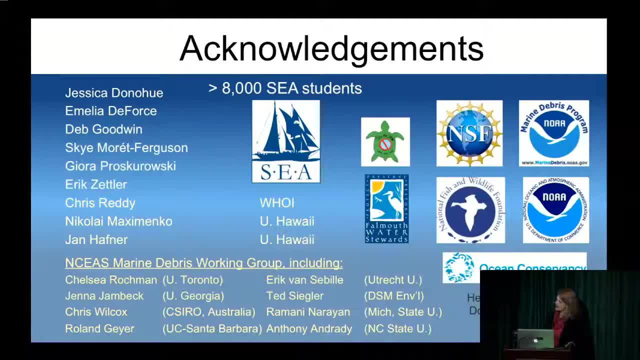 contributed to this work over the decades. Chris Reddy deserves a special call out because he's at Woods Oceanographic. He really pushed us and said: you need to get that data out there. Nobody knows what you're doing, So he was really a big impetus in getting our first paper published, as well as collaborators at University of Hawaii. 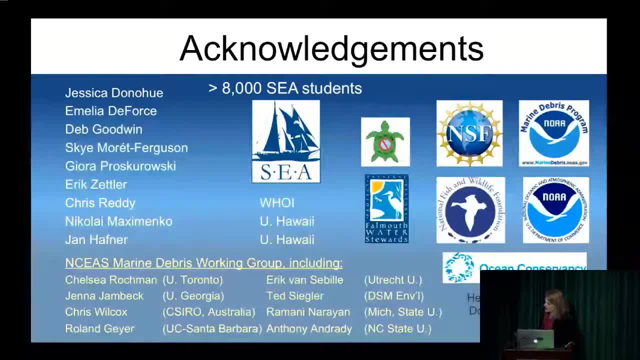 And then some of that high-level estimation work- about 8 million metric tons and 8.2 billion tons- that came out of a working group, out of the National Center for Ecological Analysis and Synthesis. So these are some of my colleagues in that working group. 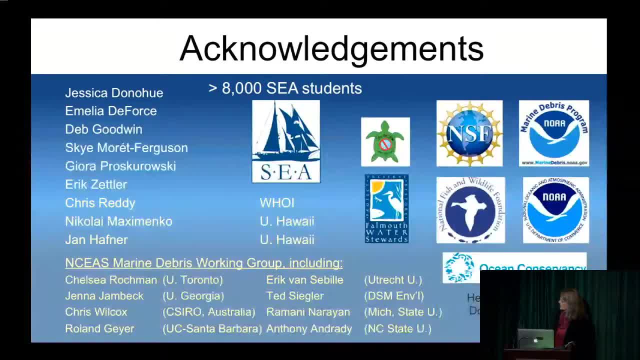 And then support from federal agencies, but also the Ocean Conservancy And the Doherty Foundation. So with that I would like to say thank you. Questions, Terrific talk. Thank you very much. Most of your solution ideas were on the supply side. You made one mention on the- it should be the demand side, but one mention on the supply side about- and you said that it was really hard to deal with- the manufacturing side. Can you say a little bit more about that side of it please? 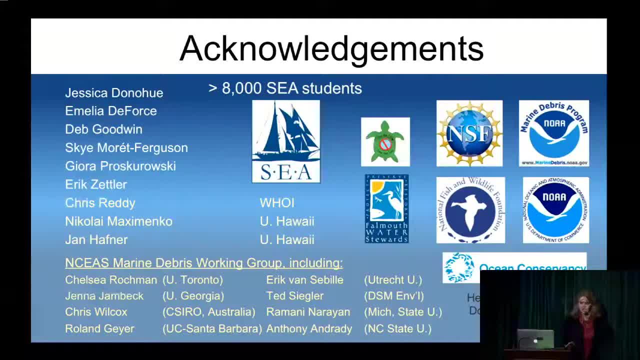 Yes, thank you for asking that, because that was actually not my answer. Okay, That was my intention and I should have. it occurs to me now that I should have put one other bullet on there, Part of. I've been fortunate to work with a group called the Trash Feces Alliance, which was put together by the Ocean Conservancy at the same time that they supported this working group to advance the science. 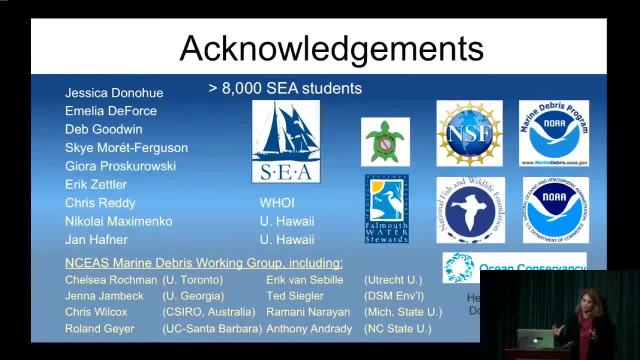 And the group is actually the membership is largely big corporations who either make plastics or make plastic products or use plastic products. I mean, we're talking about Dow Chemical, we're talking about Coca-Cola, you know big companies, And those are in the same room with NGOs. and I serve as one of a few science advisors to sort of keep the conversation honest. 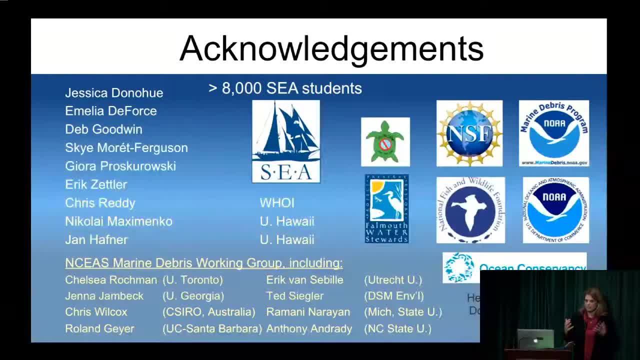 And they are looking to find common ground where they can affect solutions, And so that group, after we estimated this huge input of plastic waste from land, has decided to invest in waste management in Southeast Asia, And how that's actually going to be realized remains to be seen. 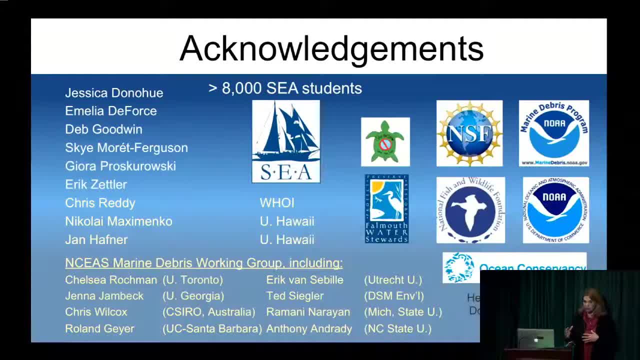 There's huge money. I think they know that this is a problem. They don't want their products out there. There's been brand shaming. There are lots of people who are really trying to attack them And I think they're trying to take the high road and act where they will. 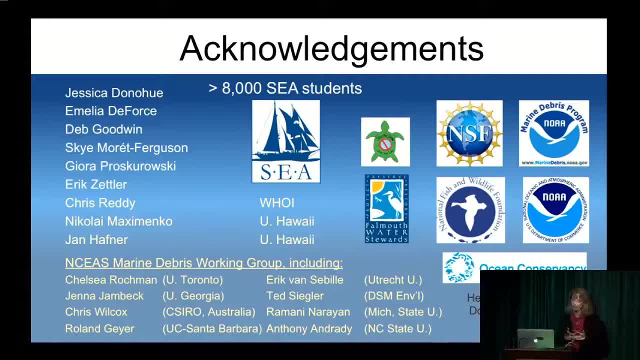 Now they're not going to stop making plastic, and I don't think we can reasonably ask them to do that- So they're going to put money towards waste management. But also there was just an initiative announced in Davos two days ago. 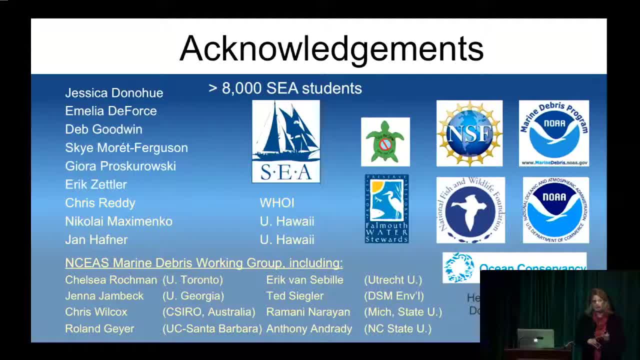 A group of these- I think it's Unilever and PepsiCo, Procter & Gamble- are now trying to start a reusable container system, sort of basically reinventing the milkman. I don't know what the feasibility of this actually is. 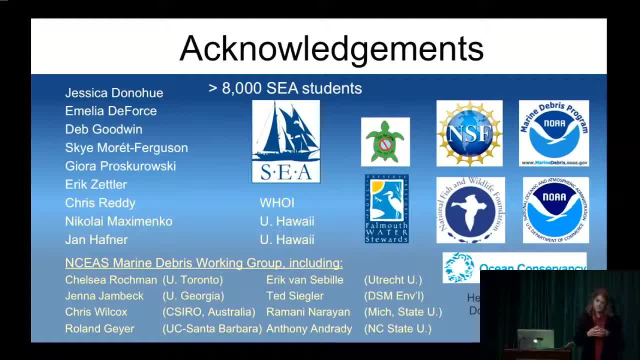 They are creating like stainless steel Haagen-Dazs containers and you buy it and then somebody picks it up and cleans it and brings it back. They're engaging. But you're absolutely right, We are consumers and we have power and I think that's why they're engaging. 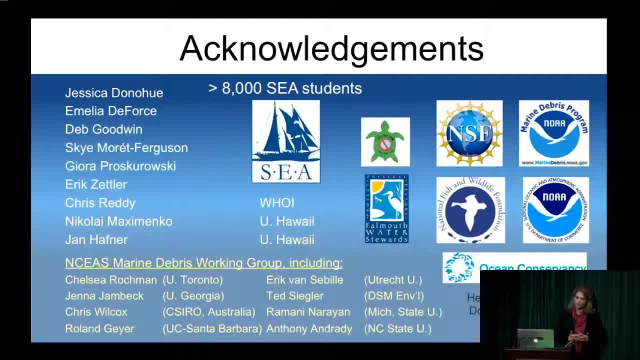 So you know, as part of a suite of solutions, you're going to see more from them. They may not be doing everything, and they're probably not going to stop making plastic. They may not be doing everything and they're probably not going to stop making plastic. 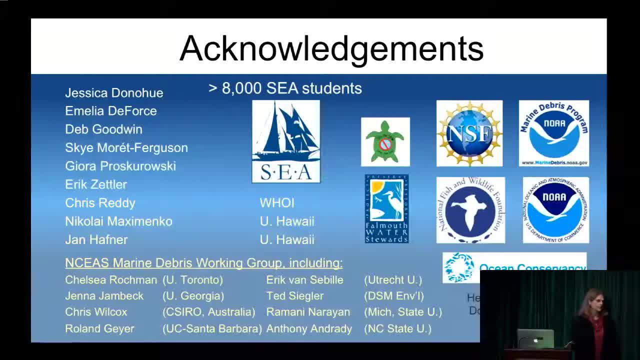 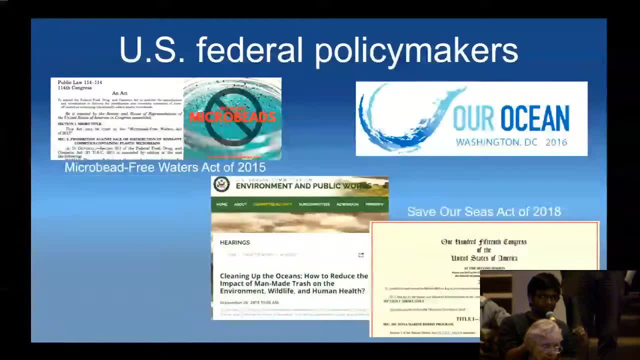 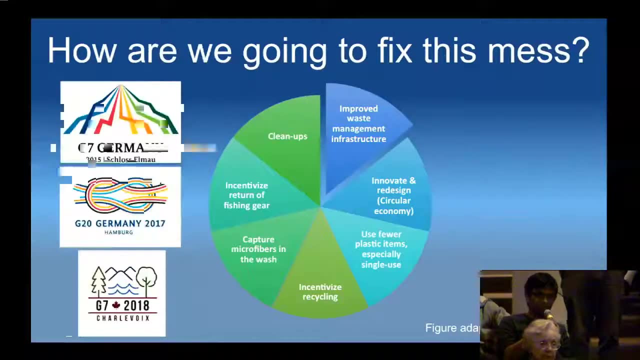 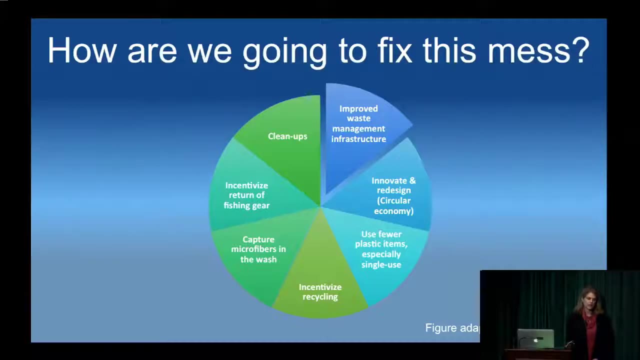 On the same topic of the pie chart that you had displayed, do you think there's a space for biomedic or replacement materials, kind of like bio-inspired plastics or other biodegradable type materials? Yeah, biodegradable plastics or compostable plastics are challenging. 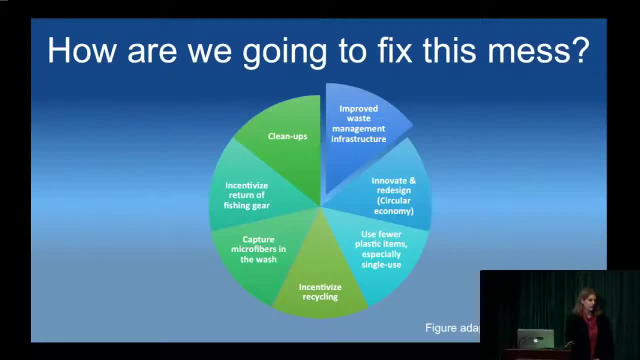 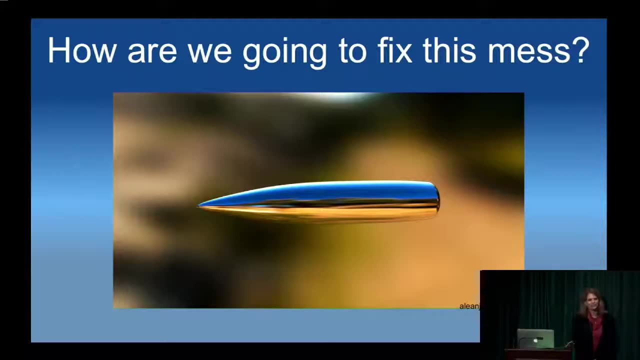 Yes, maybe I think there could be places for that. So let's remember the slide that came before that. So there are definitely folks who just say, well, let's just make it all biodegradable, We can throw it out our car window and it'll disappear. 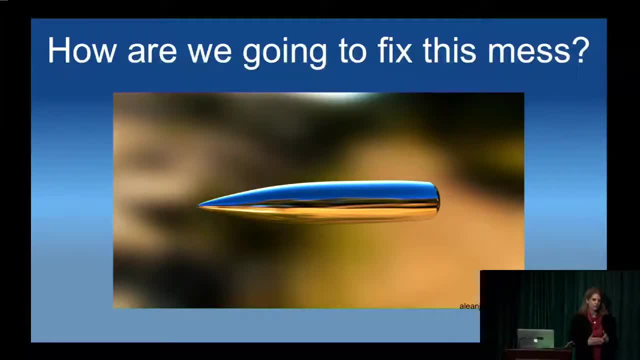 Well, you don't want people to think that biodegradable means do whatever. There are materials that exist that are biobased. Okay, Biobased doesn't necessarily mean that it will break down either in nature or in a composting facility. 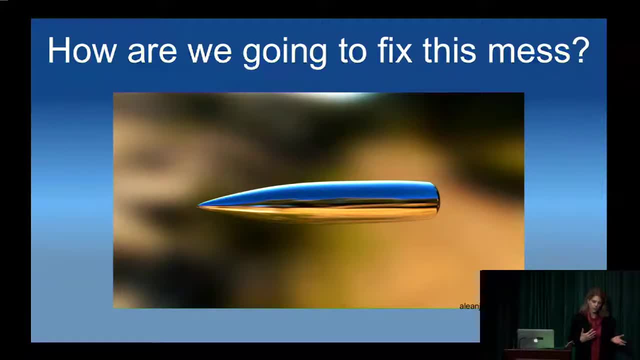 So you have to be very careful about what materials you're talking about. So even if it's made out of corn, it doesn't mean it's going to disintegrate. But there are some materials that will biodegrade, but they biodegrade in an industrial composting facility. 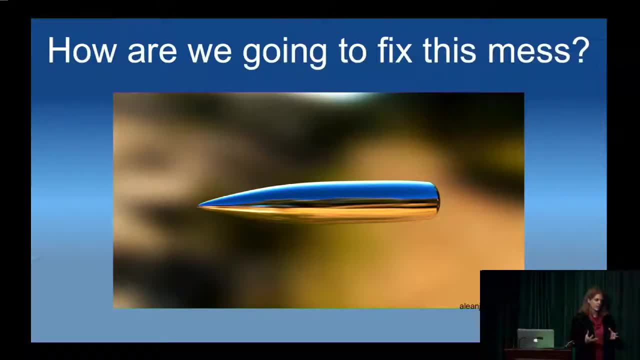 And lots of- in fact we found that a lot of the Woods Hole restaurants. we didn't come in and tell them about this new problem that they'd never heard of, right? So they were already taking some measures and a lot of them said, oh well, we're using greenware. 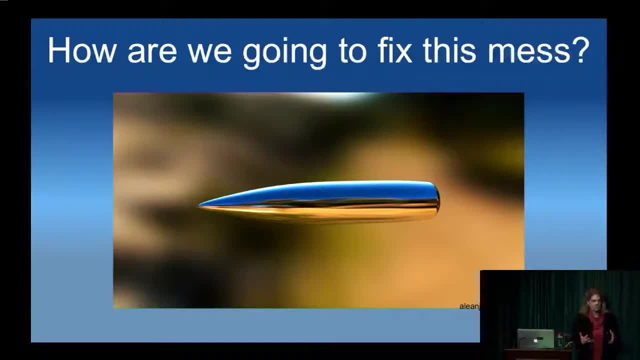 And that's great. But if you have a place for that greenware to go, where it's going to end up in an industrial composting facility, and if you don't, then it means it's going to go into the regular trash can. 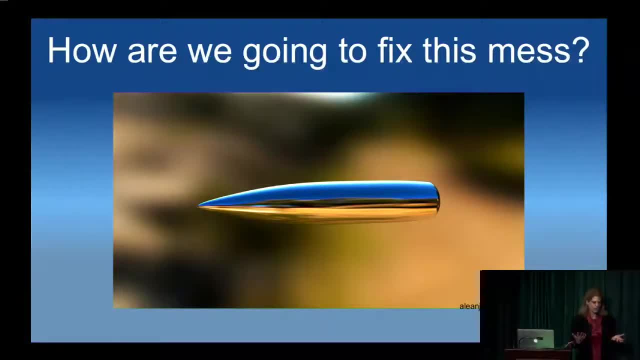 And if it's lost into the ocean, it's just as much of a hazard. So I think we have to be careful and also remember that the properties of plastic that make it so useful and versatile are things like durability and strength and resistance to biodegradation. 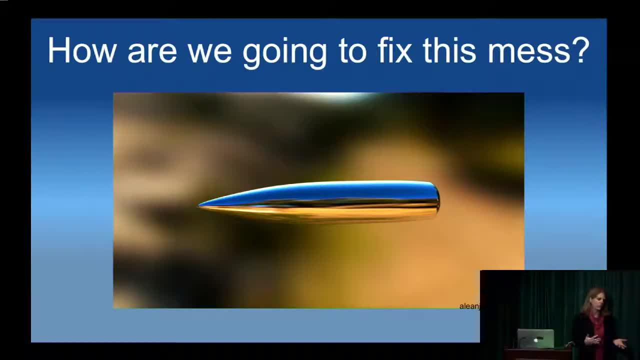 So many of the applications for plastics don't lend themselves to a material that will break down, So I personally would like to see us just use less single-use stuff than trying to make it out of something that will break down, whether in industrial composting or not. 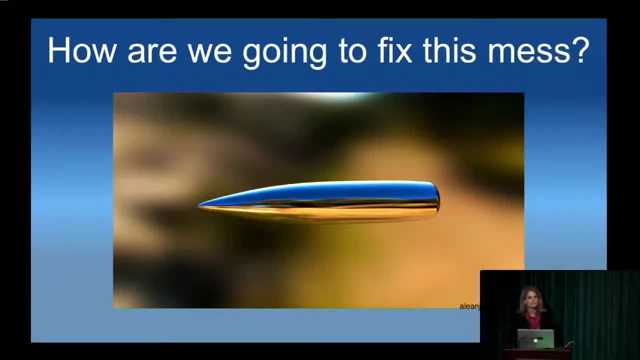 I had a similar question about biodegradable plastics, But I'm wondering, as you're talking with a biodegradable plastic, are there still actual plastic plastics, oil-based plastics, mixed in with the biodegradable? Do you know anything about that? 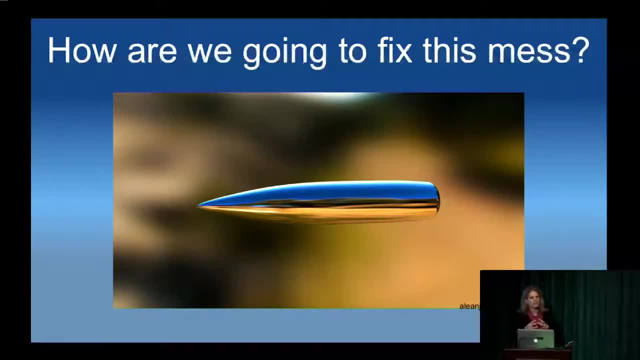 You mean in an individual item? are they mixed in? So if you had like a cornstarch bag, is it all cornstarch plastic, or are there oil-based plastics in there as well? Yeah, that's a good question. 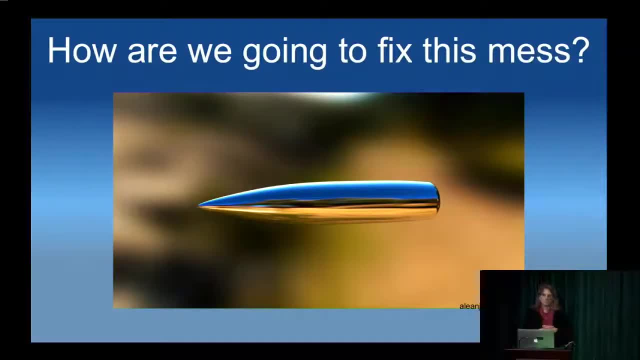 So this is where you know: consumer beware, Six-pack rings that hold your beverages right. So when I was a teenager, I knew that I had to cut out my six-pack rings so I didn't kill some marine animal. I knew nothing more than that's what I was supposed to do. 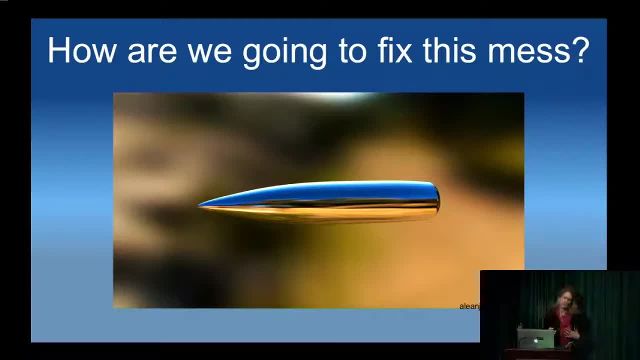 Well, those six-pack rings are now made of plastic that is called photodegradable. So it is a traditional plastic, but bound with starch molecules that allow it to fragment. So the idea is that if the six-pack ring gets lost in the ocean, it will fragment and it won't be an entanglement hazard. 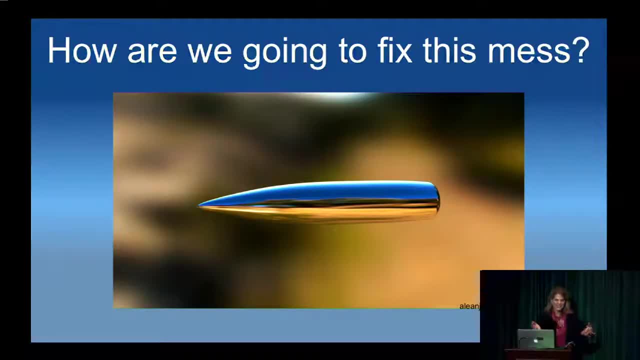 That's great, but now it's generating a tremendous amount of microplastics. So you're solving one problem but perhaps contributing to another. So I think it depends on the individual item. You really have to read what these things are made of. 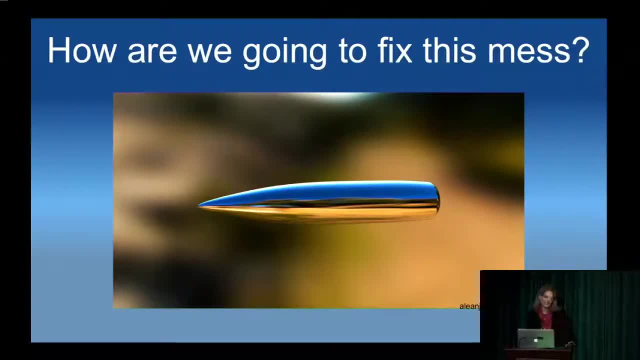 I myself have fallen for what I thought was compostable, and I accidentally bought something that was just made out of corn. So yeah, I think you just have to be careful. I was going to ask you a second question While I'm going over here, Kara. what about China, the big dog on the block with regard to sources? 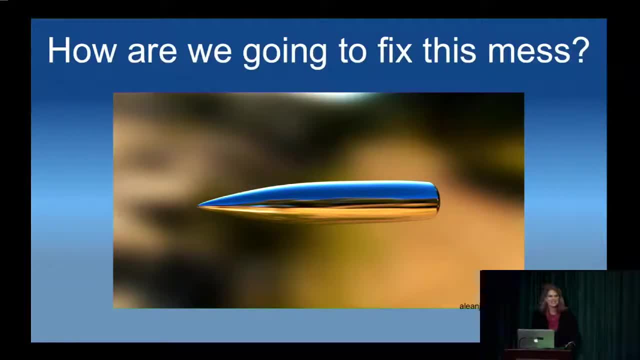 Yeah, that's a great question. So China is an interesting one, The Trash Free Seas Alliance, in following up on that study and when we put out that study, none of those numbers are right in the sense of— I mean, we think it's right to an order of magnitude. 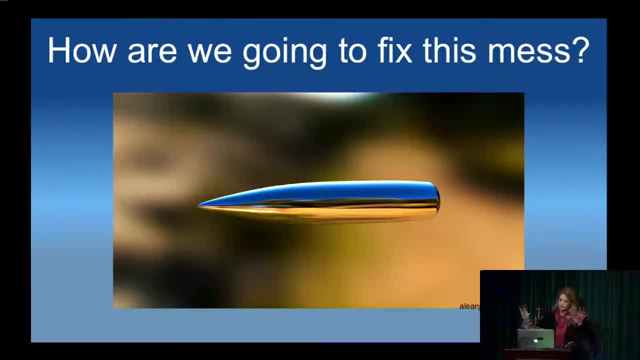 and we did enough sort of moving around with the numbers, challenging our assumptions, to make sure that we think the general kind of order is plus or minus right. So we don't think the US has got to leap up to number one. But you really need to go to these places and measure what's on the ground. 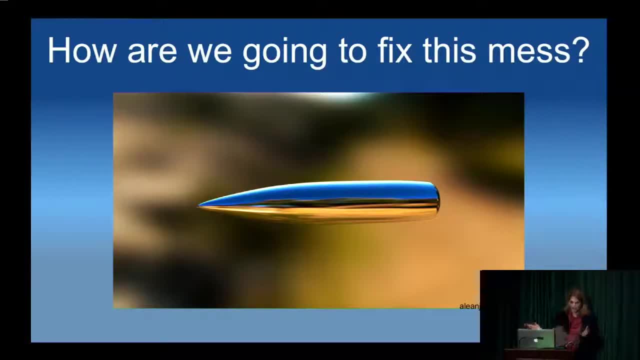 Measure. Nobody really is measuring what's flowing out of a river. I mean, very few data of that flux exist, But the people who are going and working on waste management are going to Indonesia and Vietnam and Thailand. I don't know of anybody going into China. 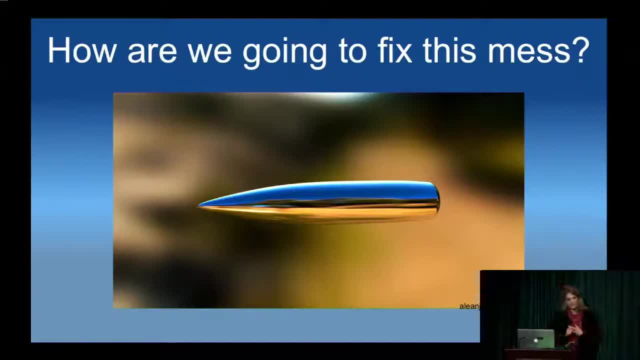 I think it's a tough nut to crack, But China also used to be, until very recently, the country that took in all of our waste, our single stream, our mixed plastics, our mixed paper, because they had a workforce that could pick through it. 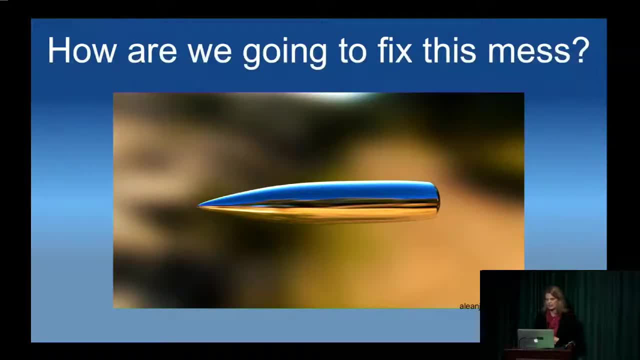 Excuse me, That could pick through it and make a living, And they have since put up what's called the green fence national sword as the policy. So they are now turning away recycling containers that are above a really minimal amount of contamination, which basically doesn't exist. 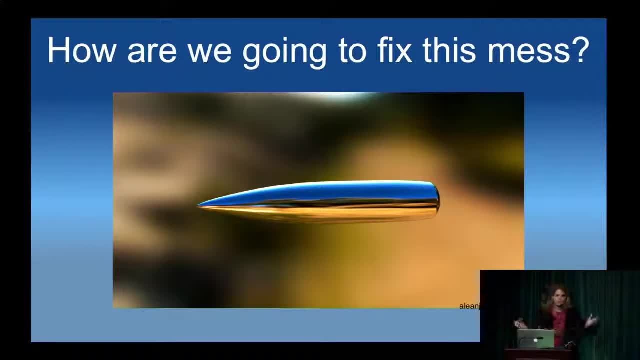 So that's really challenged our recycling in this country, because we're all used to just dumping it all in one big bin and then figuring that somebody somewhere somehow is sorting it And that somebody somewhere somehow is no longer China. So that's yeah. 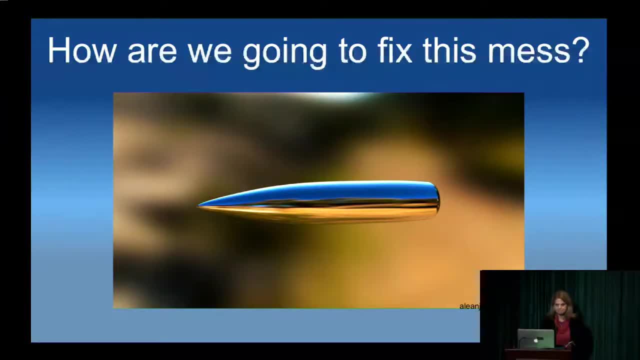 That's a good question. I had a question about the plastic fibers. Do they come strictly from things like netting or do they come from other types of plastics? So that's a good question And we don't really know. I mean, we can look at the composition of the fibers. 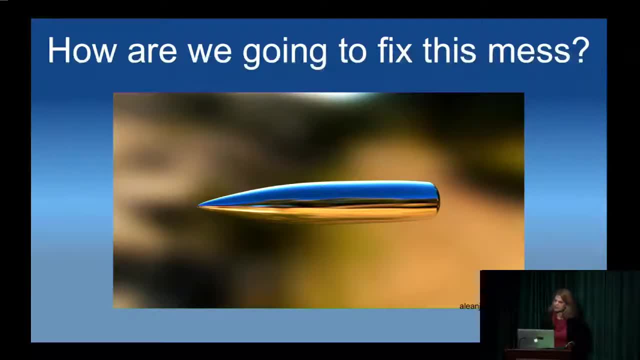 And so we can say, yes, they're polyester or nylon or whatever the material is. I think a lot of people like to talk about clothes and washing machines, because there has been a study that sort of shows that fibers shed off clothing in the washing machine. They can come out. But really I mean look around us with carpets and upholstery and microfiber cloths that you use to clean with your furniture, your car seats. I mean there's fibers everywhere, So it's not just your synthetic clothing. 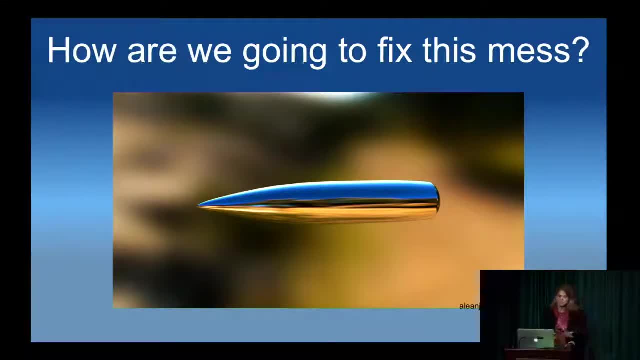 And a lot of the fibers actually are natural materials. They'll be cellulose-based or cotton or wool, So it's really important to know what type of material the fiber is that's contaminating the fish or the shellfish or whatever, But it may be more important. 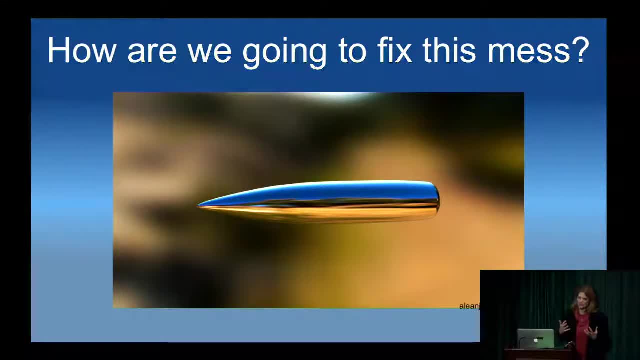 It may be more important that it's a fiber. This is where some of this, you know what is really the impact. Does it matter that it's a long, skinny thing that might be able to cross into the bloodstream, Or does it matter that it's a long, skinny thing that's made of plastic versus cotton? 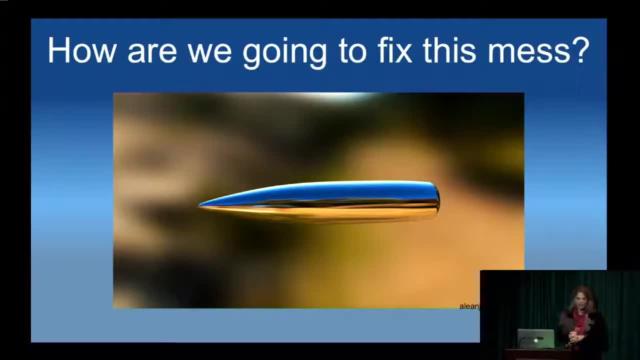 We don't have the answers to those questions yet. I don't know what the solution is to fibers. I like my fleece. I live in Maine. We have a question here. First of all, thank you very much. It's been very interesting, very informative. 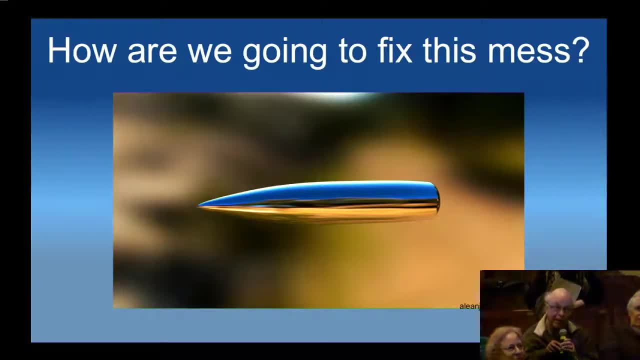 You have mentioned a couple times corn and biodegradable, that it's not biodegradable or something. What is that? It depends on the material. So most traditional plastics are made from fossil fuel sources, so oil or natural gas. You can also make those from plant-based sources like ethanol, sugarcane. 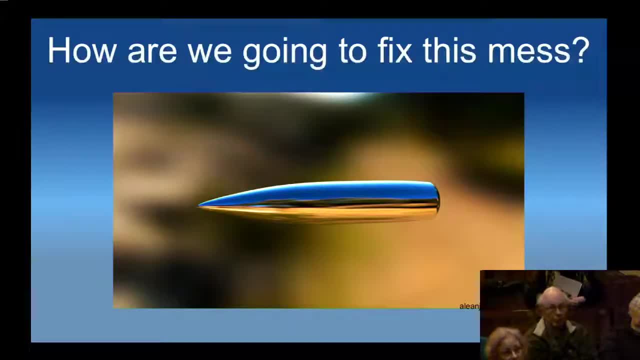 The end product is the same. It's the same molecule. Corn-based traditional plastics are no more biodegradable than oil-based traditional plastics. There is another category of polymer called PLA, polylactic acid, also made from corn or maybe- I'm not entirely sure of the constituents- but plant-based that is biodegradable in that. 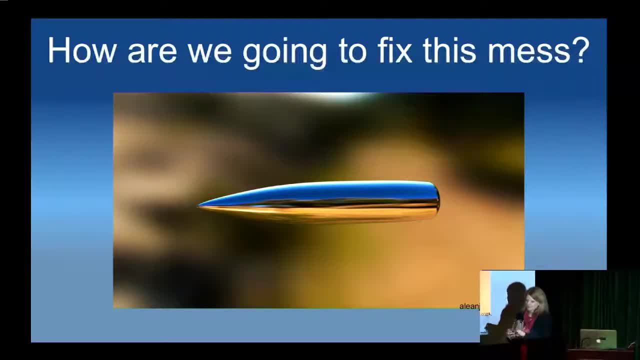 particular environmental condition of an industrial composting facility. So thank you for asking that and clarifying, because it is confusing. I enjoyed your talk. I enjoyed your talk very much. I have a comment and a question. The question has to do with the health risks associated with eating seafood, be they shellfish or regular fish. 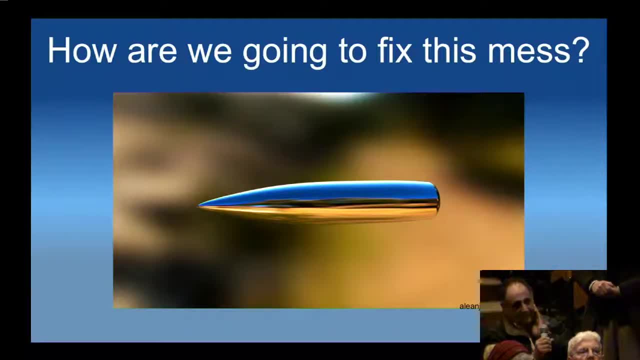 And then two. if you're only looking at floating debris, you're missing part of the problem. Given the density differences of these materials are denser than seawater in some cases, So maybe some of it is sitting on the bottom. No, absolutely. 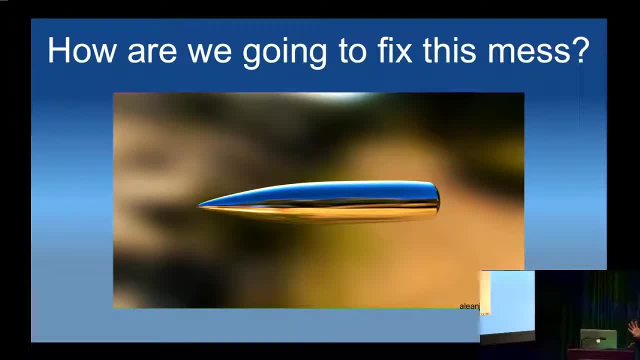 And in the beginning of the talk I tried to make clear that, although I was going to focus on stuff floating, we know there's material at the seafloor. The challenge is that we don't have enough information on the seafloor to say 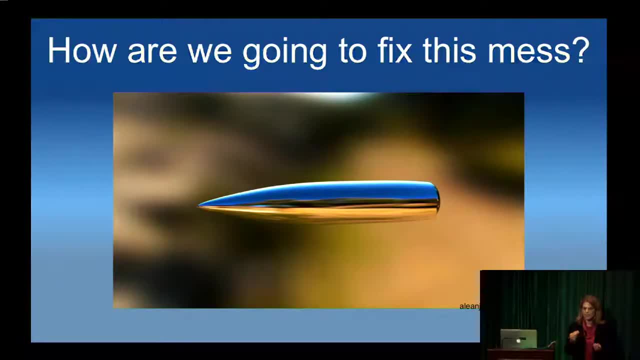 is there more sitting as big stuff on the seafloor, or is it all microplastics and sea ice, or is it all sitting on beaches? And it's interesting. It's interesting in the scientific community in this field, because there's definitely the it's all sitting on the seafloor camp. 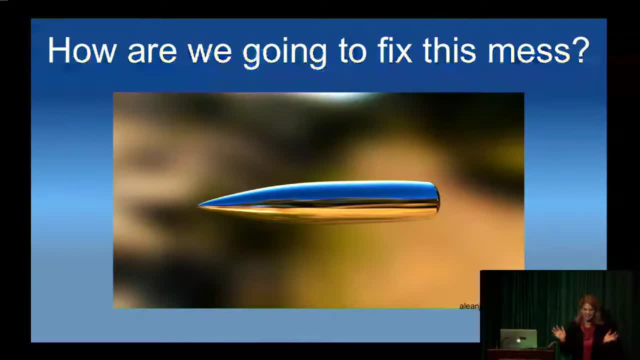 and there is the. it's all sitting on the coastline camp And I'm sort of like I don't really know yet. So that's absolutely right. I mean, we know we're missing it. In fact, we're only measuring a very small size range floating. 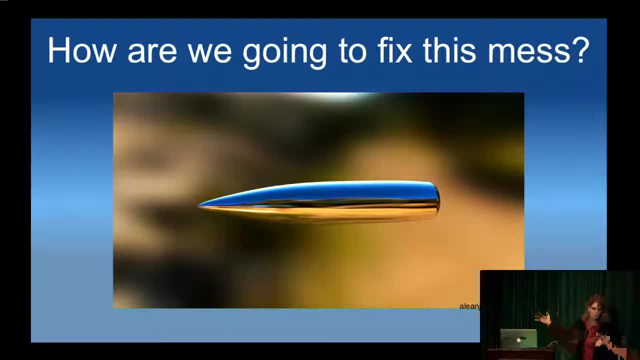 So that doesn't even account for the big stuff that's floating, like I showed you, from the Japanese tsunami. So absolutely Human health. We know that we're ingesting plastics when we eat seafood. I still eat seafood, I'm not concerned about it. 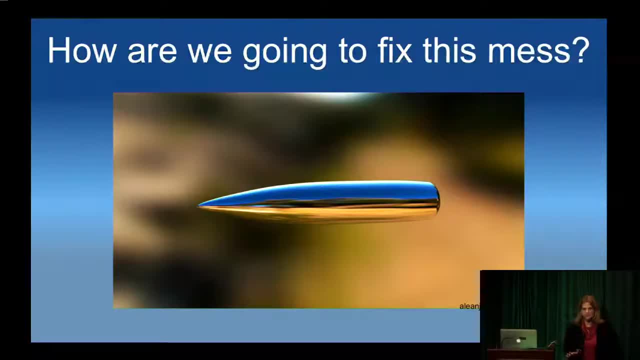 I'm more concerned about my exposure to plastics and all my other activities because, relative to what I'm exposed to through my seafood, I'm getting much more exposure on my skin and potentially inhaling it. That doesn't mean it's never going to be a problem. 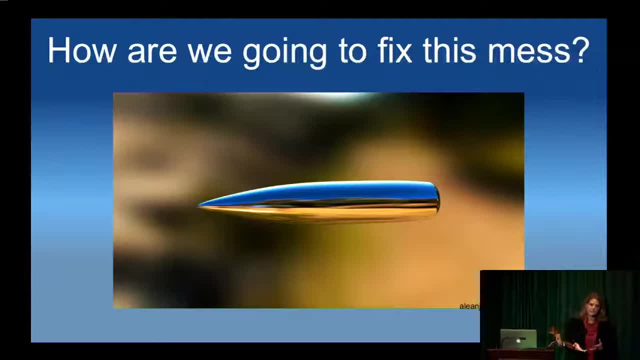 And it doesn't mean it's not a problem for the animals that are eating those things. But that's why it's such an active area of research And that's why it's so hard, because plastics it's not a single material. 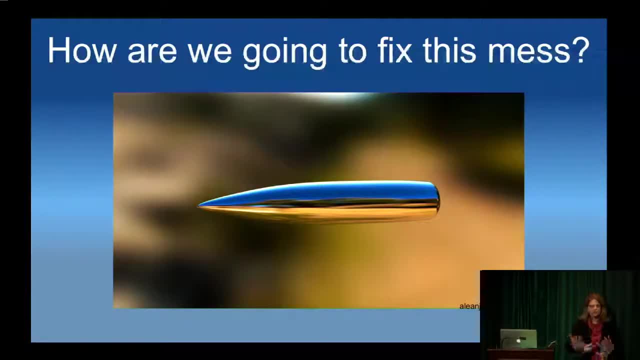 It's a variety of polymers, Some of them float, Some of them sink. There's a variety of additives. They behave differently in the environment. They're different shapes and sizes. It's not like you're just studying one thing. You're studying this really heterogeneous pollutant. 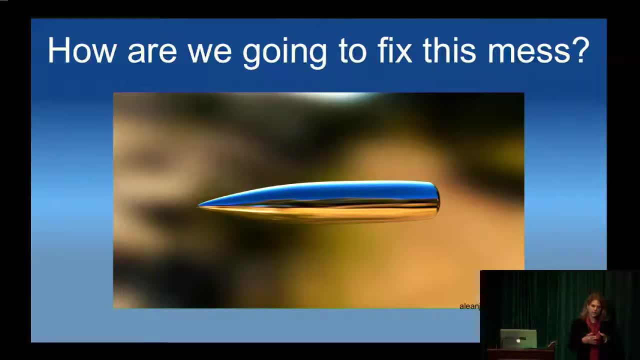 And so you have to be really careful about what you learn in these laboratory experiments and then what that tells you about the real world, whether human or marine animal. If we accept that the problem is with us for the future, because all we can do is reuse, reduce and so forth and manage what we're doing. 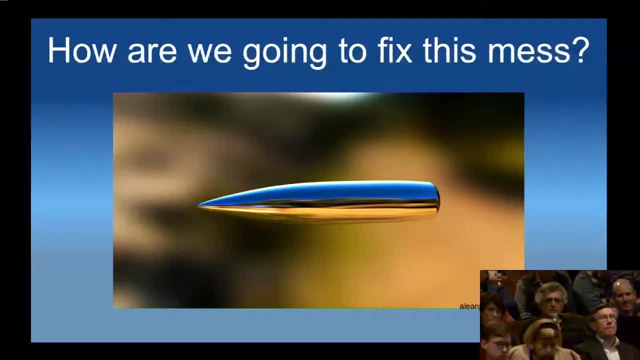 we're not fixing the mess at all. We are making it less, We're growing it more slowly. So what does the world look like in 100 years' time? That's a great question. Well, you know, I mean, we've already dubbed this era the Anthropocene. 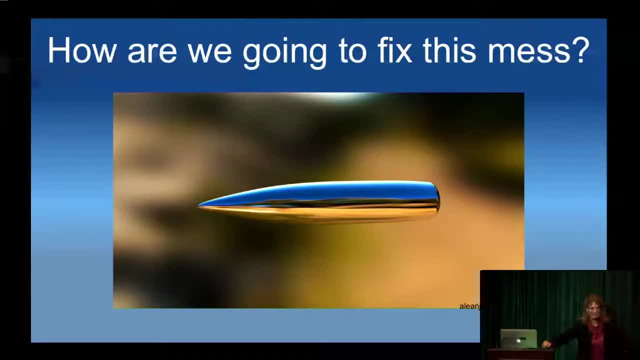 because we're going to see these layers of plastic in landfills and beach sediments. You're right. I mean, even if we reduce the way that we use these materials, that plastics production curve is probably not going to slow down. So I don't know. 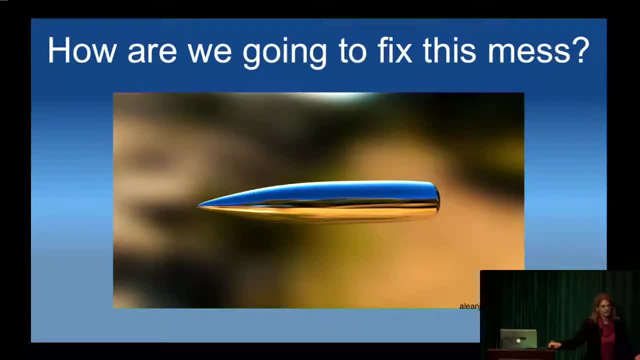 I mean, I sort of feel like plastics aren't going away and we need to think about what we do with them when we're done with them, And the producer needs to be involved with that, whether it's the person that makes the plastic or the person that makes the product. 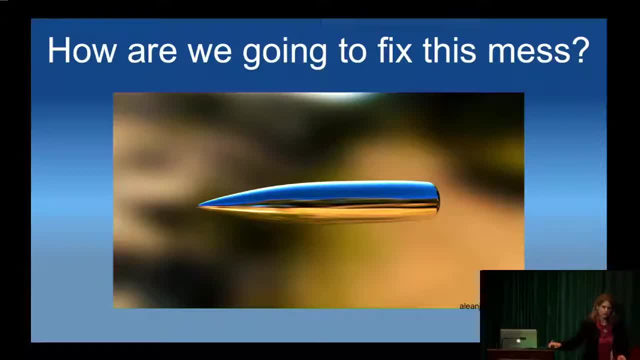 And we need to be good consumers in how we make our decisions and then how we treat our waste. I mean, the world will still have plenty of plastic in 100 years. I just hope that you know we're not unable to eat seafood. 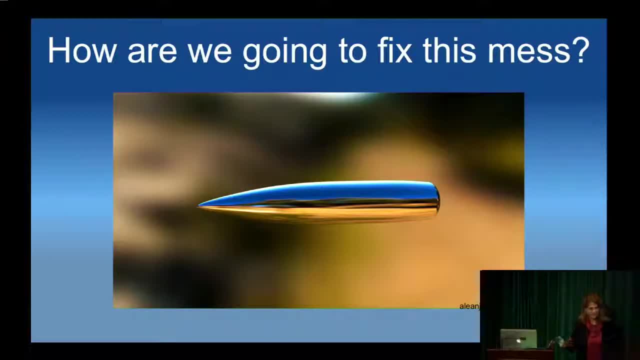 Because we've now determined that it's- you know it's killing us, And thank you for your wonderful talk. In a community like Woods Hole that is both affluent and be close to the coastline, I wonder if it's somewhat easier to convince people to have single-use products. 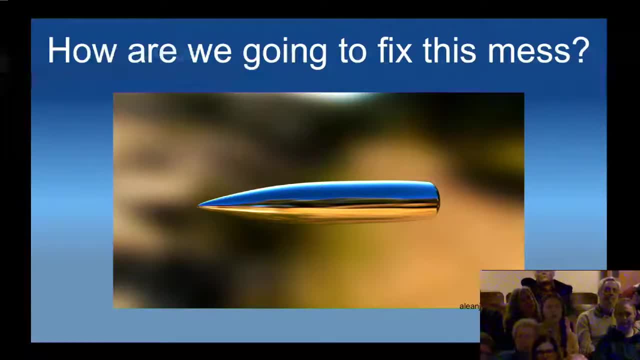 whereas in places that are maybe not as close to the coastline or have a lower socioeconomic status. I wonder what ways we could make reducing our plastics both feasible for those communities where the ease is very important and the inexpensivity is very important, as well as not maybe at the forefront of their thoughts. 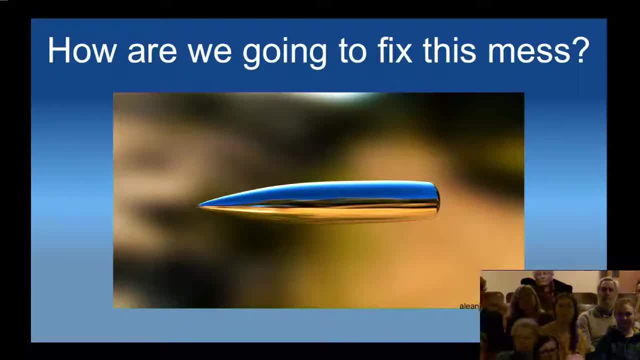 Thanks for that question. I mean it's interesting because we think about: okay, so Falmouth is a relatively affluent community in our region, so how do we reach sort of other communities close to us? But then we even think about places, communities in Africa. 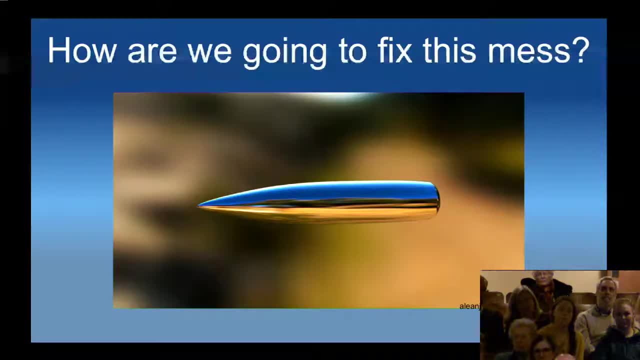 where there is no clean water and they literally buy pouches of water to survive and so you can't remove, you can't take those away And that clearly is like we need to work on clean water for those communities. So that's like a bigger problem that the plastic is a symptom of. 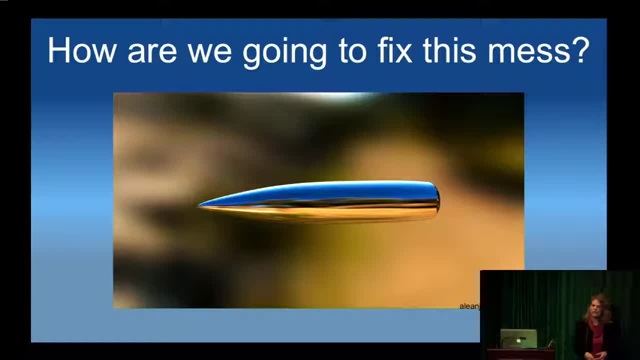 More locally. you know, I don't know, I'd have to think about that. I think about plastic bag bans and some of the arguments that you know you're disadvantaging people who can't buy reusables and the way that you overcome that is when you institute that. 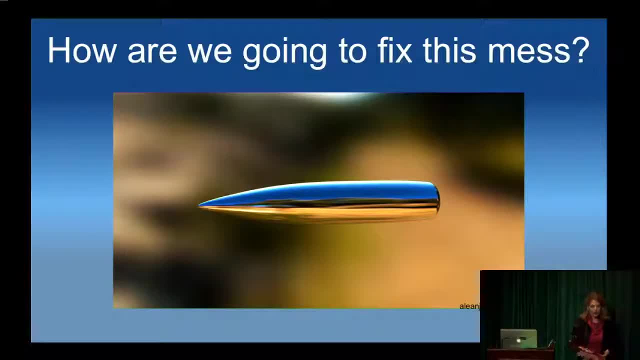 The stores maybe are subsidized to do it, but give away some reusables. So I don't know exactly how to do that. I'd have to think more about it. But we are intelligent, thoughtful, entrepreneurial people and we can figure that out. 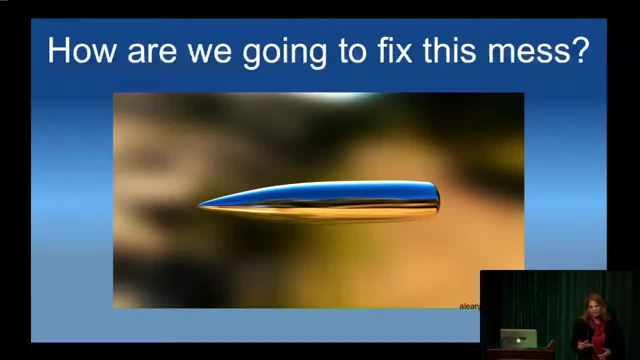 Like that. one seems like we can do that And we can do Africa water, but that's a much bigger beast to tackle. But it's true, We can't say you can't have your pouches of water. Thank you very much. 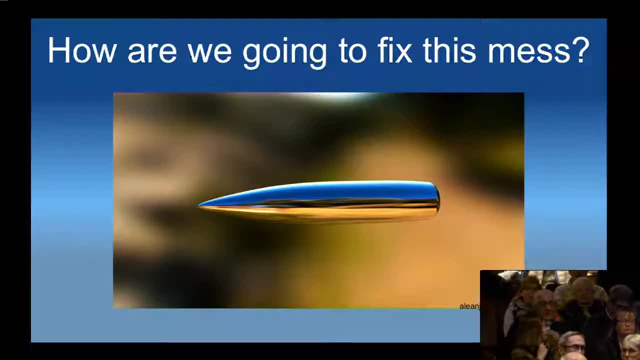 It was a wonderful presentation. I think we are all here in this audience and all of the population are the silver bullet to solve this problem. However, I don't think plastics are the only problem. There have been several studies readily available where plastics only represent 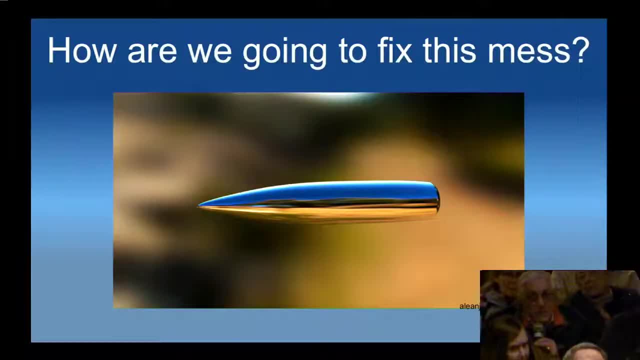 10% of the worldwide waste that is going somewhere, be it in a landfill or be it in the ocean. I think an interesting aspect of this and future study would be to look at within 10 to 15 miles of a coastline. 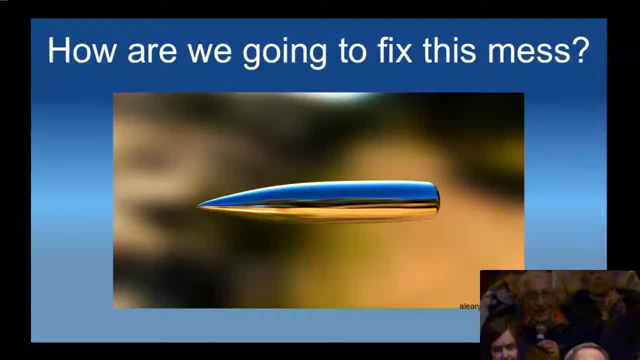 and see what the bottom of the ocean looks like and see what materials which are heavier than plastic materials are actually on the bottom, Because 90%- it is a fairly large number, That's true- Most of that is organics. So when you think about waste actually, 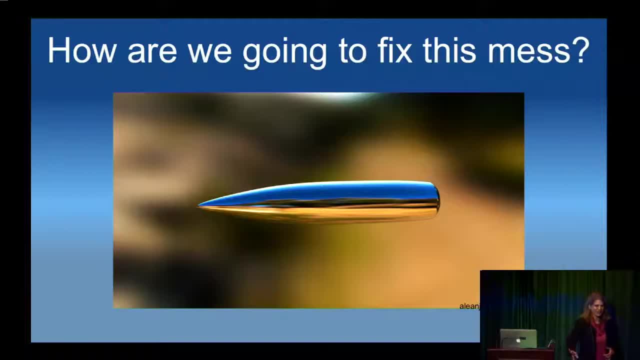 one of the best things we can do is divert organics to composting, and that will severely reduce our waste stream. There have been- I mean, it's not that there's- no information about what's going on, what's on the seafloor, and you're right. 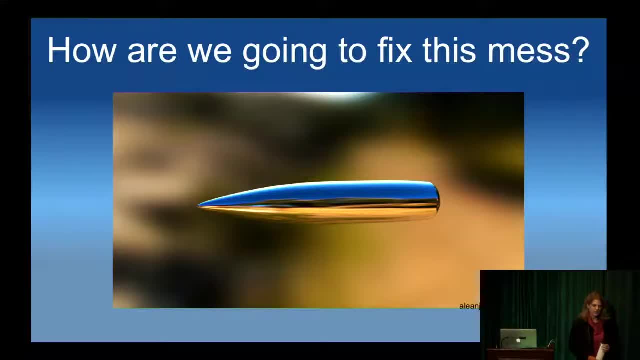 I mean, you'll see the tire or the kitchen sink and things like that, At least by count. when we look at what's on the beach and in many of the seafloor studies, most of it, at least in part, is composed of plastic. 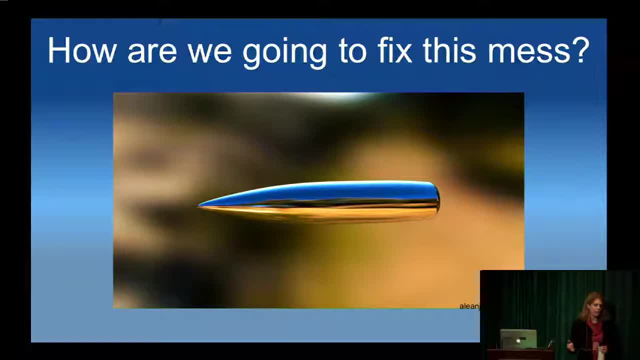 But I take your point. I mean surely there are centuries of glass, whatever sitting on the seafloor, The thing with glass and metal, at least, as some of the sort of major materials that we use and dispose of, they do sink and they don't really move. 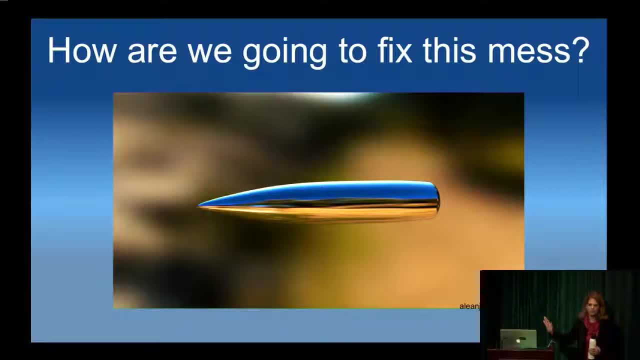 So the thing with plastic- and when we started in this working group I mentioned, we took marine debris as all materials and we pretty quickly narrowed in on plastics, not because they're evil and we hate them and people love to hate them, but because there's actually really good reasons for that. 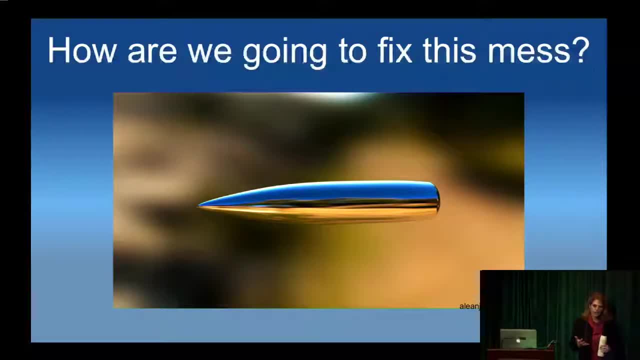 Not only are they the most abundant things floating, but they transform over time. So these chemicals I talked about can come and go. The additives can leach out, Other things can sorb. They break down into smaller and smaller pieces. We don't think they ever biodegrade in the environment. 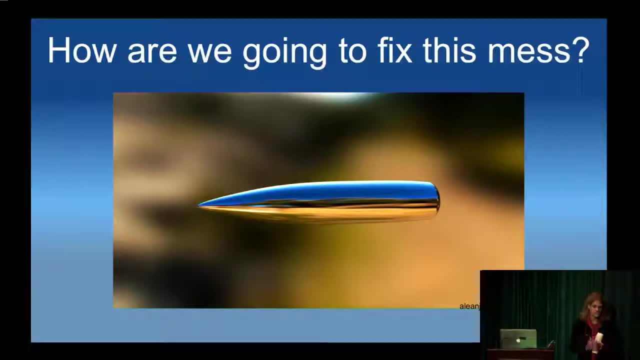 I mean it's hard to say that positively or that they never will, But they move around, They transform, They interact with wildlife the same way, Whereas a glass bottle or unexploded ordnance or the kitchen sink is kind of sitting there. 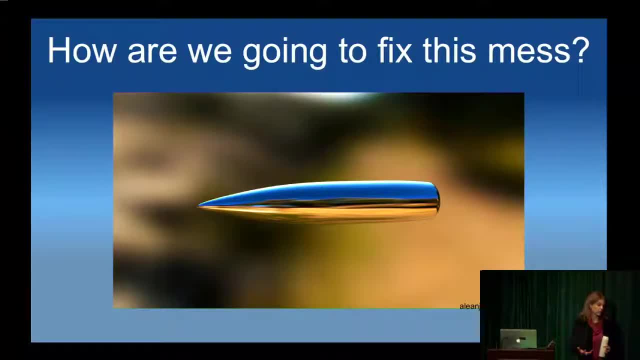 And unless you have some kind of major disruptive event, it's probably just sitting there and affecting the immediate area. So I take your point. I mean, plastics are not. yeah, it's not 90% of our waste stream, but it is an increasing number. 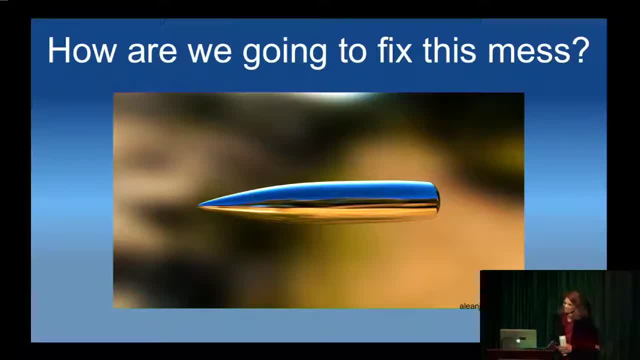 So I would like to thank Kara for this great talk and also for this discussion That we just had, And also to each one of you for being here today, So please thank you to everyone. If you would like your own trash and splash sticker. 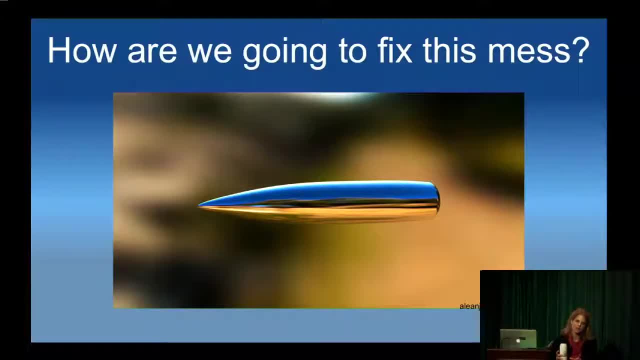 they are on the table in the back, as well as some postcards that are made with artwork from the local K-12 community. We had a call for ocean art and we created some messaging postcards with those, So I welcome you to take those and share them.